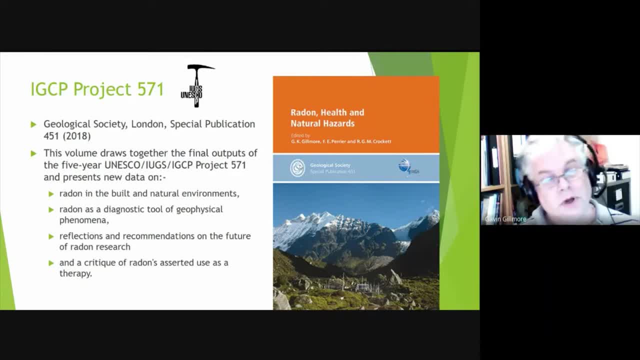 because indeed it can be a very useful tool to think about radon research in the future, where that might be going, And also there has been some interest in radon's use as a therapy, But that's something which I won't be commenting on, particularly in this. 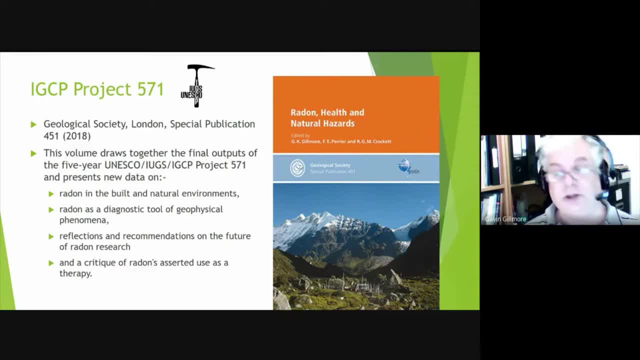 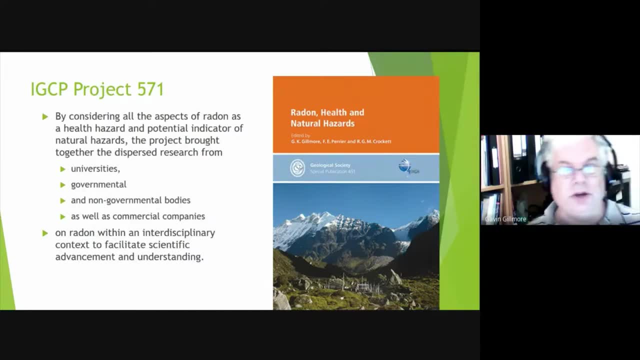 session, But nevertheless it's not something I would actually recommend to you. So the project is looking at health hazards, potential indicators of natural hazards, and drew together research from a very disparate veryan亲 work. So this is a very significant study published in Connecticut. 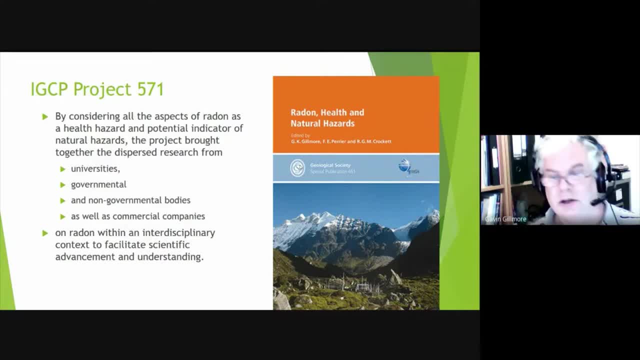 where they study the risk of emissions of radon and the potential use of it And at the end of this study they willing to develop a model to try to date back to the first body of individuals, So people working in universities, government bodies, 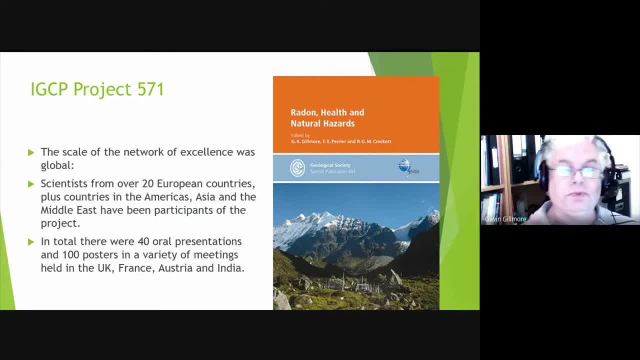 non-governmental bodies, commercial companies, all working together in this interdisciplinary. European countries, plus countries in the Americas, Asia, Middle East, have all participated in the project And there was something like 40 oral presentations. So there was a whole series of meetings in UK, France, Austria and India and 100 posters as well over the 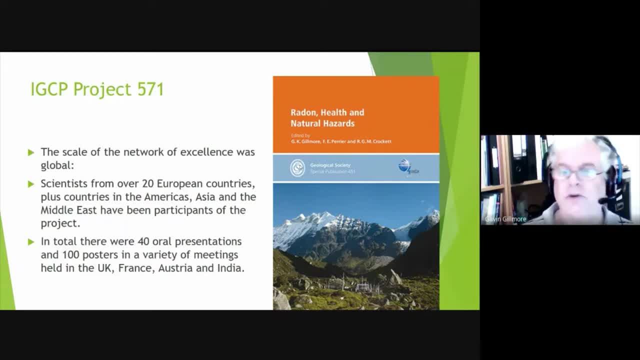 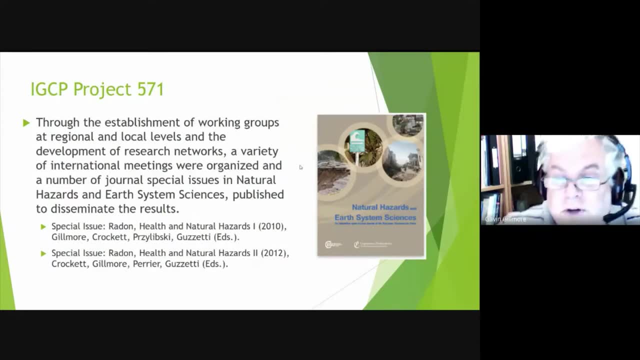 five year period. So an awful lot of material was produced by the project. So some of that material was published in the Geological Society final publication that I've just shown you pictures of. But also we had two special publications in the Natural Hazards and Earth System Sciences. 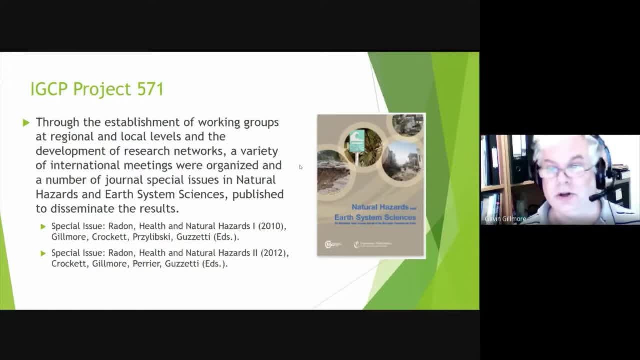 journal, which, incidentally, is a free, open access journal for those who want to look at papers. So we produced working groups that worked at regional and local levels, whole series of meetings, as I said before, on which used the special issue in 2020, which was 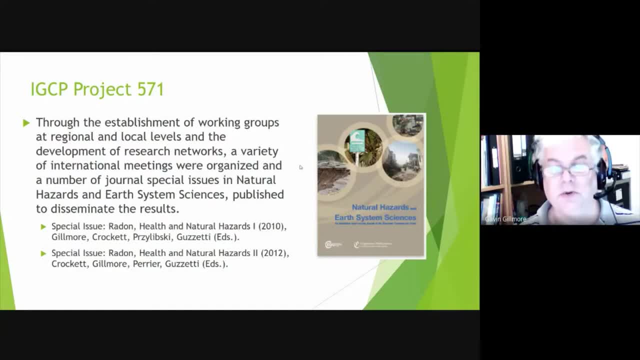 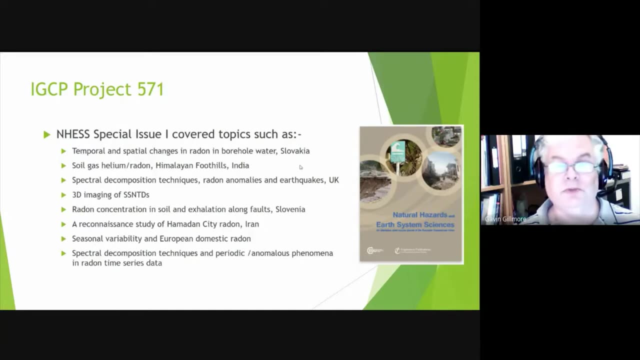 published in 2010, and then a further special issue in 2012.. Okay, so I'll just run through some of the topics simply to show you the breadth of material that we looked at. So in special issue one, things like temporal and spatial changes in radon in borehole water. 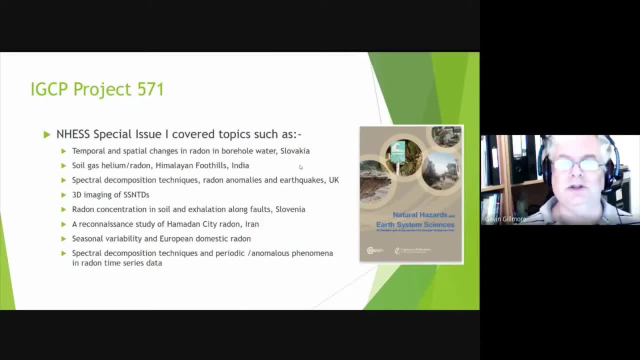 in Slovakia. Now radon is actually easily dissolved in water, So it actually can be ingested in radon, Okay, In radon enriched waters. So we looked also at soil gas, radon and helium in the Himalayas, looking at radon anomalies and earthquakes. 3D imaging of solid state nuclear track detectors. 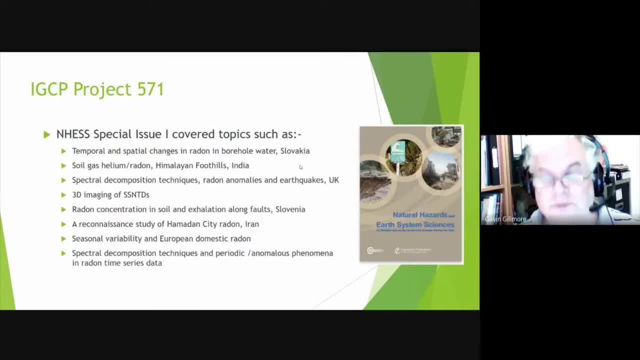 which is what SNTD stands for. So that was about quantification of radon: Looking at how radon actually is exhaled along faults in Slovenia, Looking at cities such as Hamadan in Iran- and I'll talk a little bit about that later. 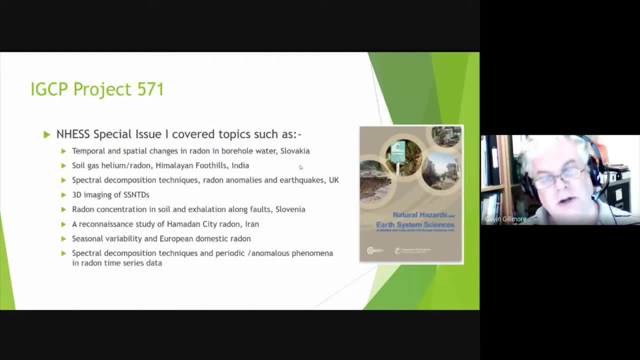 on Looking at seasonal variability and radon across Europe, basically in domestic properties, And then also looking at periodic and anomalous phenomena in radon time series data And then issue two things like looking at ornamental stones, So granites, for example. 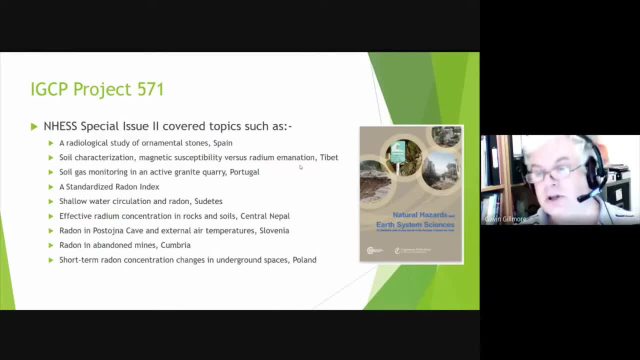 are quite often used as ornamental stones, but they can be enriched in uranium-238, which is the precursor for radium-226 and radon-222.. So we also then looked at magnetic susceptibility and radon and radium emanation. We looked 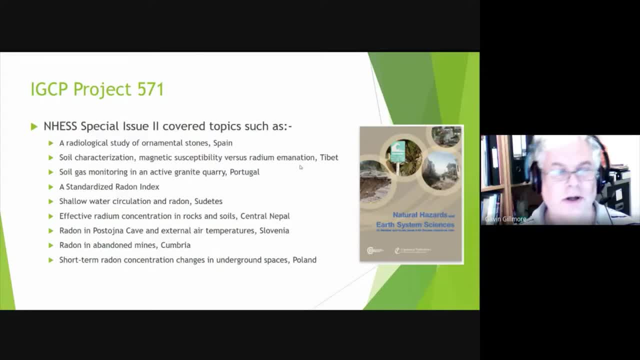 at a granite quarry, looked at soil gas monitoring, looked at water circulation in the shallow waters And radon concentration in shallow versus deep water. Looked at radium concentration in rocks and soils in Nepal. Then looked at caves and the comparison between internal and external air temperatures and 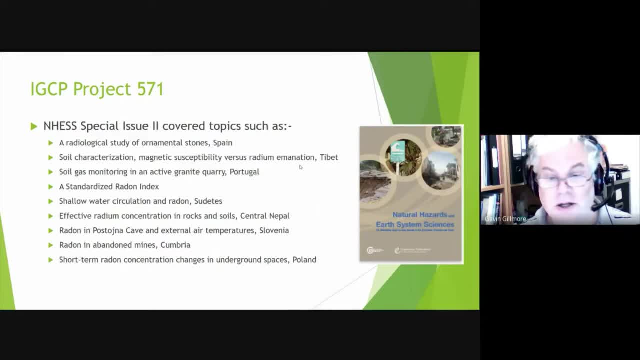 radon And then abandoned mines in Cumbria in the UK, So these were copper mines- And then looking at underground spaces in Poland and looking at short-term radon concentration changes. So a whole variety of different topics were looked at during the project. 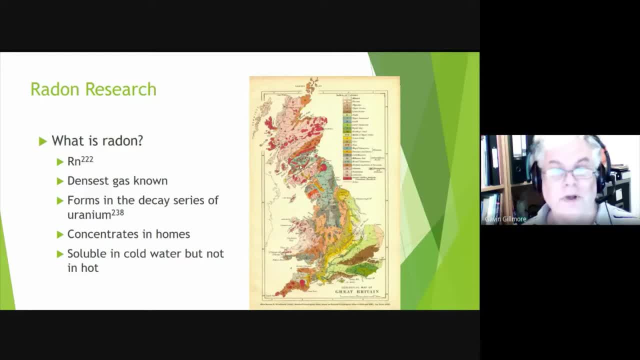 And lots of different countries contributing. So what is radon? Okay, so many of you will know we're talking about radon-222.. So that's a radioactive gas. It's the densest gas known, So we'll tend to concentrate in basements and ground floor of buildings. 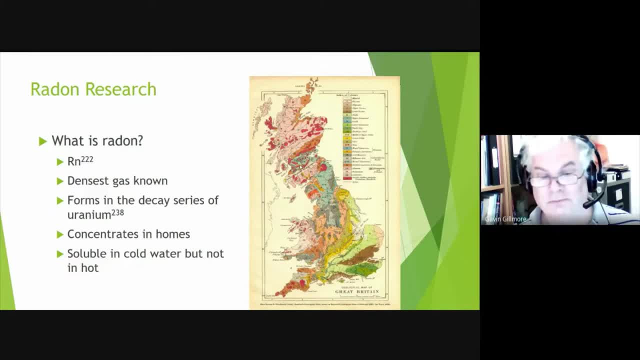 It forms in the uranium-238 decay series Concentrates in homes. It's soluble in cold water but not in hot water. So of course if you heat water or you make the water turbulent, then you can actually release gas from the water, assuming there's any gas there in the first place, of course. 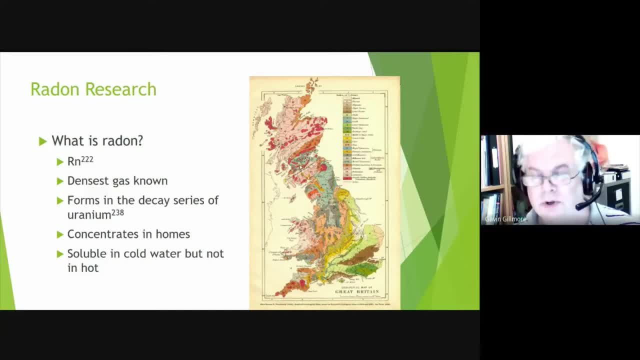 And then you can see this whole geological map of Britain, And one of the interesting things about the UK is that geology is incredibly varied. Okay, so it's one of the most complex geologies per square kilometre of any country. So that means actually, in theory, radon can vary quite considerably. 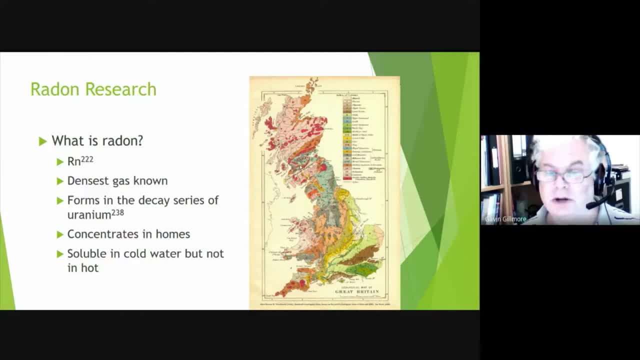 And I said earlier that radon can be associated with granite, So the red spots that you see here, particularly in the southwest England, you can see red blobs And this represents granites, And these particular granites have high radium, uranium and therefore radon generation capabilities. 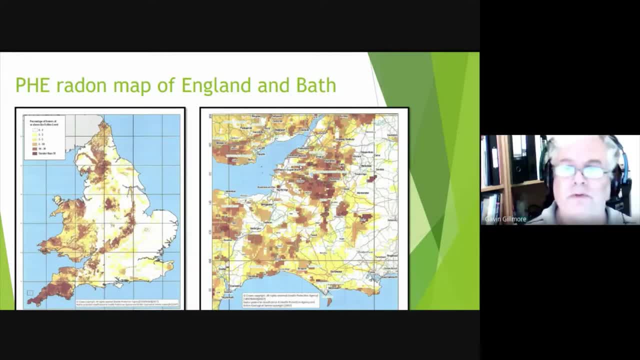 So Public Health England have produced a radon map of England and the UK. Bear in mind This map is based on measurements made and not everywhere has been measured, So you have to treat the map with a certain degree of wisdom. So the map is not a sort of authoritative guide. 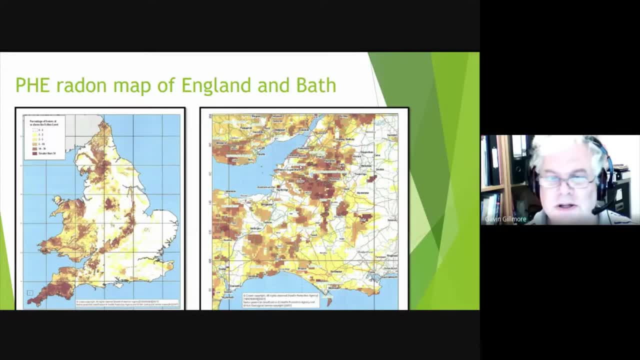 It's not saying you will find this amount of radon here. It's basically saying it's a predictive map. It's saying this is what's likely to occur at this place, based on the data on which the map is based. if you see what I mean. 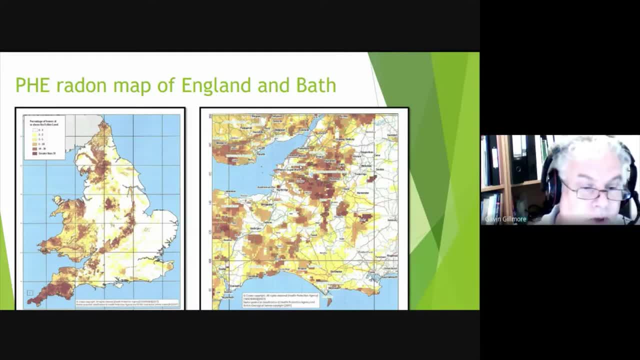 But you can quite clearly see that the map is based on the data that you see here. You can clearly see on the left-hand figure high concentrations of radon with homes above the action level: 10 to 30 or greater than 30% of homes above the action level. 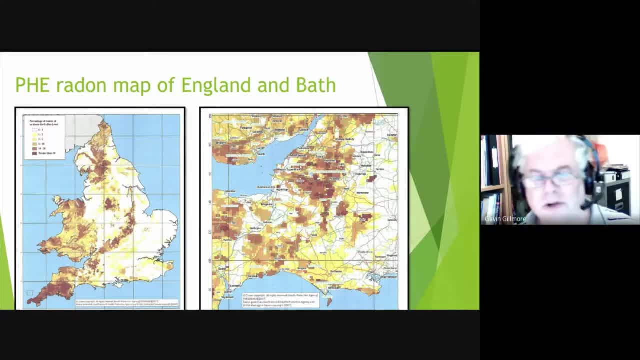 So the action level in the UK is around 200 becquerels per cubic meter of radon gas, And becquerel is one disintegration per second. I'll say a little bit more about the action And then if you look at the map on the right, you can quite clearly see, if we look more. 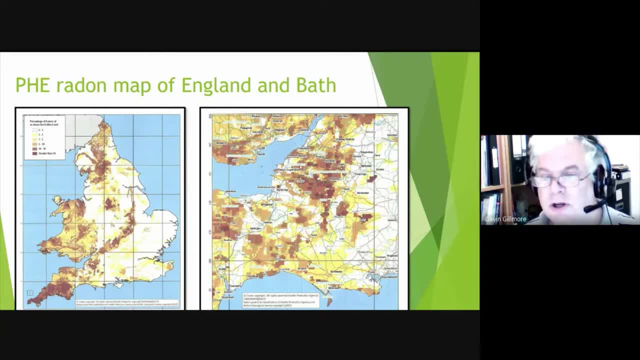 closer to home you can see the Bath and the surrounding countryside, particularly to the west, has a significant radon problem. So you can see concentrations in the Radstock, the Keensham and around some parts of Bath as well. So Bath and northeast Somerset has a radon issue. 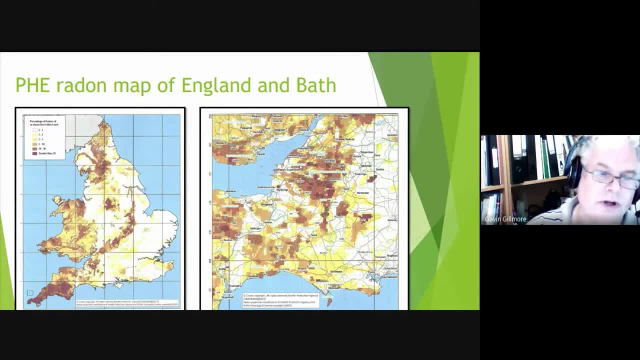 The other thing I was going to point out is that you can see Wales- I'm not going to go into that, I'm not going to go into that- But Wales has raised radon And you can also quite clearly see if you look at the right-hand part of the left-hand. 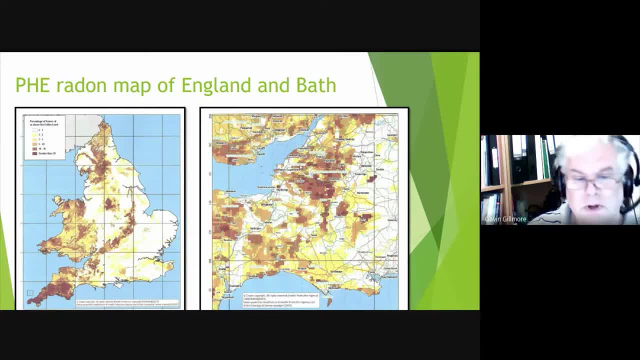 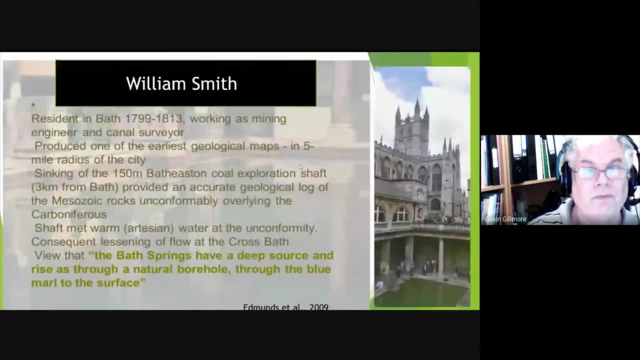 image you can see southeast England. there's a sort of a circle or a sort of squashed ellipse, I suppose, of higher radon And that's associated with the geology which is an anticlinal structure, the Wealdon anticline. 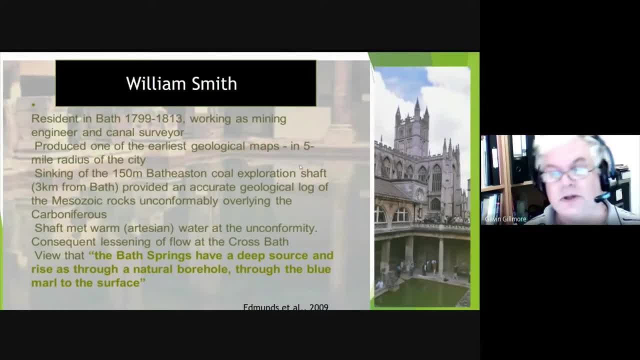 So what has radon got to do with Bath? Well, okay, Yeah, There's a lot of examples in Bath and the surrounding area. Bath has been linked to radon historically. So William Smith, often known as the father of English geology, spent a lot of his time. 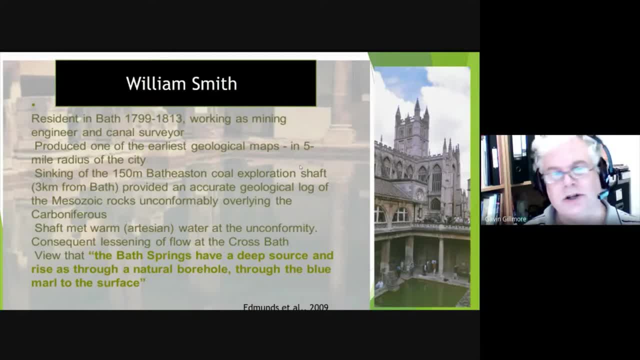 in Bath. He worked as a mining engineer and as a canal engineer And he produced one of the earliest geological maps of a five-mile radius of the city And he sunk a coal exploration shaft. Yeah, In Bath, Eastern, three kilometers from Bath, produced a very accurate geological log of. 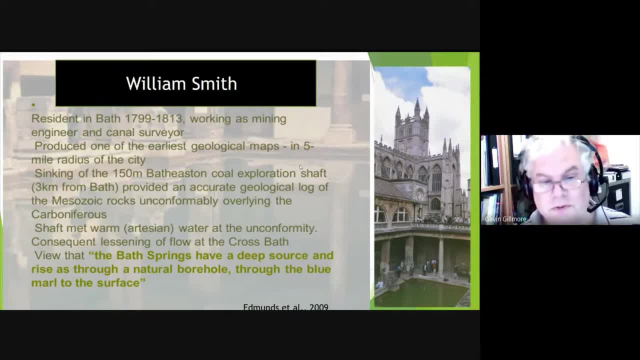 the rocks And he met artesian water that was warm in that well And also he, by digging the well, he affected the flow of some of the Bath Springs. So the spring at Cross Bath, for example, was affected And he concluded that the Bath Springs have a deep source and rise to a natural borehole. 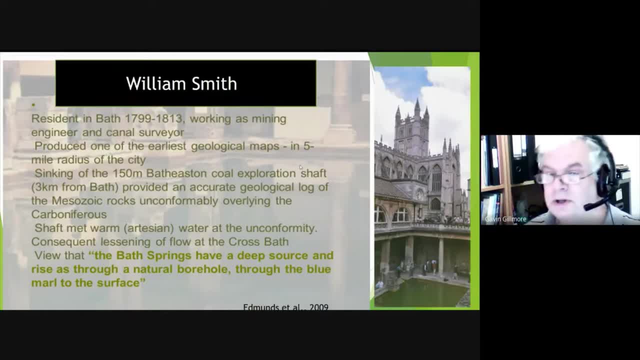 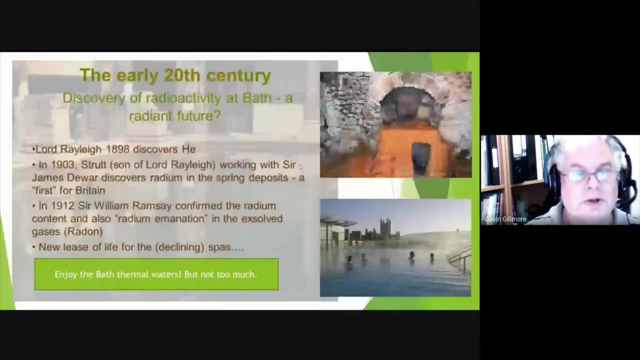 through the What he called the blue mile to the surface. So here's a picture on the right of Bath Abbey and the Roman baths, And this is very interesting because Bath Abbey is now partially heated by geothermal waters from the springs. But it's particularly interesting because of the link with radon and radium from this. 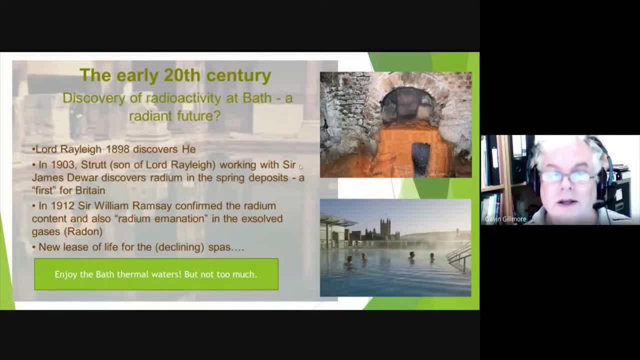 talk perspective. So Lord Raleigh, 1898, discovers helium. 1903, the son of Lord Raleigh, 1903. Lord Raleigh, working with James Dewar, discovers radium in spring deposits, a first for Britain. And 1912, Sir William Ramsay confirmed radium content and also what he called radium emanation. 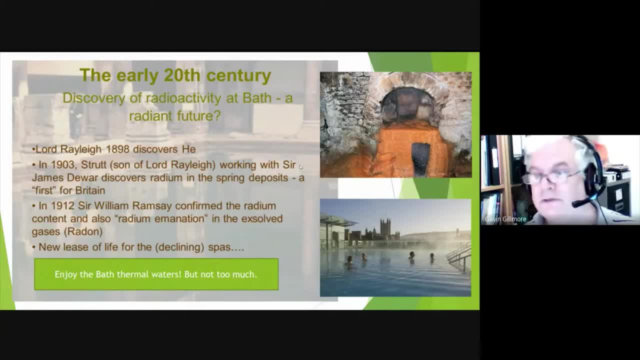 which was then later known as radon, And these were identified in the springs in Bath. So, as a fact, radium and radon were first identified in the UK, in Bath, And they predicted a new lease of life for the springs, which at the time were declining. 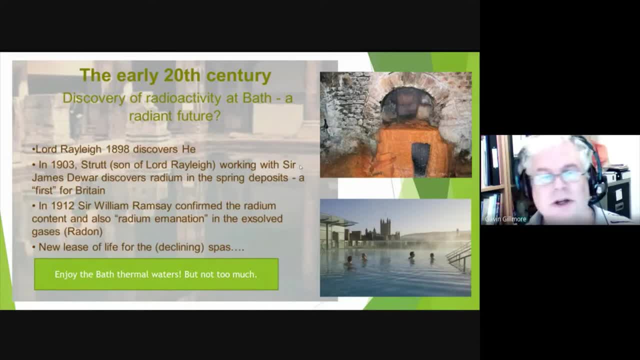 because there was a belief at the time that the radioactivity in the water was going to be good for you. I won't say too much about that at this stage, but I will come back to that. And so they said: yeah, there's a new lease of life for these declining spars. 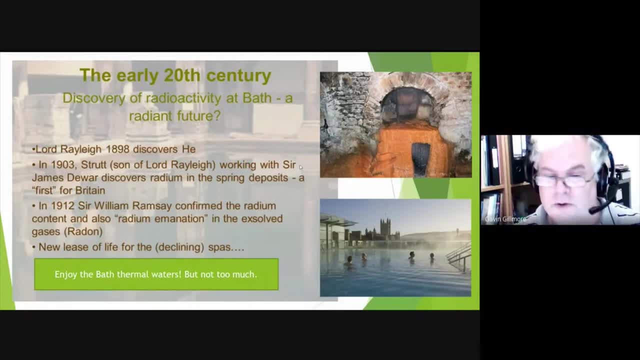 You can go and get yourself irradiated in the Bath Springs. So if you see 1940s brochure for Bath Spa, it talks about the life giving emanation of the springs. Bottom right you can see a recent development, a relatively recent development, back in 2012,. 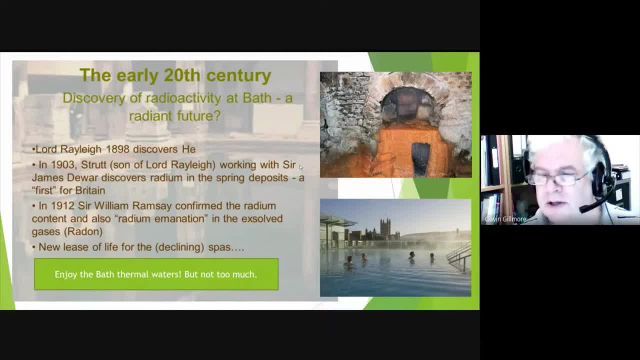 I think this was finished. This is ThermiSpar, so a luxury hot thermal spa on top of a hotel overlooking Bath. So notice, it's in the open air, So of course, any radon in the water is being dissipated quite nicely. So I said that radon, Radon 222, comes from the decay of uranium 238 in rocks and soils And this is the decay chain, So you can see uranium 238, and it goes through both alpha and beta decay through to radium. 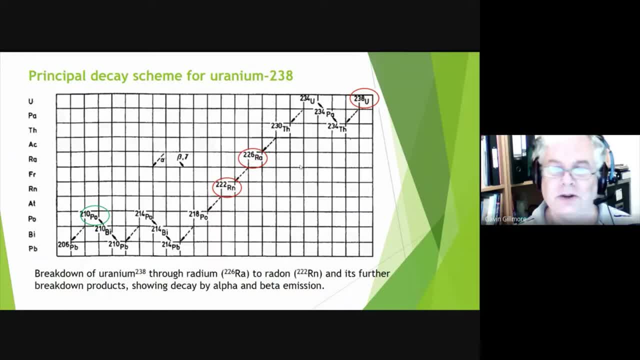 226, which then goes from alpha decay through to radon 222. So radon 222 is a gas You can breathe that gas in. That gas will deliver then Polonium 218, lead 214,, bismuth 214, et cetera into the body. 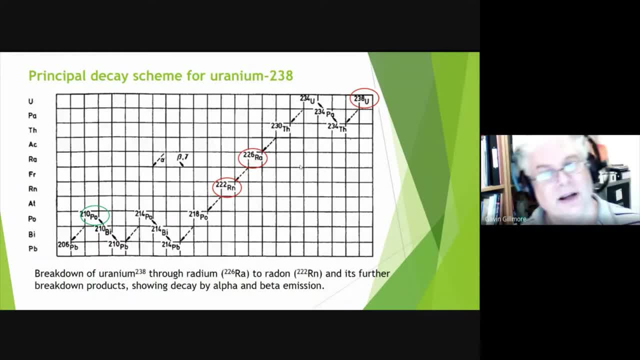 So this is why we're sort of a little bit concerned about radon and the concentrations of radon that people may or may not be breathing. in Notice I've also green circled polonium 210, which occurs in that decay chain. Hopefully it'll become obvious why I've done that as we move through. 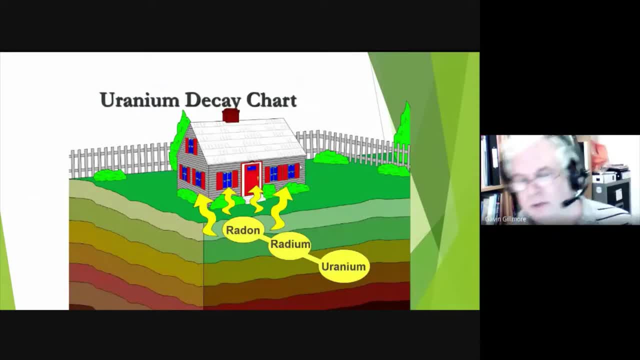 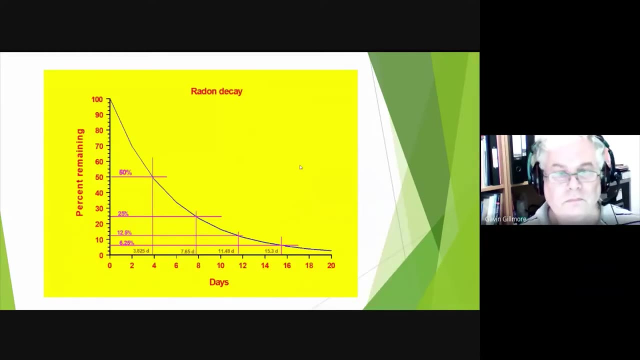 So here's a cartoon of the decay chain. So we've got uranium 238 in the soil and the rocks. That decays to radium 226, which in turn decays to radon. The radon is a gas, and then that can act as a delivery system into a building. 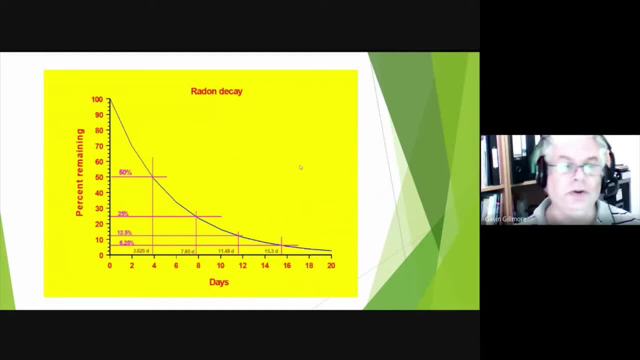 If we think about radon decay, so all things decay given time. So radon has a half-life of 3.825 days. OK, So 50% remains After 3.825 days, then after 7.625 days, 25%, et cetera. 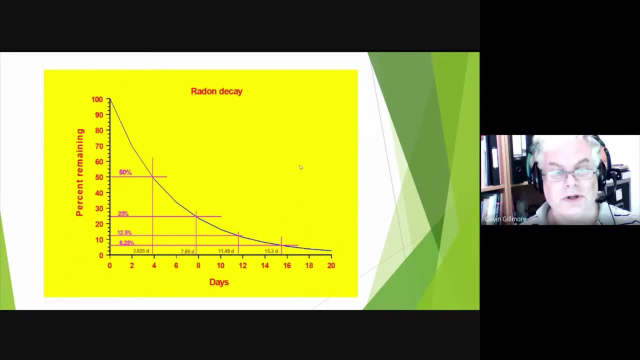 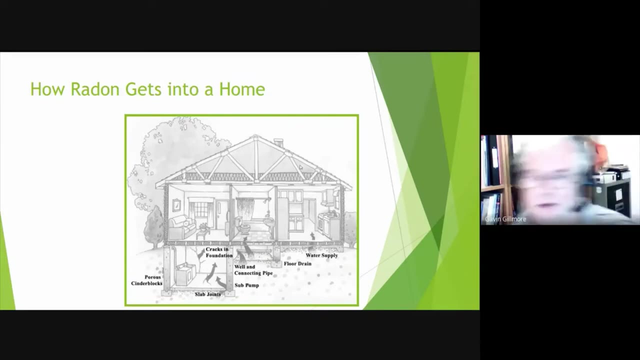 OK, now that 3.825 days is significant because that's enough time for radon to emanate out of the ground into a building and then be breathed in by an individual. So why does radon go into buildings? Well, they go into buildings for a variety of reasons. 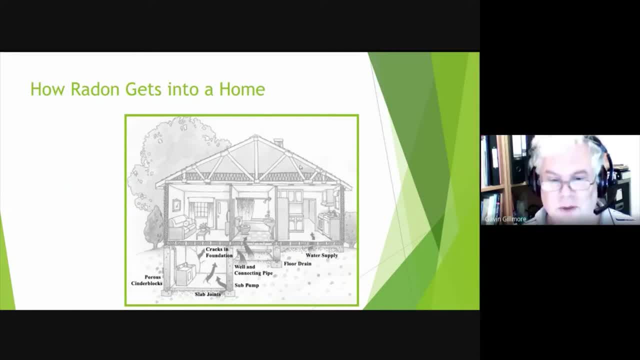 First of all, we build them on the ground, of course, And that ground may be enriched in radium And uranium, which men may give off radon gas. And of course the buildings themselves are porous, So we might have porous breeze blocks, as we would call them. 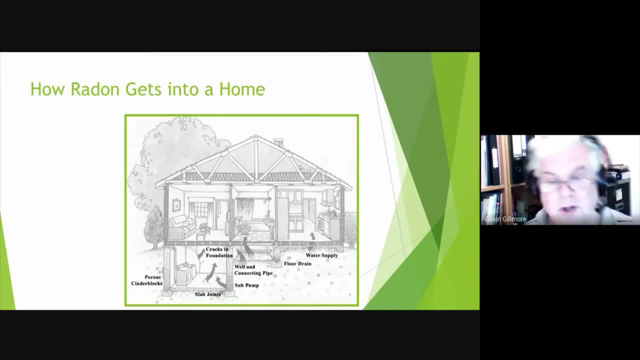 We've also got joints, We've got pipework, We've got cracks, We've got water supply drains- all sorts of potential entry points for gas to go from the soil into the building. The other thing to bear in mind is that wind is blowing over the top. 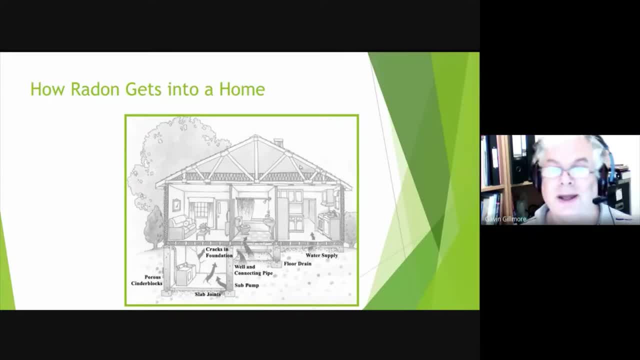 of the building. As wind blows over the top, it's drawing gas, or in this case drawing air, out of the building, So that creates a negative pressure effect. It's called the chimney stack effect. You're also heating the air, of course, in a property, so that's causing the air to rise. 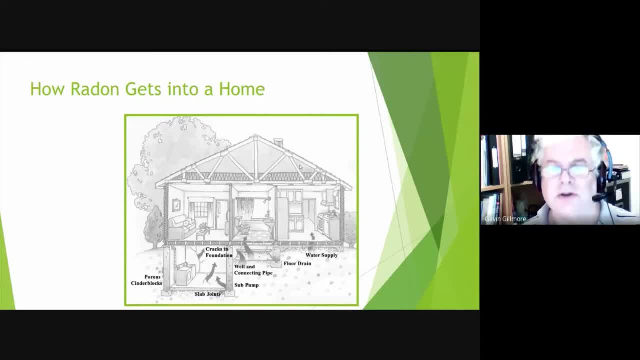 The very fact you've got a building creates an area of negative pressure, because air is pressing down on the building rather than the air in the building. So all of these things come together to create a negative pressure zone which, of course, will attract radon from the ground into the building. 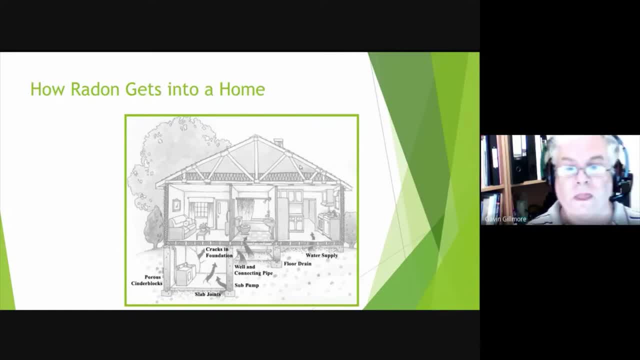 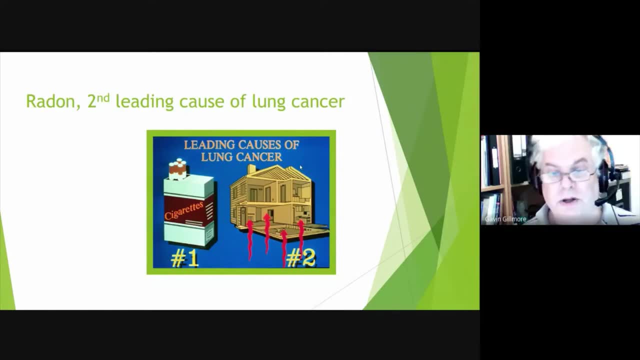 And it's the same for any ground gas. So radon has been recognized as the second leading cause of lung cancer. Now the actual numbers are debatable, depending on the maths and also the secondary smoking and how many numbers you can attribute to secondary smoking. 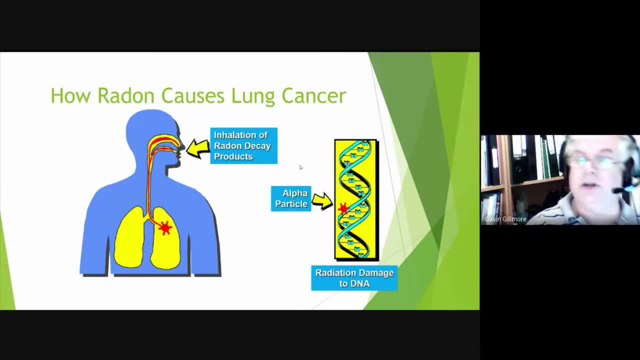 So how does it do it? Well, of course, radon, as I said before, is essentially a delivery system. So radon itself, It is radioactive. So you breathe the radon in. it goes deep into the lungs. Most of the radon you've breathed in just is breathed straight out again. 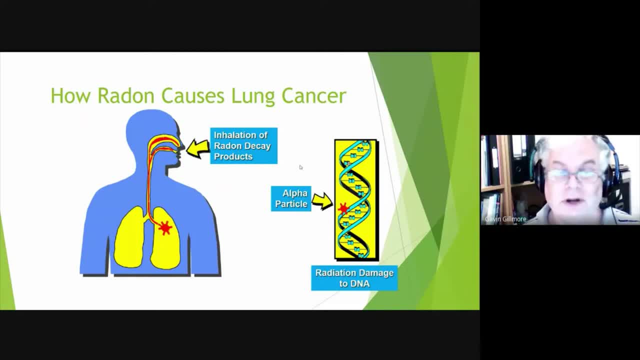 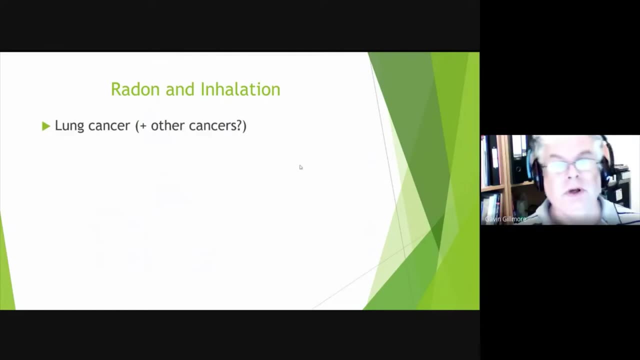 But what remains are alpha particles from the decay of radon, And those alpha particles can cause cellular damage, damage to DNA, et cetera. So there has been a link with radon and lung cancer, although it can take 20 years for the 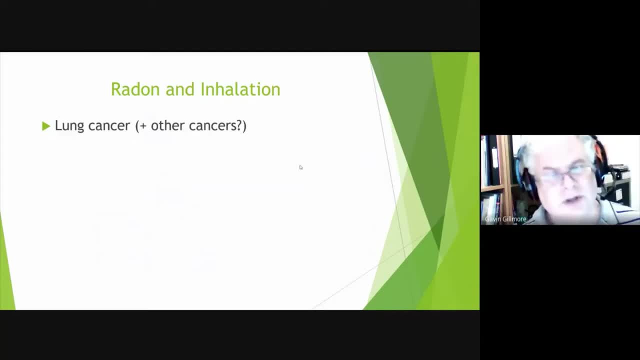 lung cancer to develop And there's also been a link to other cancers. But those other cancers, the studies on that, have been quite contradictory at times. So radon decays to form radioactive particles. Those particles can actually remain suspended in the air. 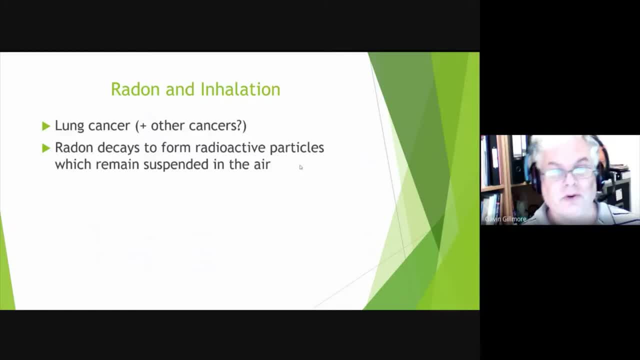 So not only can you breathe in the radon gas, but you can also breathe in the radioactive daughter products, And they particularly may be suspended in the air if you've got water in the atmosphere or particulate matter. So radon is a very important element. 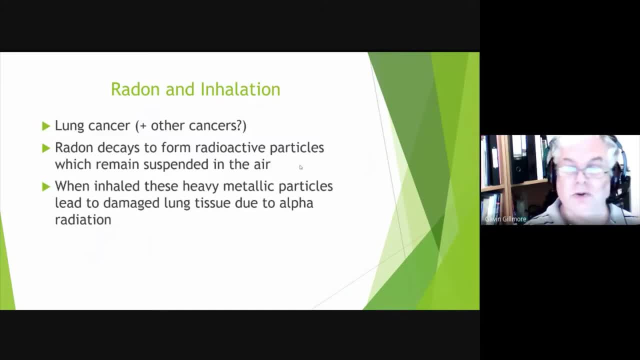 So, when inhaled, those heavy metallic daughter particles can lead to damaged lung tissue as a result of alpha radiation. In the US, the Environmental Protection body there has suggested that 20,000 deaths per year are caused by radon-induced lung cancer, although, again, the numbers vary. 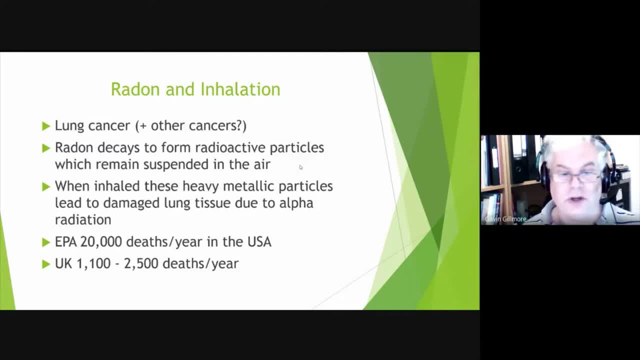 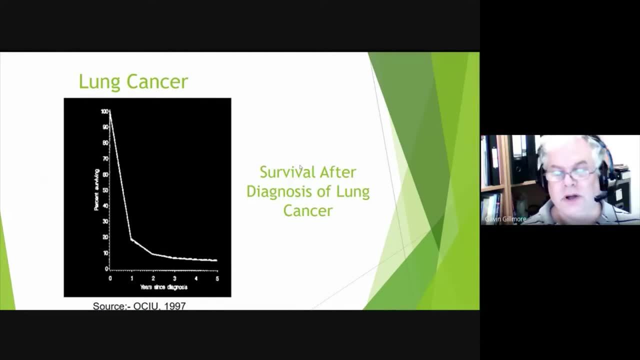 And in the UK anything from 1,100 to 2,500 deaths per year have been associated with alpha radiation. So when inhaled, those four factors are associated with lung cancer. The thing to bear in mind is the survival rates from lung cancer are very poor. 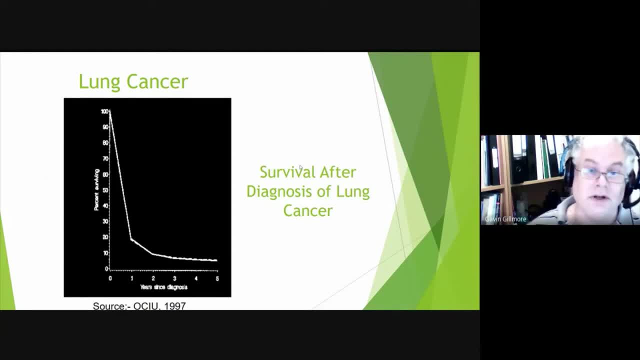 So this is based on 1997 data. Nevertheless, the curve doesn't look much different today. So after 1 year: 20% survival. After 2 years: 10% survival. OK, So if you made it after 2 years after diagnosis, then you had a good future ahead of you. 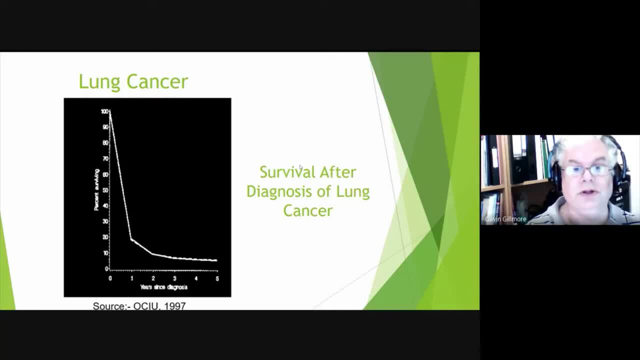 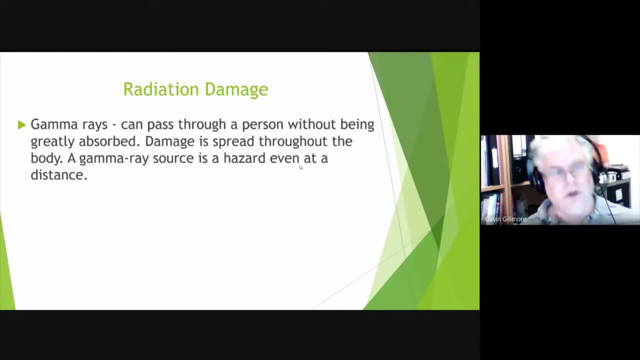 So lung cancer is still a very, very strong, very, very dangerous disease. So that's what we're looking at- is still one of those diseases you don't want to catch or don't want to get. so radiation damage. so you've heard of gamma rays. i'm sure gamma rays can pass through a person without being greatly. 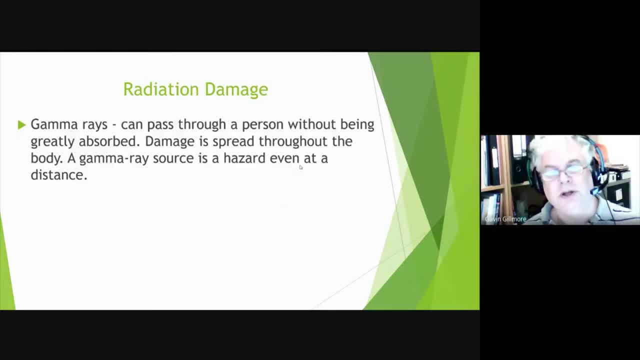 absorbed, it could be. damage can be spread through the body. so a gamma ray source can be a hazard at a distance. so you need something solid between you and the gamma rays. x-ray is very similar. beta particles, or i mentioned earlier, have a low penetrative power. they can penetrate about a centimeter of body tissue. 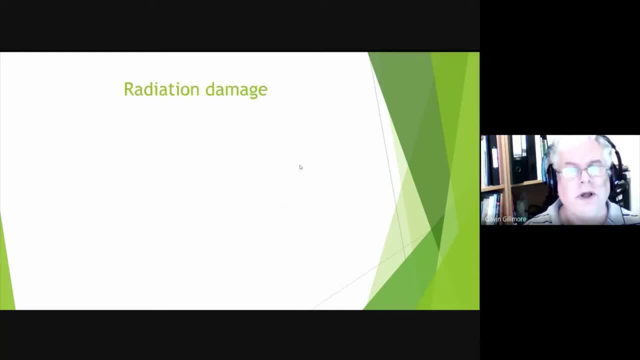 but cause the same sort of damage as gamma rays. alpha particles are interesting because they only penetrate one ten thousandth of a centimeter of tissue. so you think, well, that's not a problem then, surely? but the problem is is that they give up more of their energy over that short distance. 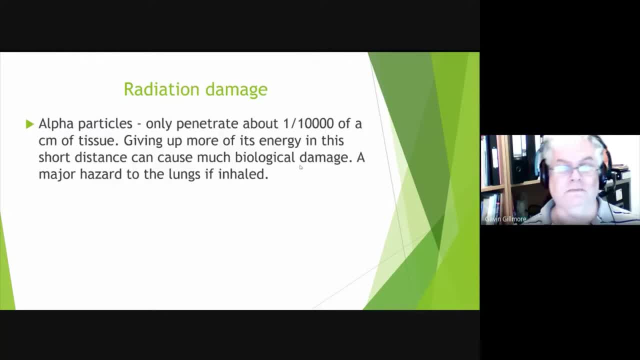 so in theory, they can cause a lot of biological damage. So what you don't want is an alpha emitter inside the body. So, of course, if you're breathing in a gas which decays by alpha emission, then this could be a major hazard. 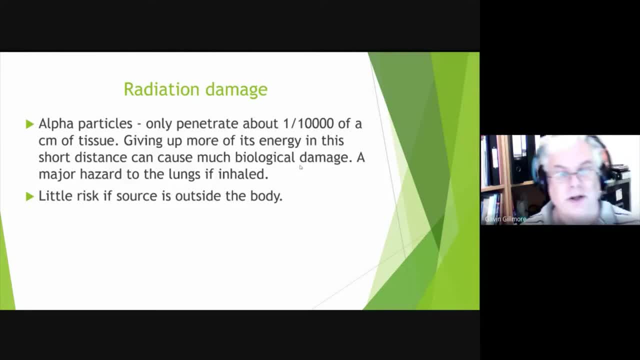 So if the source is outside the body, generally speaking it's a little risk. The dead skin cells on the outside of your body will tend to stop alpha particles, So an alpha particle can be stopped by a sheet of paper. So here we go. 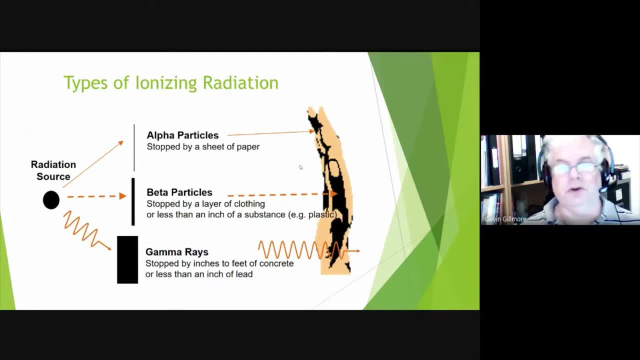 This is illustrated. So we've got our radiation source: Alpha particles being stopped by a sheet of paper. Beta particles can be stopped by a layer of clothing or an inch of a substance such as plastic, or less than an inch Gamma rays. of course, you need something like concrete or lead- certainly something. 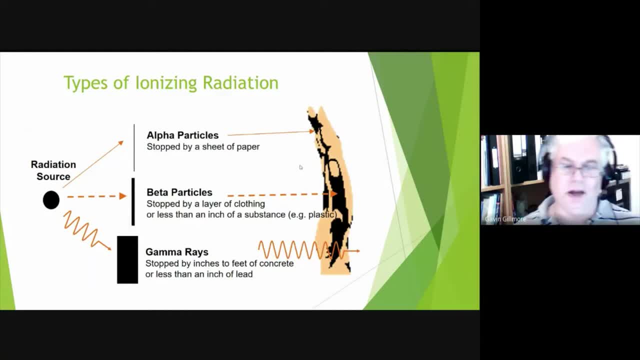 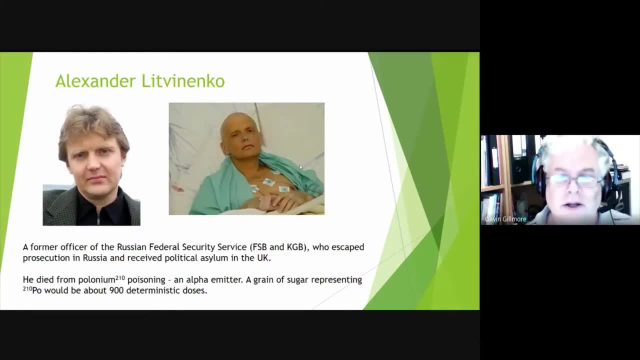 dense barium to actually prevent gamma rays from passing through. Now I mentioned polonium-210.. Because I don't know whether you've heard of it. You remember this, but this is the case of Alexander Litvinenko, who was a former Russian. 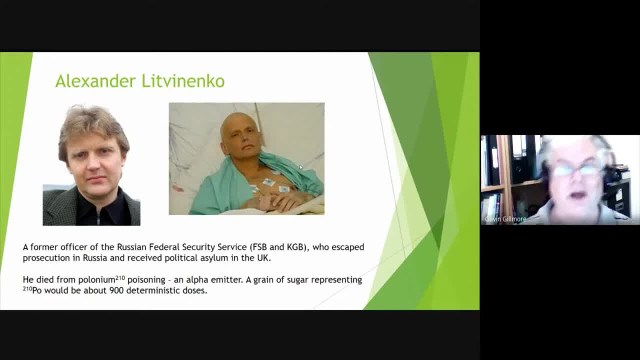 FSB and KGB officer who heavily criticized Putin in various books that he published or became very unpopular in Russia, So escaped and received political asylum in the UK. But he was poisoned using an alpha emitter, So polonium-210.. And people sort of speculate about how much he was poisoned by. 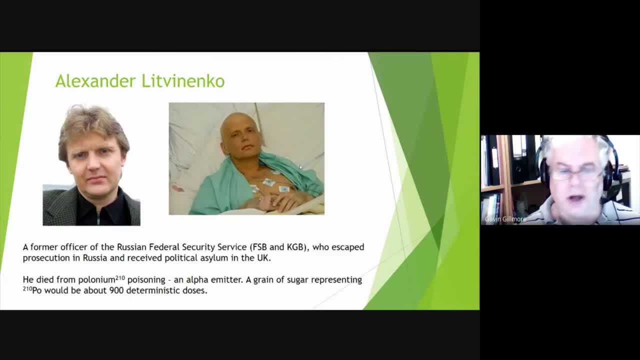 So a little bit went into his tea, But a grain of sugar representing polonium-210 will be enough to kill around 900 individuals, What we'd say deterministic doses. So we have. this introduces the idea of radiation and damage, and there's a big debate of whether. 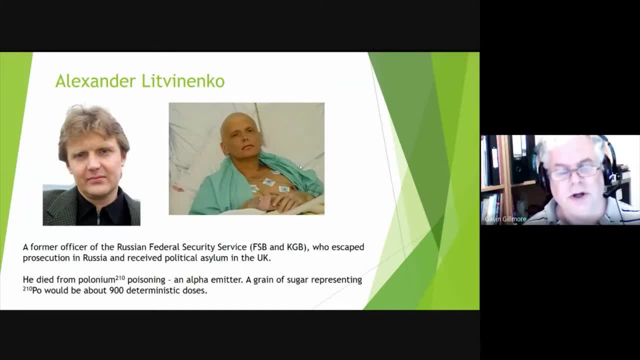 you have what we see deterministic damage, or whether we see what's called linear no threshold damage. So Yeah, So I can talk about that later, But it's, it's an interesting debate. Where do you, how do you, assess the risk? is it basically is influenced by how you look? 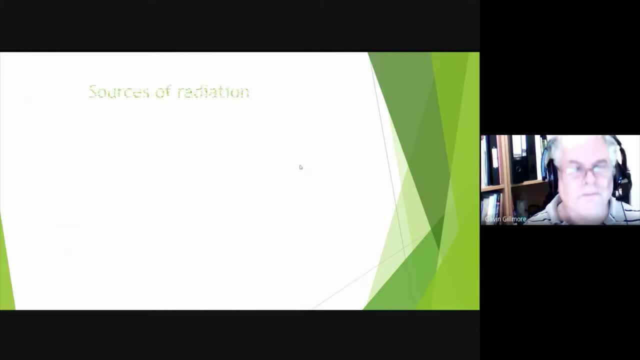 at radiation and its potential damage. So we're all exposed to radiation in our day to day lives. So 15 percent of what we're exposed to is artificial. Eighty five percent is natural And, of course, as we all know, natural is good for you. 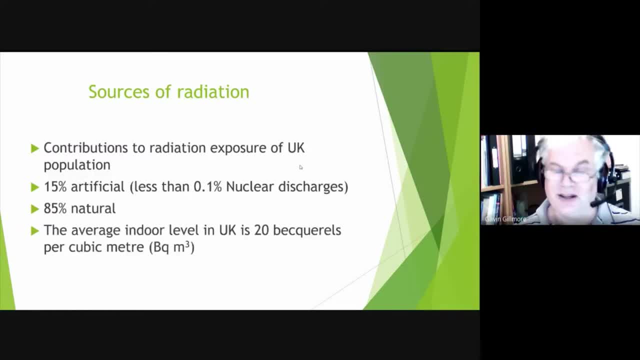 So you can see that the average indoor level in the UK is actually low. It's around 20 becquerels per cubic metre. Bear in mind, the UK action level, as I said earlier, is 200 becquerels per cubic metre. 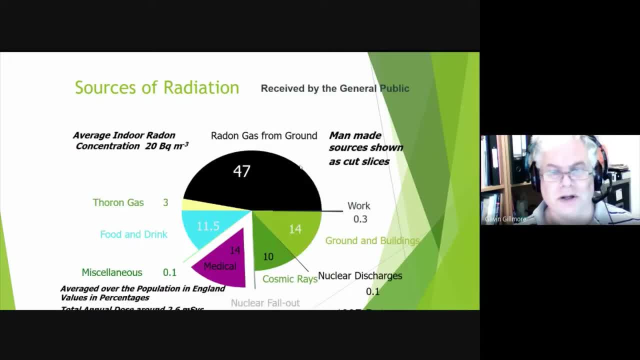 So you might say: well, what are we concerned about? I'll come back to that. So this little diagram, OK, it looks at dose received to a member of the public. So the total annual dose received is around two point six millisieverts. 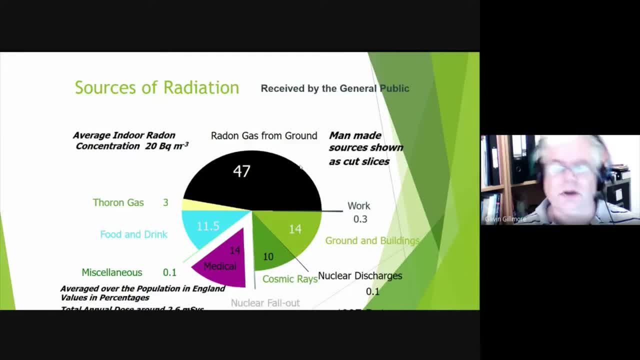 OK, So there are different ways of measuring radiation. We use millisieverts. The states use a different system. Radon gas from the ground counts for something like 47 to 49 percent of our dose. Other exposures- the ground and buildings work, nuclear discharges, cosmic rays, medical 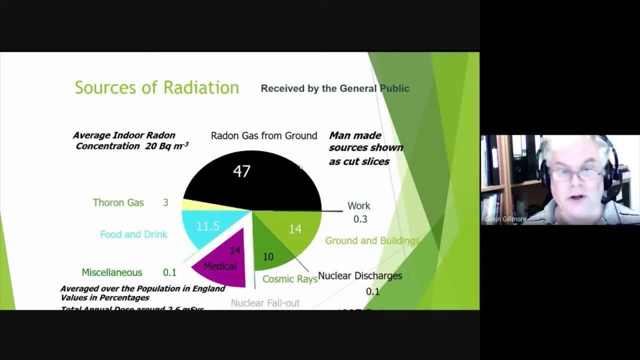 X-rays what we eat and drink. So bananas contain radioactive potassium 40,, for example. Also Thoron gas- I'll mention a little bit about Thoron gas later- has a much, much shorter half life, So is not considered a risk in the same way that radon is. 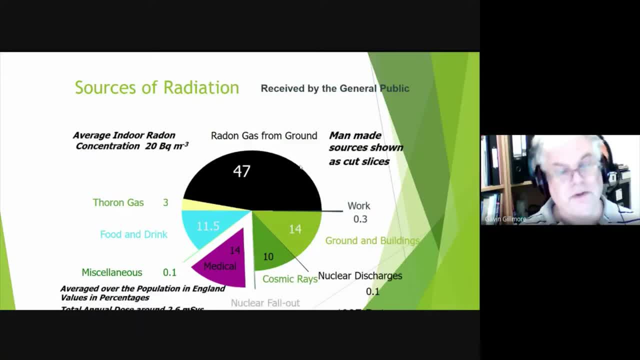 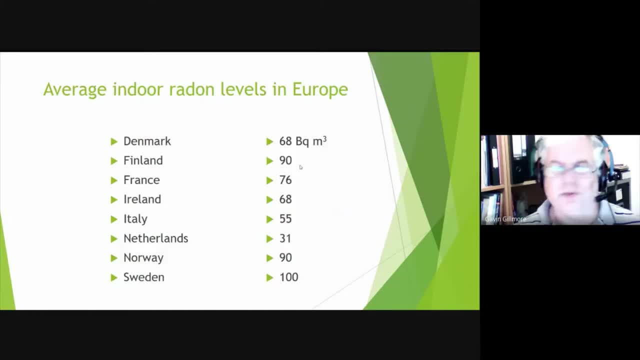 So these percentages are for the average individual. of course, we all know there isn't such a thing as the average individual. So if the UK has 20 becquerels per cubic metre of gas, what's it like in Europe? Well, you can see the distribution here. 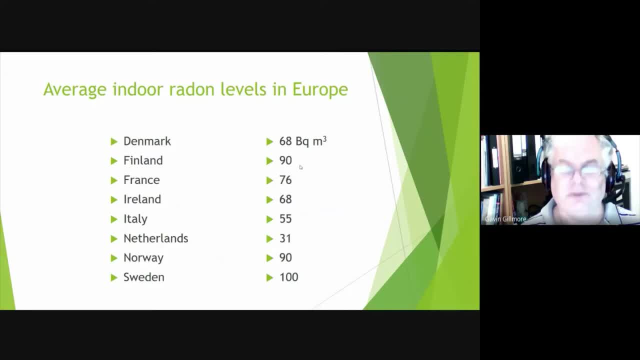 Generally speaking, European countries have higher average indoor radon levels than we do, But our problem is the distribution of that. So Sweden, Norway, Denmark- you can see Finland, So you can see a certain pattern here. So the colder countries have higher radon levels because they have less in the way of. 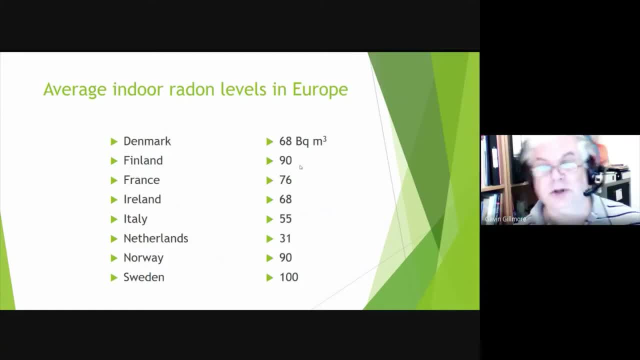 air exchanges per hour of indoor air because they're trying to retain heat and also the underlying geology. So that's a little bit of a risk factor. But you can see that there is a lot of risk factor for the radio in those countries. 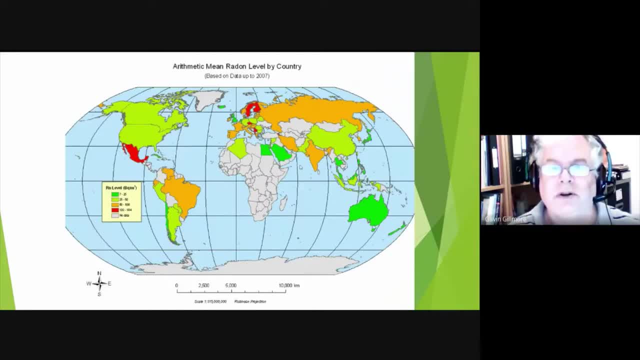 So if we look at a map of the world of radon levels by country, you can see a number of Scandinavian countries have quite significant radon levels. It's raised in Russia as well. India, certain parts of Europe. The UK, by comparison, looks low, but this tells a misleading story. 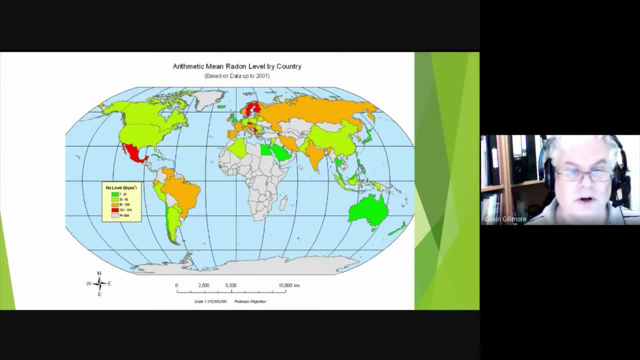 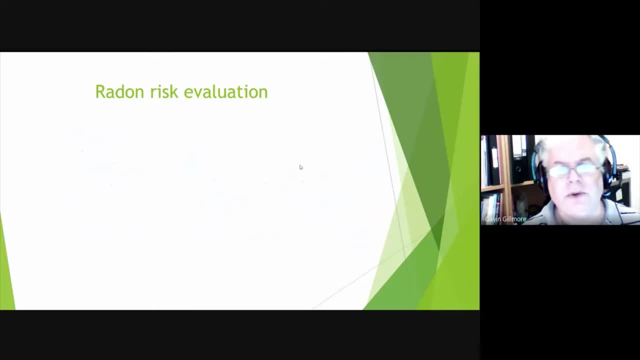 And the same in Australia actually, But then parts of South Africa, Parts of South America look relatively high. So how do we evaluate risk? So some studies have suggested, and the EPA in the States have suggested, that at 74 becquerels 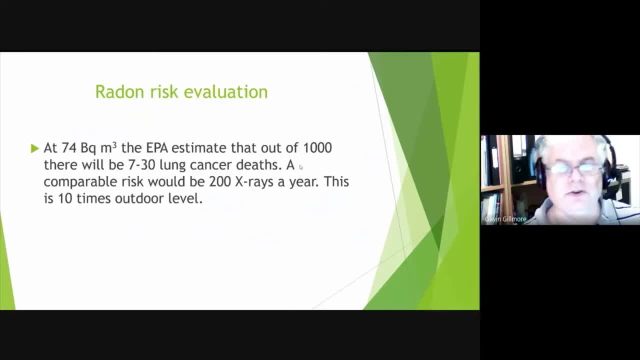 per cubic meter out of 1,000 individuals, there will be between 7 and 30 lung cancer deaths. That's a huge variety in number, But nevertheless You know, 7 to 30 out of 1,000.. 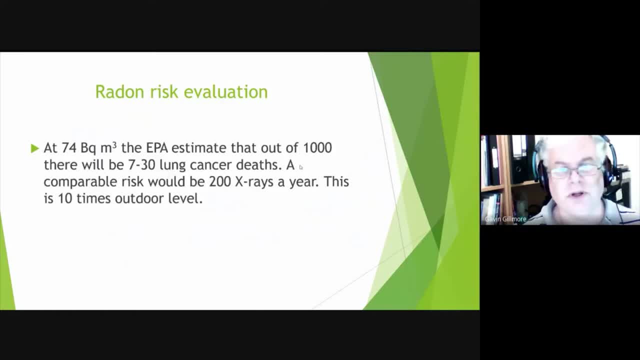 So a comparative risk would be something like 200 x-rays per year, which is a lot of x-rays. So if we up the game and say 7,500 becquerels per cubic meter, estimated lung cancer deaths out of 1,000 will be between 440 and 770.. 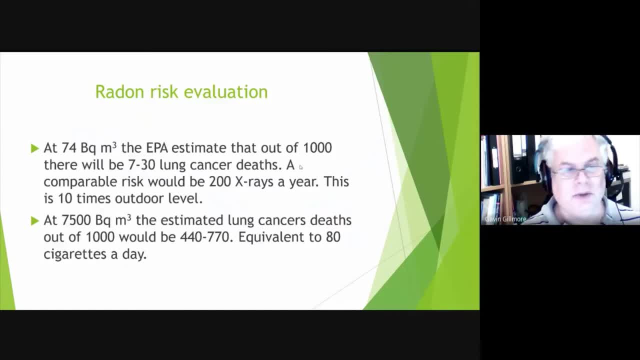 So you'd have to be smoking something like 80 cigarettes a day. Now you might say, well, that's high, And you know 7,500.. Well, we don't get those sort of levels in homes in the UK. 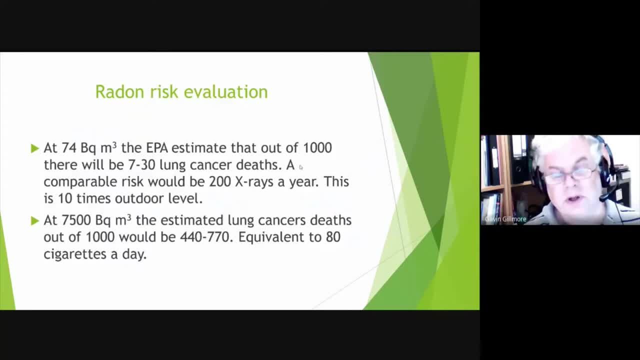 Well, we don't get those sort of levels in homes in the UK, So you'd have to be smoking something like 80 cigarettes a day. Well, actually, in fact we do, And the record at the moment stands for around 22,000, 25,000, something like that in the. 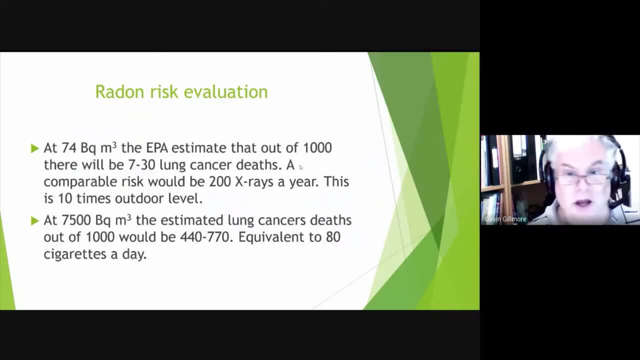 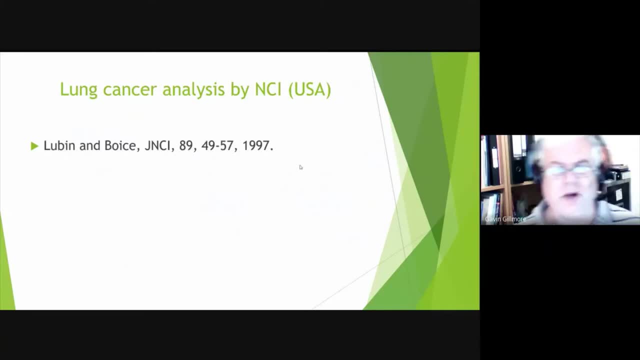 UK- In England, should I say. It has been higher in other parts of the UK. So what do we understand about risk from radon? Well, a lot of this is based on work published in the 1990s, for example by the National 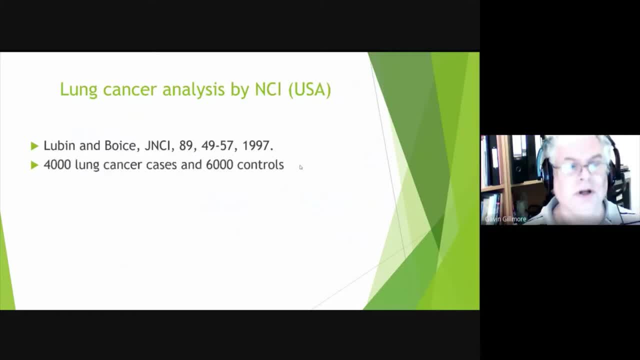 Cancer Institute in the USA. So Lubin and Boyce had looked at a 4,000 lung cancer case study, 6,000 controls And they said there was a significant trend of increasing lung cancer with increasing indoor radon exposure. So they said there was an excess relative risk of 13% for 25 years exposure at the US. 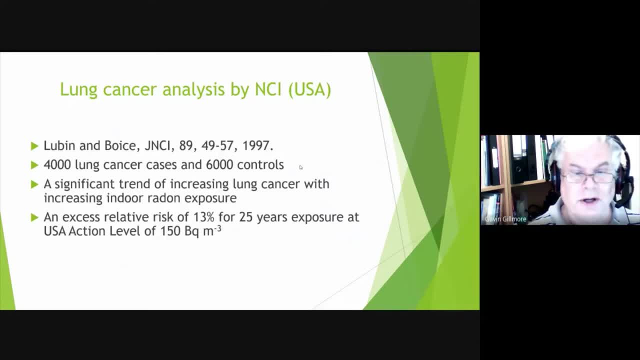 action level of 150 becquerels per cubic metre. Now the US actually, as I said earlier, measure radon differently And they use a measure called a picocuri, So they measure in picocuries per litre. So that's equivalent. 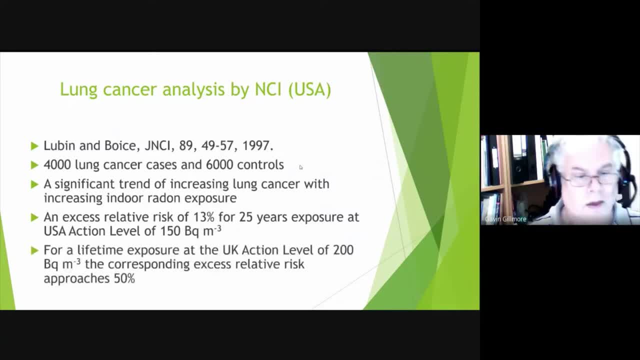 They measure at four picocuries per litre For a lifetime exposure. at the UK action level of 200 becquerels, the corresponding excess relative risk approaches 50%. So that might beg the question: why do we have an action level of 200?? 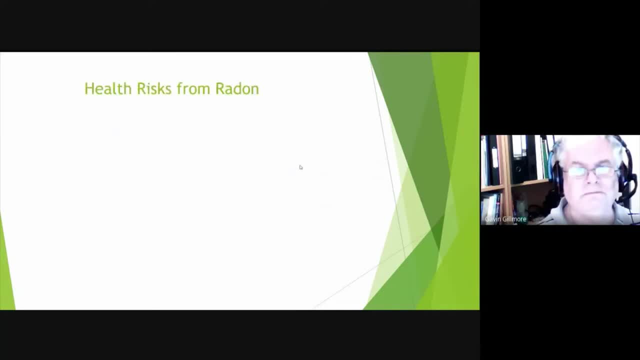 That's a very good question. I will come back to that. So there's also been a lot of studies done looking at lung cancer risk amongst uranium miners And they've noticed actually that there's a significant risk in terms of increased lung cancers amongst miners generally. 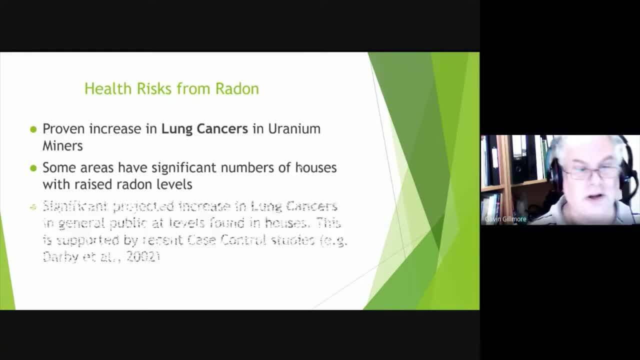 Some areas also have significant numbers of houses with raised radon levels. There's a significant projected increase in lung cancers in general public at levels found in those houses And that's been supported by a number of- I say recently it was 2002, case control. 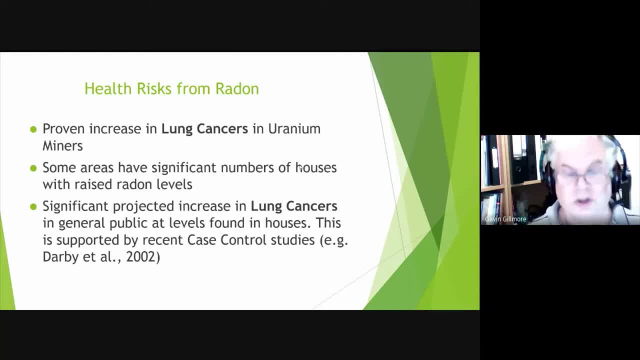 studies, The DARBA et al study. They conducted a study in 13 European countries, very comprehensive study, And they concluded in actual fact there was no safe- in inverted commas- level for radon. So we might say there's an action level in the UK above which we should remediate. 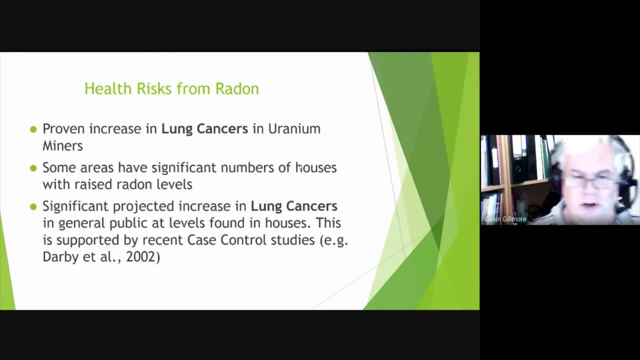 But in fact the DARBA et al supported the idea. well, there were no boundaries that were safe as such. So the World Health Organization has recommended that Radon in homes be kept at 100 becquerels per cubic meter or less. 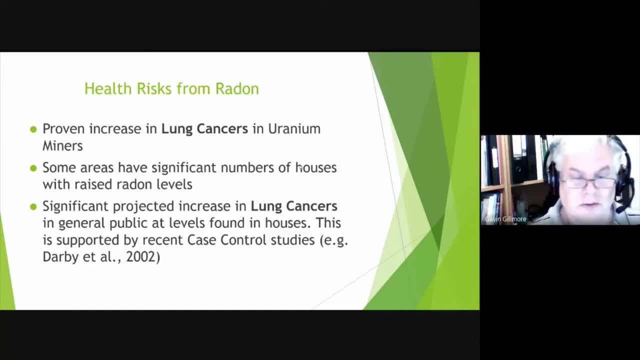 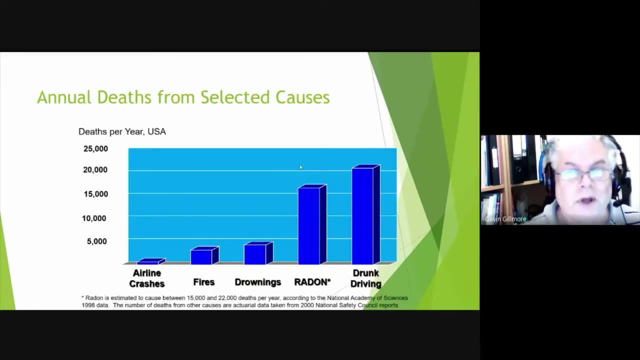 So the UK has now introduced what is called a target level of 100 becquerels. So they kept the action level. But if you do remediate then you have to try and get it below the target level. So we say, well, yes, we can see that there's an issue with radon. 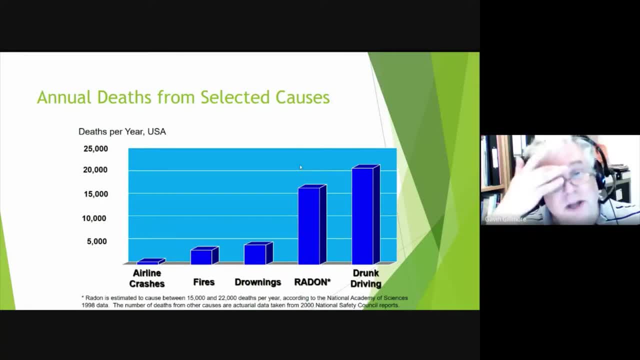 How does radon compare with other risks? So this is deaths per year. in the USA. You can see airline crashes, fires, drownings. There's a lot of risk. There's a lot of risk, But you can see that there's also a number of things. 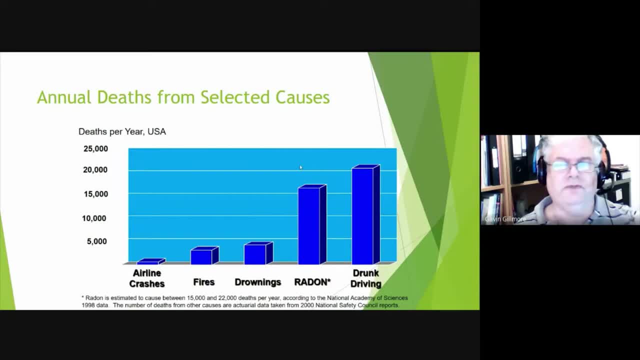 Radon and drunk driving. So notice this- just over 15,000, 16,000. So this is the lower limit. So the limit for radon in the US is between 15 and 22,000.. So drunk driving is more significant than radon. 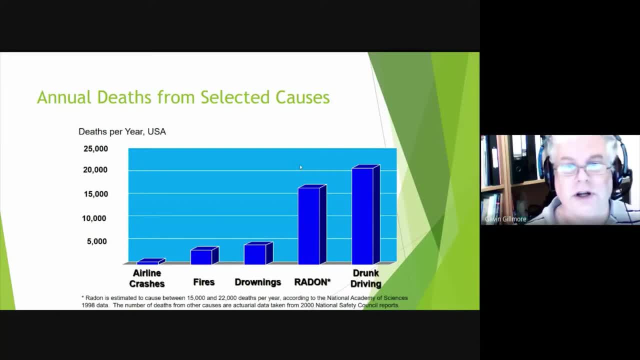 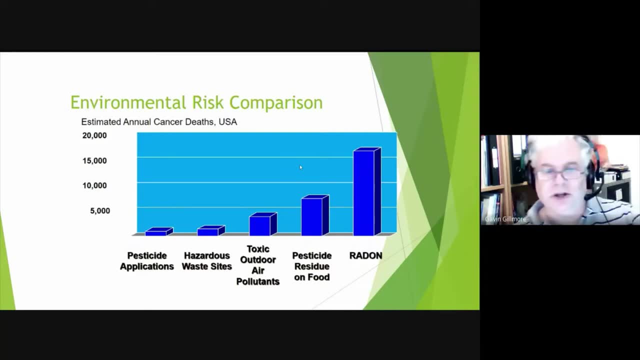 But fires and drownings and airline crashes are significantly less in terms of annual deaths. And then, if you look at estimated annual cancer deaths And other sorts of toxic substances, as it were, you can see pesticides, hazardous wastes, toxic outdoor air pollutants, pesticide residue and then radon. 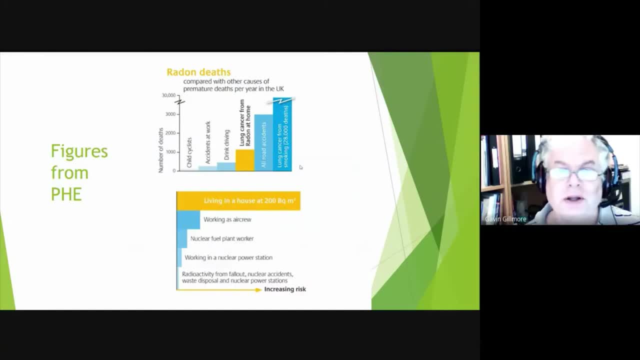 and this is from the uk's public health england body and you can see they're comparing the number of deaths. so this is premature deaths per year in the uk amongst child cyclists, accidents at work, drink driving, then lung cancer from radon at home and road accidents and lung cancer from smoking. 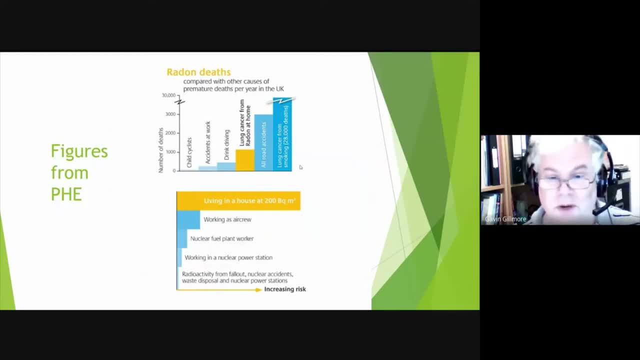 and then the bottom figure shows: you know, living in a house at 200 becquerels and the risk compared with working as aircrew. as aircrew you're exposed to cosmic radiation- nuclear if you're flying, of course, nuclear fuel plant workers working in a nuclear power station, radioactivity from fallout on nuclear accidents, etc. 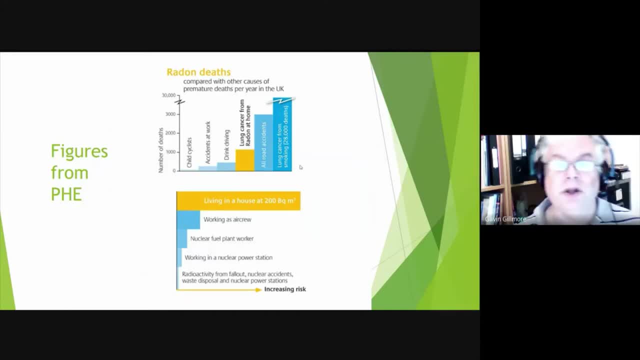 uh. so, coming back to the top figure, um, the. as those recent studies have shown, actual fact, the worst combination is smoking and um living in a home with high radon. there's a synergistic effect and actual fact, if you smoke and you live in a high radon home. 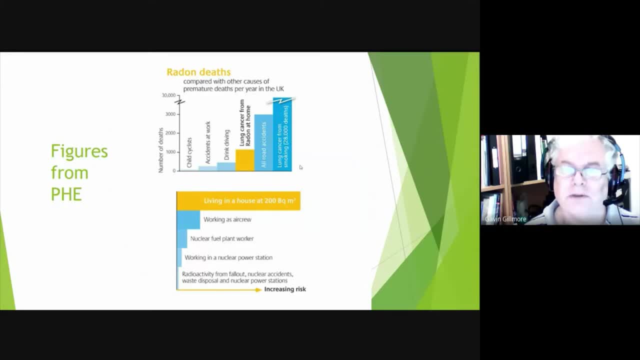 then you're 16 times more likely develop lung cancer. so you either don't smoke, which is the best option, or, if you do smoke, don't live in a radon affected area. so here's another example looking at risks in the uk compared to world risks. 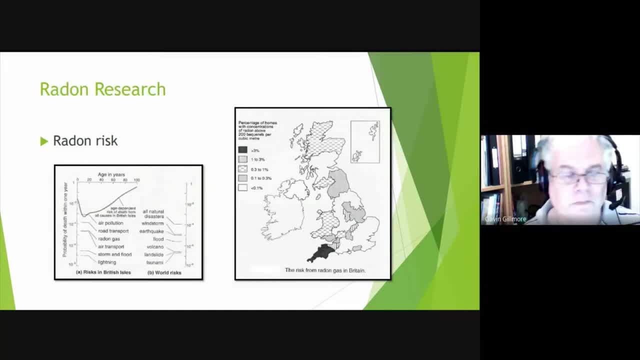 you notice, for the uk, radon gas is quite high. there, air pollution is high. of course we don't have volcanoes or tsunamis as a general rule, and then you can see the radon risk from uh on the map on the right and you can quite 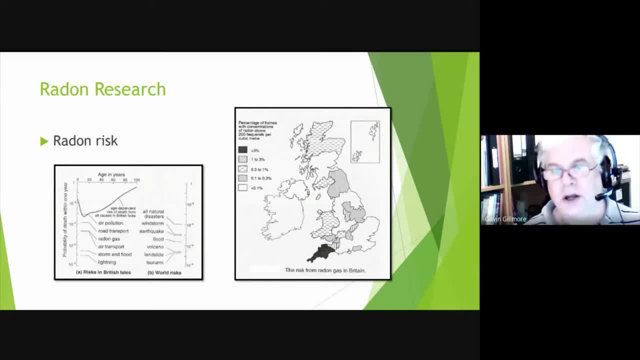 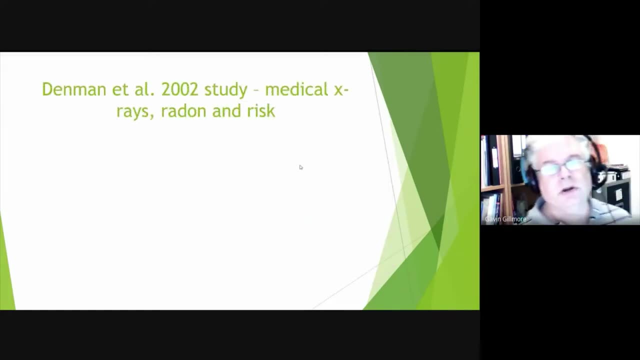 clearly see. you know um greater than three percent uh higher radon risk um in southwest england but you can see that bath and northeast somerset um doesn't get away without some risk. so a colleague of mine, damon et al 2002, who is a medical physicist working in northampton at the 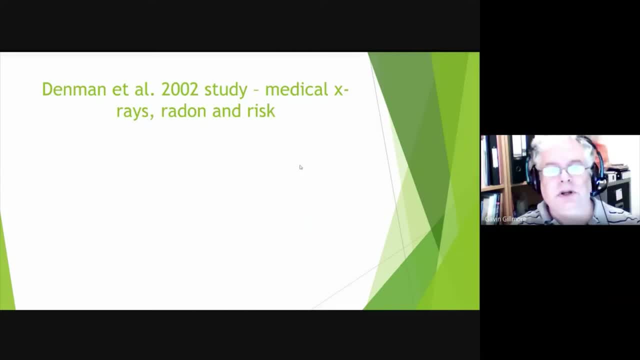 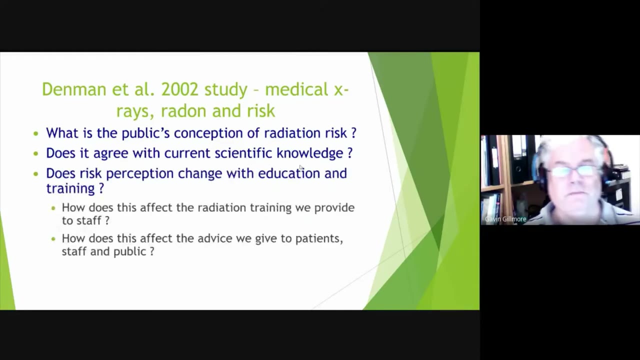 university and also in the hospital. so well, let's compare medical x-rays, radon and risk and people's perception of risk. so how do people pursue, perceive radiation risk and do their views align with scientific knowledge? and if you train and educate people, how does that affect risk perception? 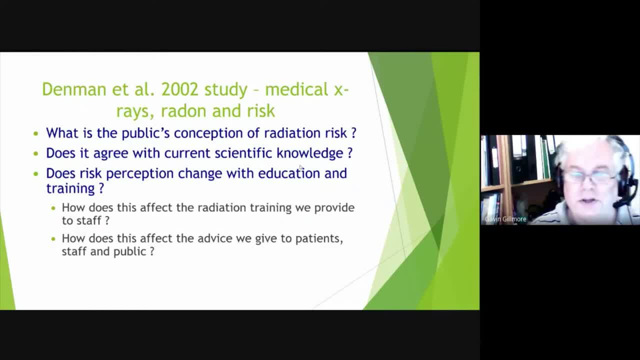 so, um, you know how then should we give advice to people such as patient staff and public, etc. so there was something like 115 returns from the questionnaires and they looked at school children, they looked at trainee nurses, some of my undergraduate students and staff, the national cancer institute. 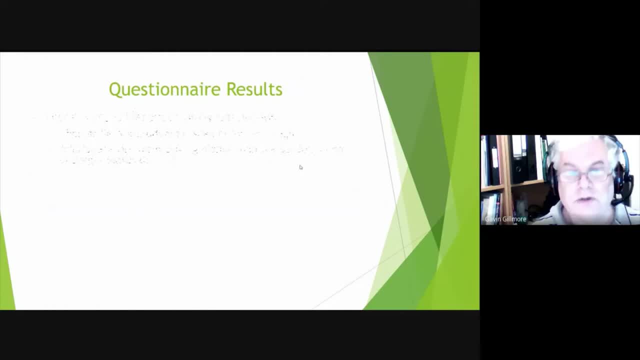 institute, national cancer research center, as well. um, so there were significant differences between groups. not surprisingly so. the school children placed radon very high, and they did that because they'd just been told about radon. uh, adults rated risk from driving higher than the students and undergraduates did. nearly everyone considered radon to be more of a. 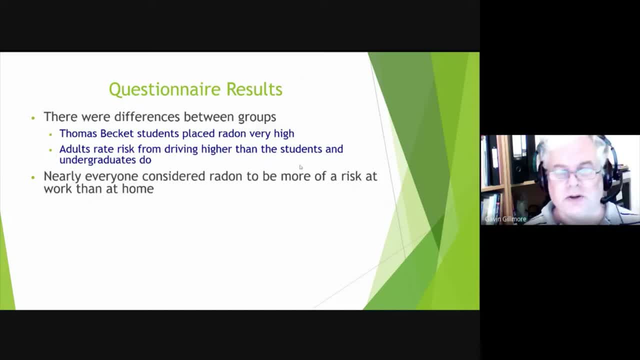 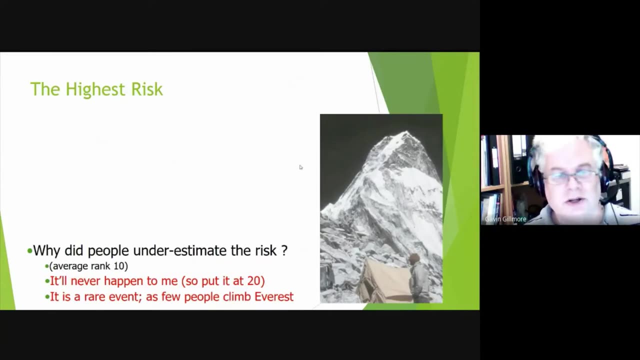 risk at work than at home, but then that's illogical when you think about it, because you spend longer at home. everyone overestimated the risks from living near cellar field, mobile phones, transmitters, coal mining and driving. so what was the highest risk? so their risks were 1. 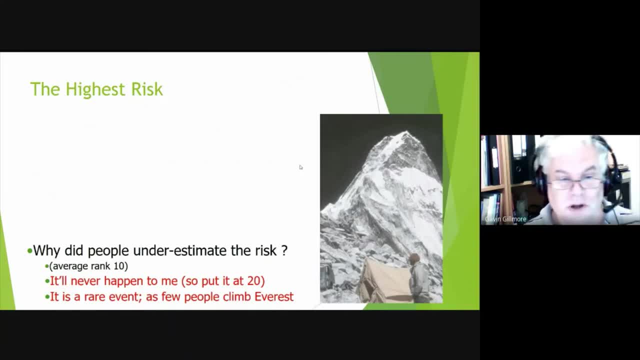 to 20. okay, so 20 was the lowest, one was the highest. well, actually climbing everest was interesting. so between 1921, 1998, over a thousand, a sense of everest- 160 deaths above base camp. so you're only 10 times more likely to die on the ascent, but you could still die on the descent. 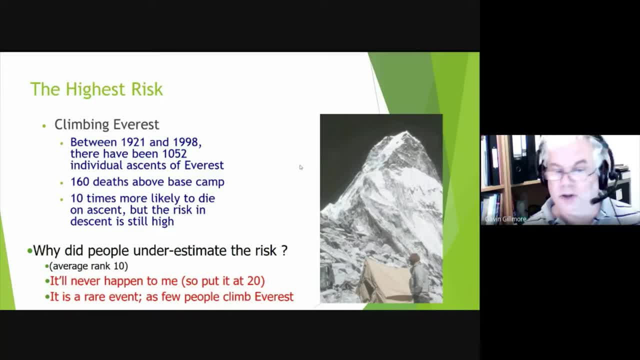 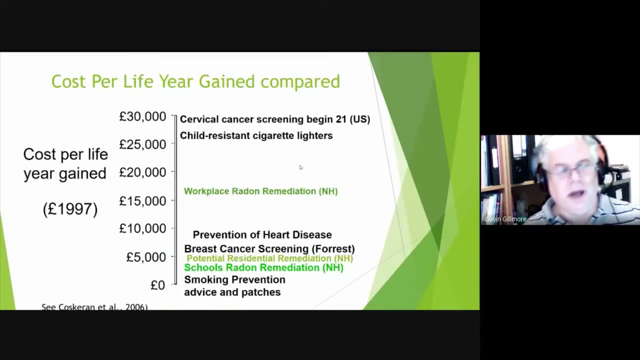 okay. so people underestimated the risk. put it around 10 out of 1 to 20 scale. and why is that? well, it'll never happen to me because i'm not going up everest. but also some people said, well, it's a very rare event, few people go up everest, so reasonable. so you say, well, okay, let's think. 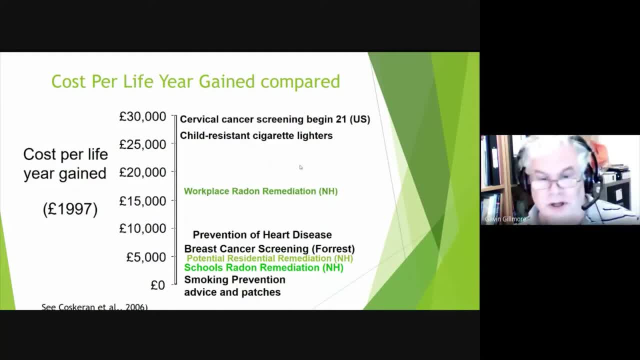 about the cost of remediation. so you can remediate a property. you can put in a sump under the floor which creates a low pressure zone that draws the gas to the sump. you can then put a pipe that goes outside of the building to vent that gas. okay, so what would happen if we did all this kind of work? 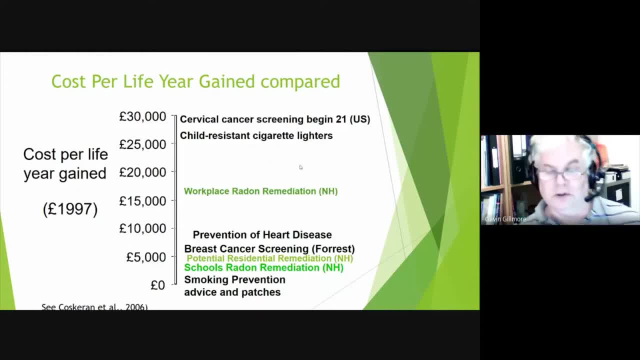 and we sort of talked to people and got people to measure the radon in the first place. so this looks at cost per life year gained and this is work that i was involved in back in the early 2000s and you can see- you know smoking prevention relatively cheap. 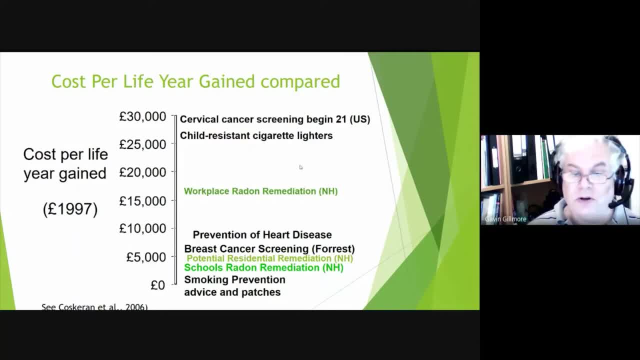 in terms of device and patches, schools, radiation remit. so red on remediation is relatively cost effective. potential residential remediation is cost effective. then we've got things like breast cancer screening, prevention of heart disease campaigns, workplace radon, child resistance, cigarette lighters, etc. now the reason it says potential. 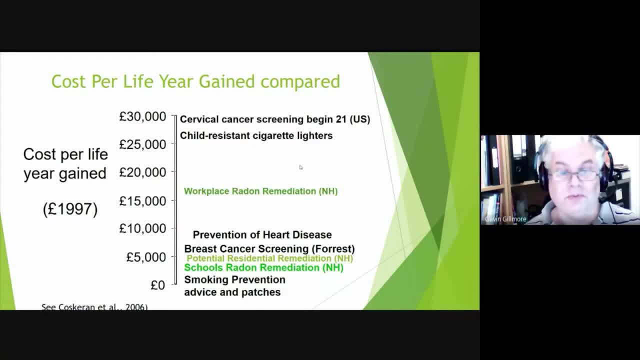 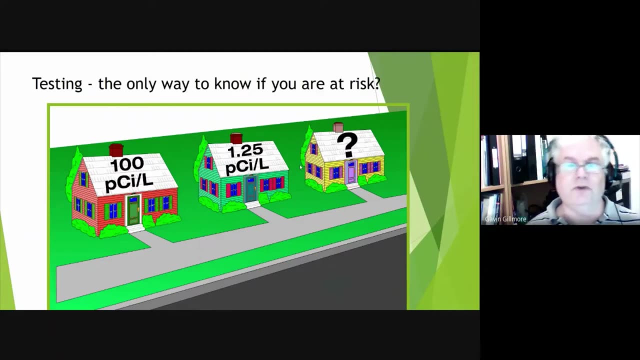 residential remediation is that actually a lot of people would test, or some people would test, but even though they knew they had a high result, they didn't do anything about it, and so that affects the cost per life year gained calculations. so here we've got three buildings. this is from the usa, so it's in picacurys paleta. 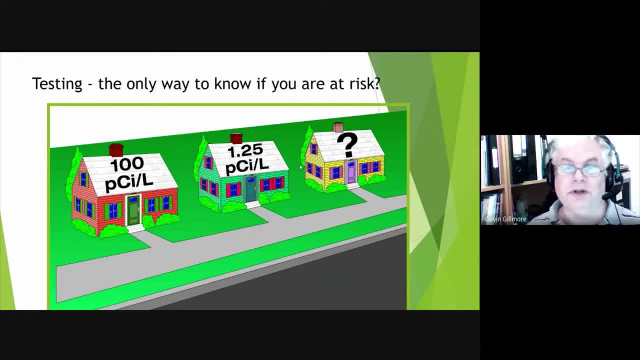 so we've got one home. remember i said four picacurys paleta was the action level equivalent in the us. so middle home hasn't got a problem. left-hand home clearly has a problem, right-hand problem- who knows? so, um, the rodent council has always said the best way to know is to test. 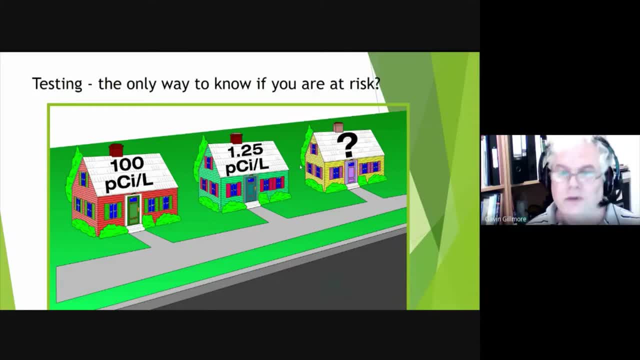 um, of course, what can vary between homes? the home can be built in a different way. one could have cracks in the floor. uh, they could be lived in in different ways. some people like fresh air, some people don't. some people heat their homes more than others. some roofs may be more leaky than 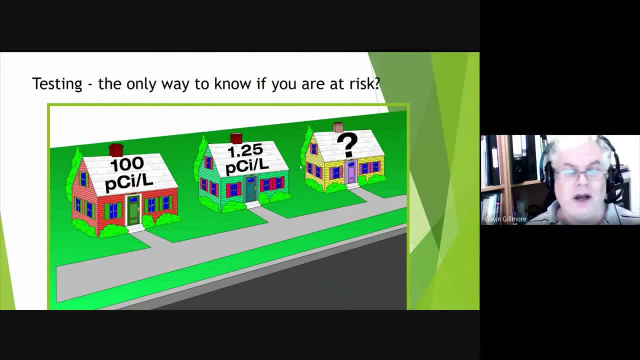 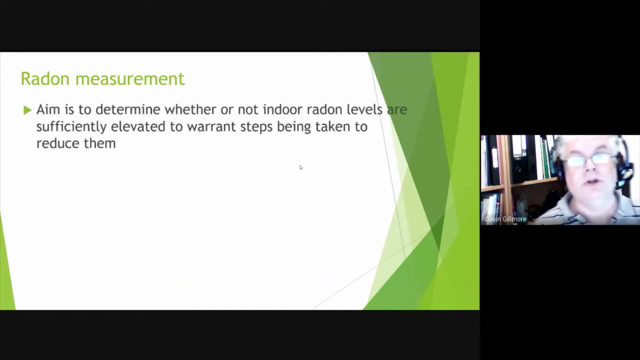 others in terms of air. um, the left-hand house might have an uranium or load beneath it or a fault beneath it, along which radon can travel. um, so we, we don't know. so, um, ideally, you want to measure. so the idea of measurement is to determine whether or not indoor radon levels are sufficiently. 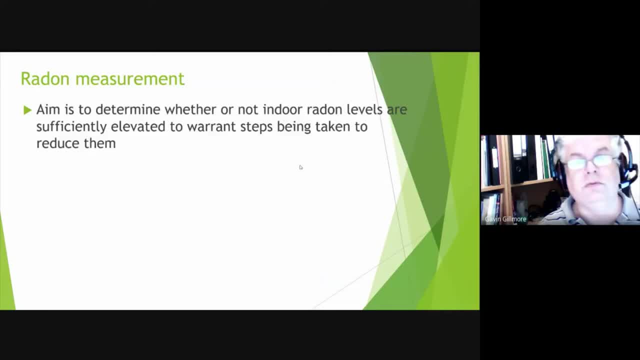 elevated to warrant steps, um, to actually reduce those levels, in other words, to take remedial action. so, and then also, if you've taken remedial action, you need to think, well, has it been successful? ideally, when you're doing measurement for risk and radiation risk, you want to measure over a. 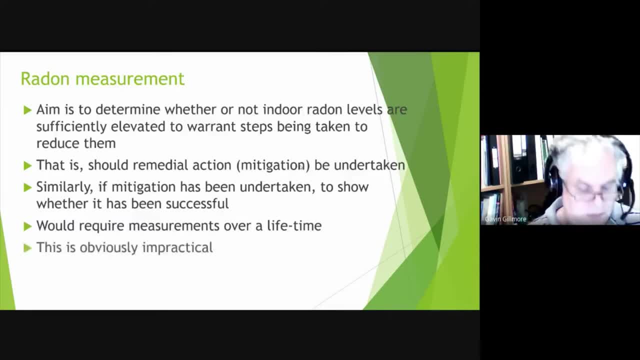 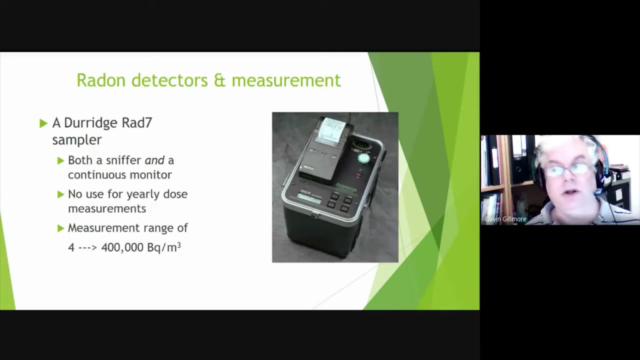 lifetime. that's clearly impractical. um, so you'd actually measure over short periods of time, okay, but then you need to somehow scale that up. i'll come back to that in a minute. so there are lots of different ways of measuring radon. uh, this is just one device. this is called a durage rad 7 sampler, one that we've got a couple of these. 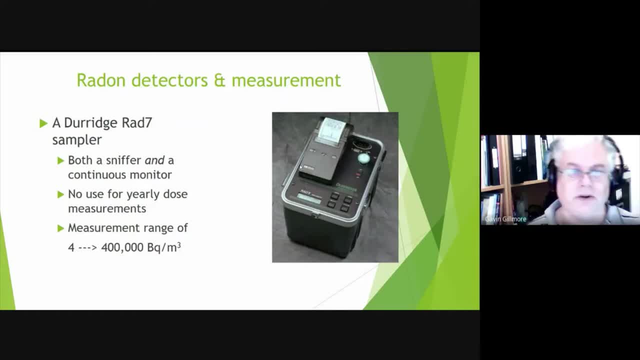 at bath spa university and this is a device that we've got a couple of these at bath spa university and this is what we call a radon sniffer and a continuous monitor. okay, so it can give you, you know, hourly results or half hourly results, can be very accurate machine, but you can't use this. 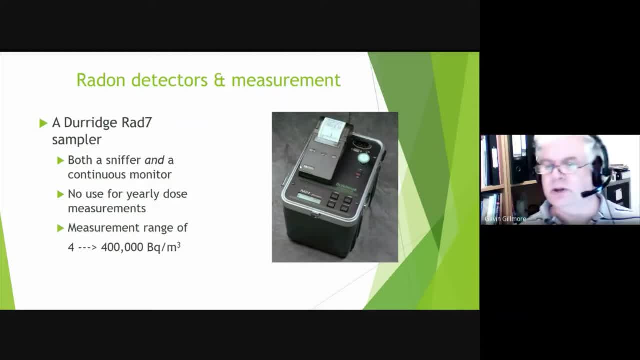 for a yearly dose measurement has a very good dynamic range: anything from four becquerels up to 400 000 becquerels, or higher than that, if you calibrate it in the right way, um, but this is not going to give you what you're going to be able to do. is you're going to be able to calibrate it in the right way, um, but this is not going to give you a. 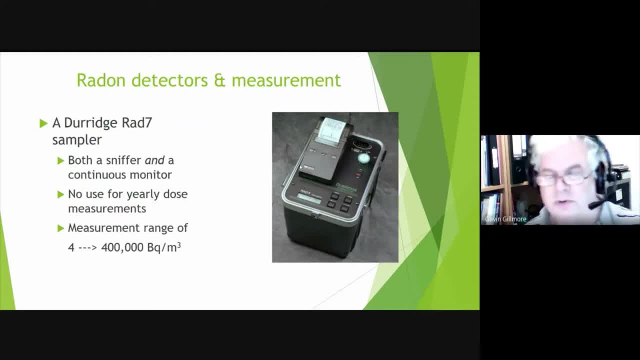 what we call a time averaged result. this is going to give you an actual result at that moment in time. radon varies enormously through the day. okay, so actual fact. if you're going to measure for a certain period of time, you probably want time averaged rather than um active, um devices such 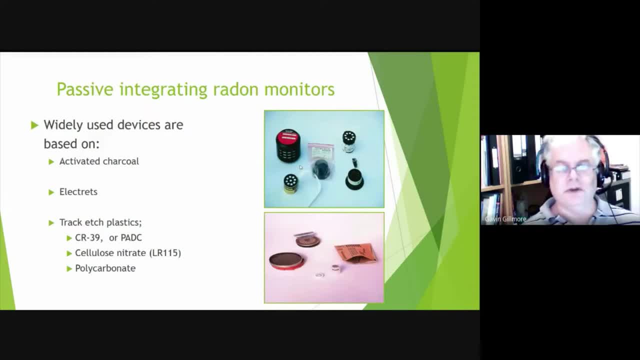 as this. so these are what we call passive devices mostly, so electret's slightly different. um, i won't say too much about those because we tend not to use them very much in the uk, uh, and we tend not to use activated charcoal these days either, but this is used in the states. 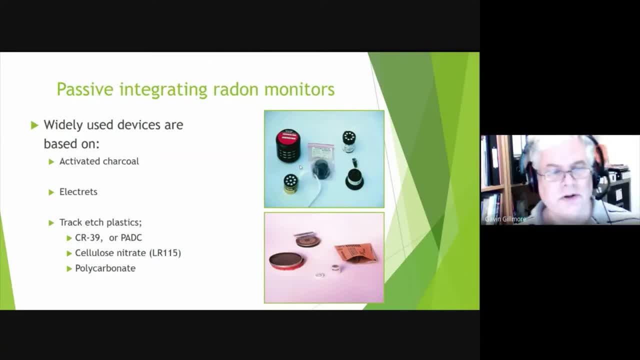 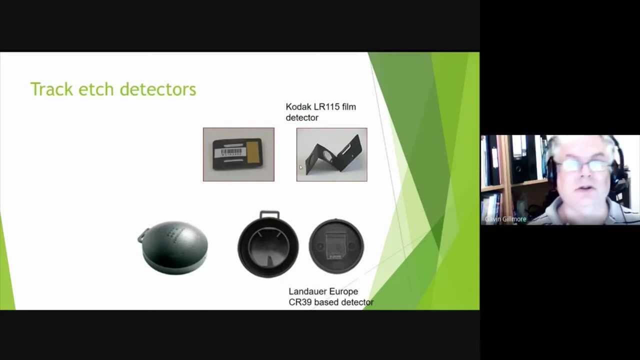 what we tend to use in the uk are track etch devices- and i'll say a little bit more about these- and there are various different versions of track etch devices. lots of different manufacturers, as you see, produce different looking devices. so these are two typical track etch detectors. 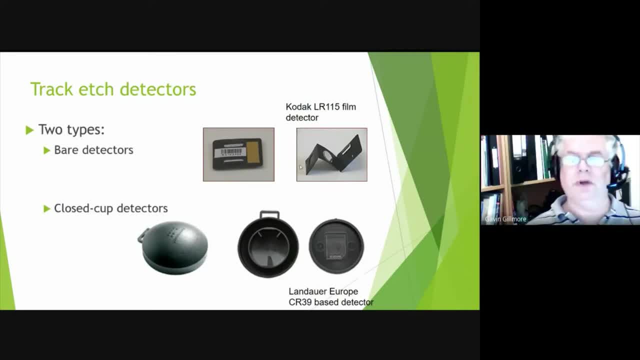 so one is called a bear detector. so it's a bit like, um, you know, a badge that you would wear for radiation detection and you open it up and it's made of a film and basically, as the alpha particles impact on that surface, it changes the character of that surface. 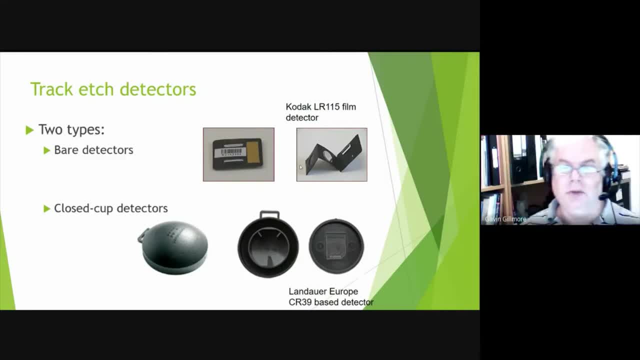 and the bottom one is called a closed cup detector. in theory, the advantage of the closed cup is that it's designed in such a way that only radon can pass through a very narrow gap between the bottom and and top parts of the plastic detector and you can see the detector. 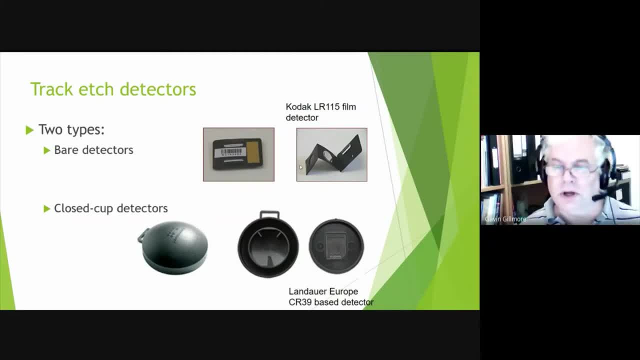 itself actually in the device. okay, so the little plastic square that you can see is the detector itself. so this is a special type of plastic, a bit like plastic used for glasses and things like that. it's called cr39. it's the type of plastic and basically alpha particles will strike the plastic surface. 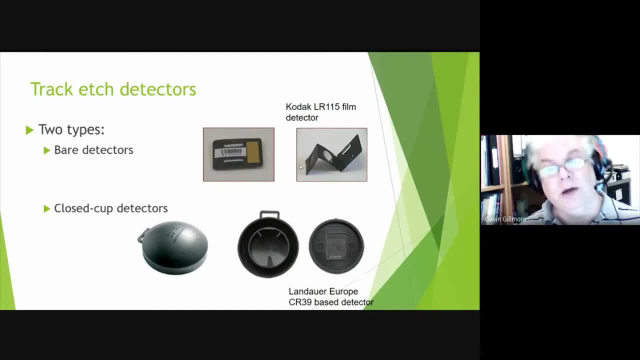 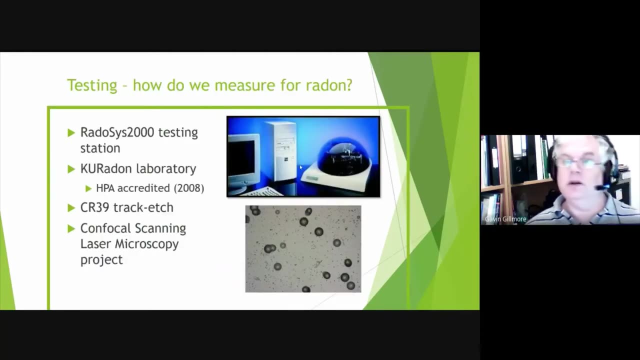 damage the structure of that surface and then by putting that device into acoustic soda solution, that etches the damaged plastic and we can then see the etched tracks, as they're called, hence track etch detectors. so again, there are lots of different ways that you can actually look at those. 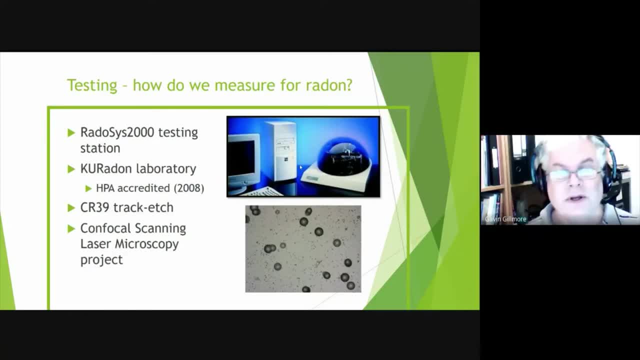 tracks. so this is just one system that we have at bath spa. so this is called a radarsys 2000 and it's a domed. you see the domes feature on the right is an automated microscope powered microscope and before i came to bath spa i was at kingston university. 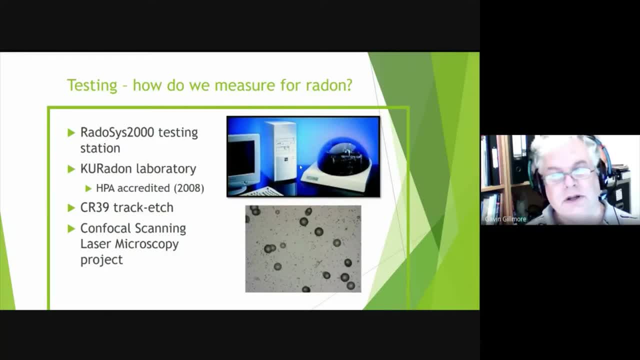 and we ran a hpa accredited laboratory called k radon at um at kingston and we're just setting that up in bath spa. so it actually looks at 39 detectors, counts the number of tracks per a given area and then is able to then calculate the amount of gas in the atmosphere. so you can see. 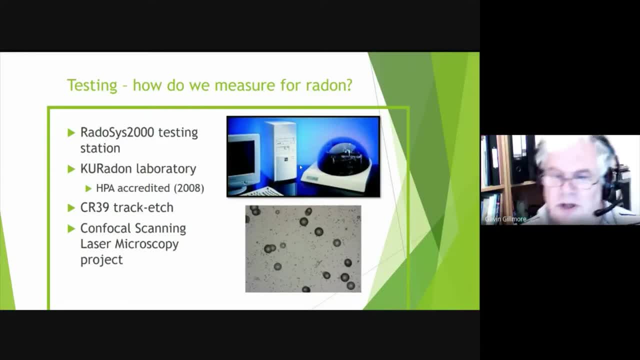 a 2d image below, not a terribly clean image, but you can see a series of pits or tracks and you can see some of them are combined. uh, so some are individual, some are angled. okay, so we can take such a device, this cr39 detector, and we can further scan that using a cone focal microscope to improve the measurements of radon. 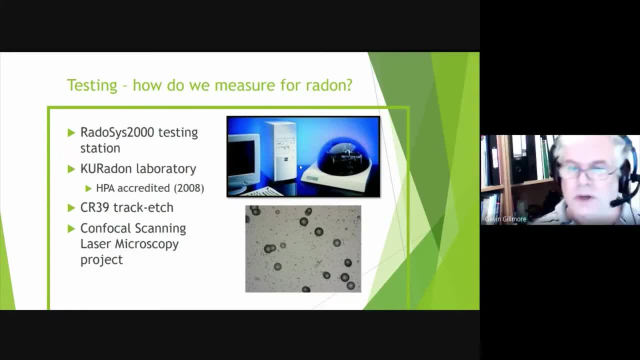 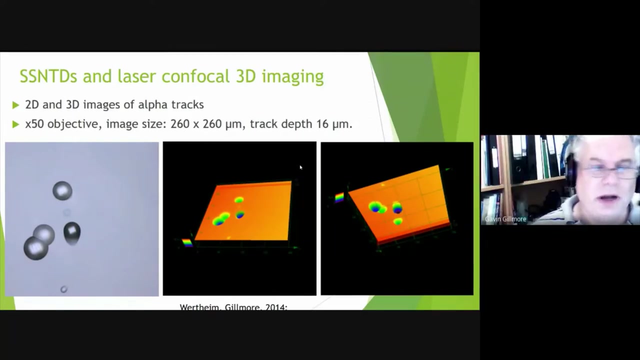 so one of the issues here is that the automated system will basically fit a circle around each track and count the number of tracks, but of course if you've got combined strikes then it's not able to differentiate between some of those strikes. so here we've got images taken with a confocal, so we've got 2d images on the left and then 3d images. 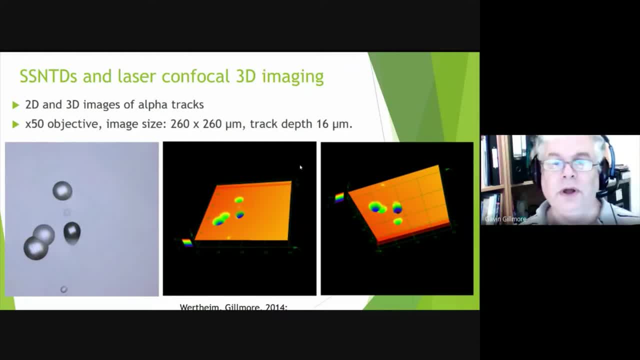 in the middle on the right you see a top view and a bottom view and the track width is about 20 microns and depth is about 16 to 20 microns as well, and you can actually spin that around. so we have got a little video clip that my colleague 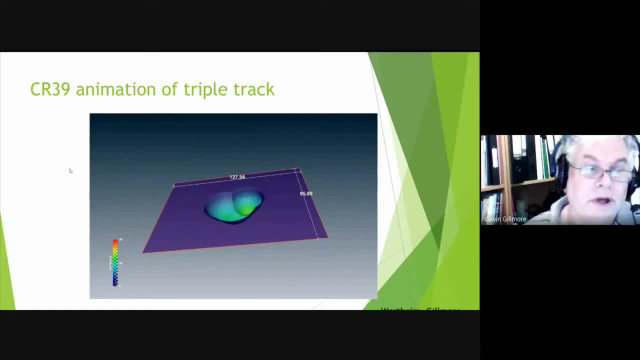 David Gertheim, Professor Wertheim at Kingston University put together on work that we were doing and you can see this is a triple strike. now this would be a problematic for radon readers to read. so if we run the little video clip you can see what we can do with it. 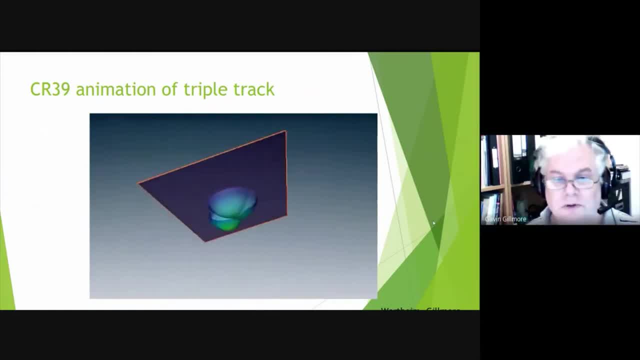 okay, so you can see we're spinning it round, we're looking at it all different angles. we can measure the depth, the width, um, we can also look at which strike happened first and with that all the information can tell us about what alpha particle may have created the track. 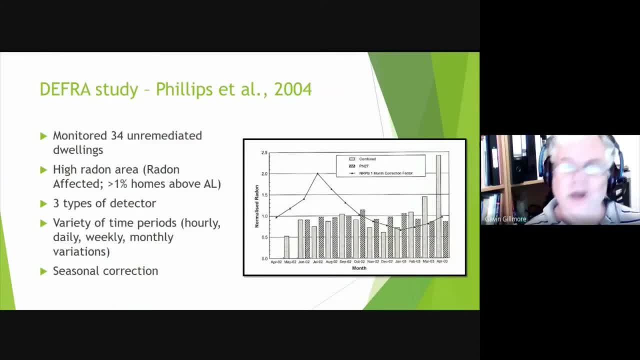 So back in 2004 I was involved in a DEFRA study looking at unremediated dwellings, and one of the issues we were looking at was different measurement types. what was the best type of measurement that we could use? We looked in a radon affected area. 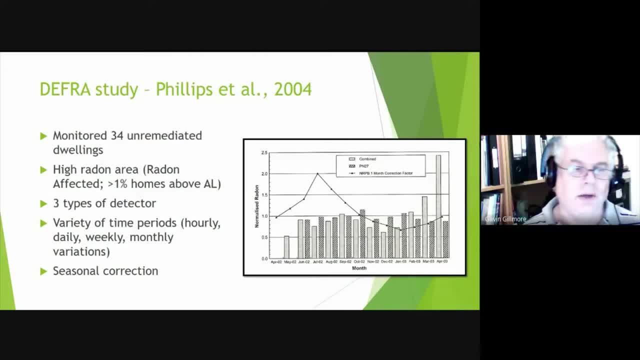 and we looked at three types of detectors over a variety of time periods, looking hourly, daily, weekly, monthly variations, and we were also looking for seasonal variation. Okay, so on the figure on the right, you can see when it says NRPB- one month correction factor. 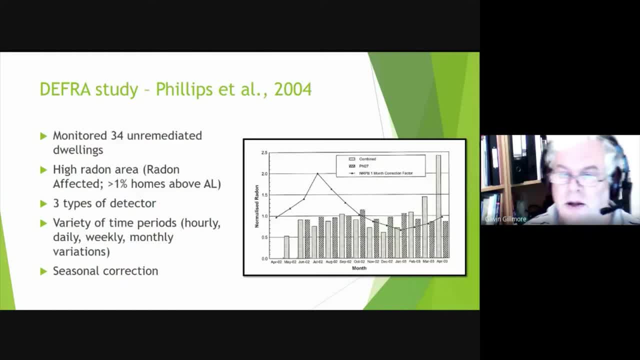 so that's the National Radiological Protection Board, as it was back then, and you can see there's a sort of a curve. and then the data, that the columns are basically the radon measurements taken with different devices, and you can quite clearly see that our pattern, 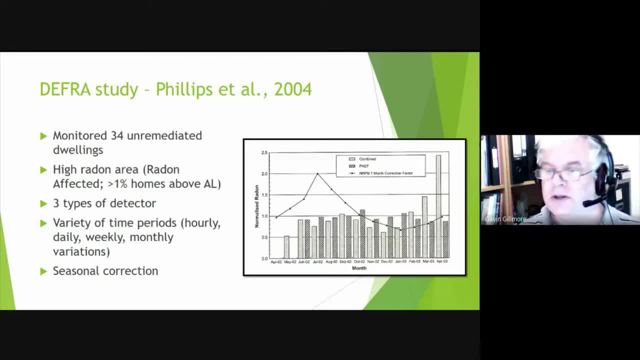 of radon doesn't fit the correction factor curve. So the idea is that you could measure in July, apply the correction factor curve and then that will give you an average result for the year. Fortunately, if you did that with this database, you could see you'd end up with a. 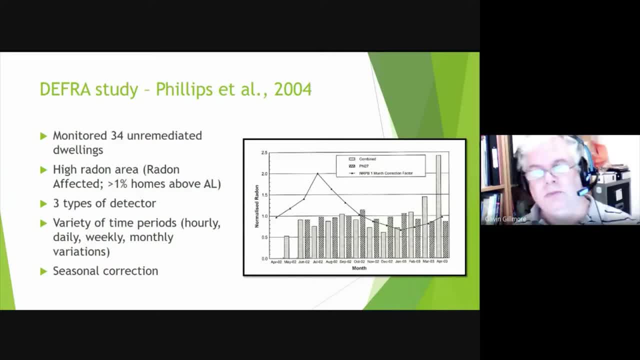 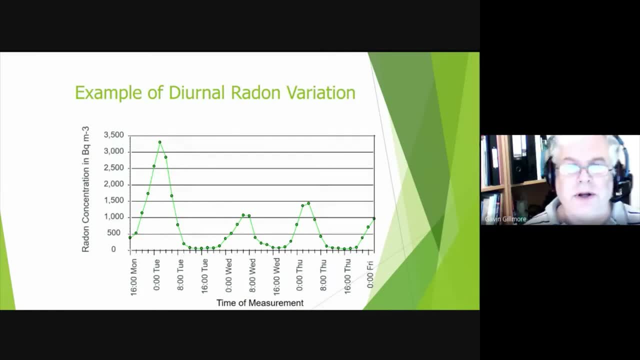 the wrong result, And that was because of different conditions within the ground. So the other thing we have to bear in mind is that we see a huge amount of variation in radon. So this is actually a good example of real data from the DEFRA project, showing you diurnal 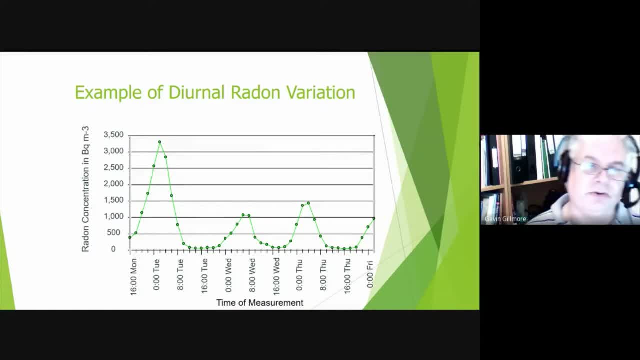 variation and you can see peaks up to 3000 becquerolles or more. I normally think, oh, this is very disconcerting, but you can see there is a slight power margin due to the numbers that we're trying to get in the data, and this was done atbil玅rden for us, But we did have a very good. 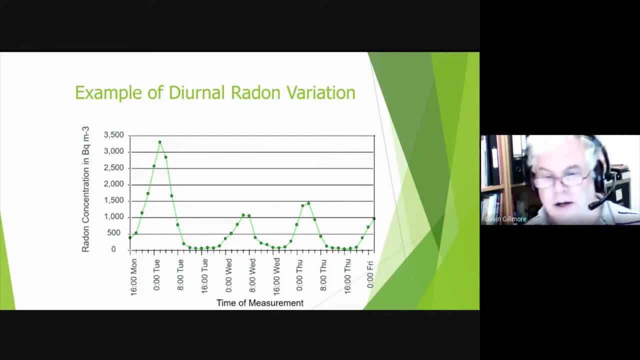 then the levels dropping right down during the day, peaking again at night. So this was a building that was closed up at night so radon could build up to high levels. open during the day and then the radon dissipates. But how then do you assess the risk? 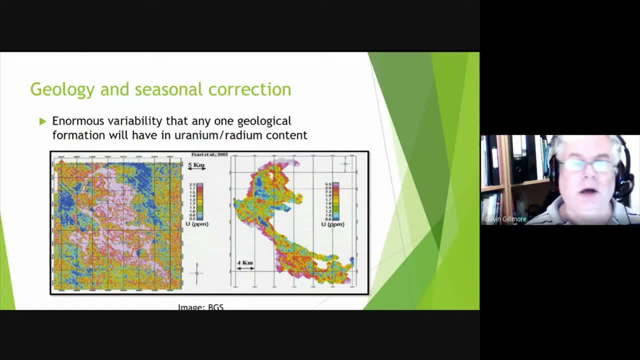 So we know that we see enormous variability from any one geological formation. So this is a BGS map of one particular formation. I think this is the Jurassic mile formation And it shows you. actually this is two different ones showing uranium parts per million And 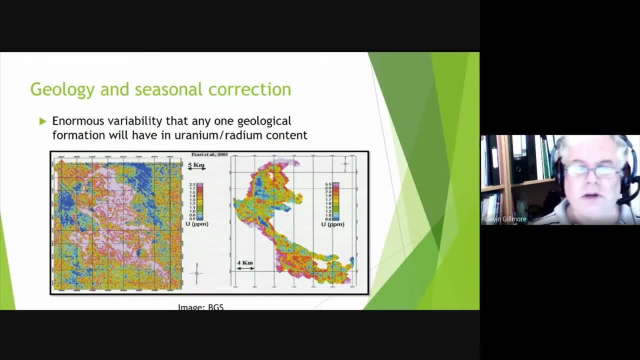 you can see on that one information a huge variation in uranium parts per million over a given area. So of course homes in one part, although you're on the same geology, might well experience very different radon levels within the home. 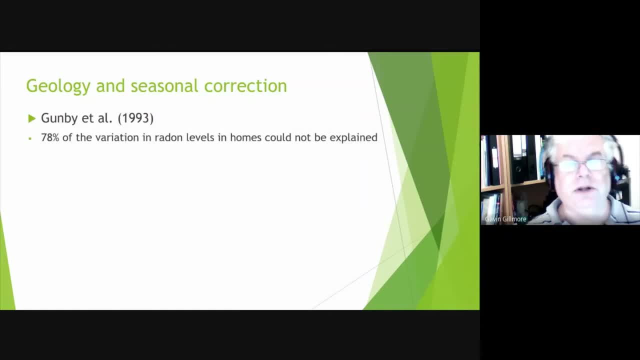 So this causes a bit of a problem when you're looking at seasonal correction and the influence of geology on radon. So Gumby in the late, sorry, early 90s said 78% of variation in radar levels in homes could not be explained. That's not very helpful. 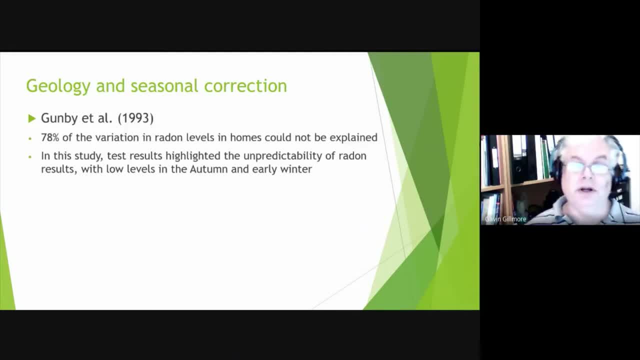 So the test that he did and the test that we did in our study showed that there was radon- could be quite unpredictable. We're giving low levels in the autumn and early winter Now. normally you'd expect high levels in the winter period because you're closing the property up and 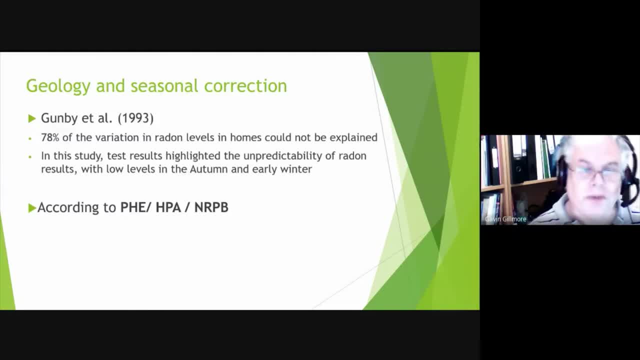 heating the building. So according to Public Health England Health Protection Agency, NRPB, these are the different sort of names for the same body. If relative average radon concentration is taken as one, In July the indoor radon concentration will be a half that of the average value. So in 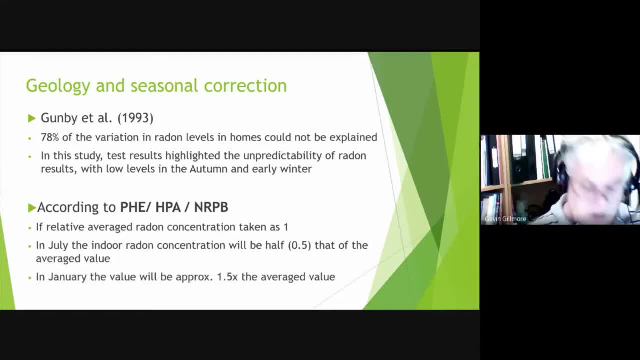 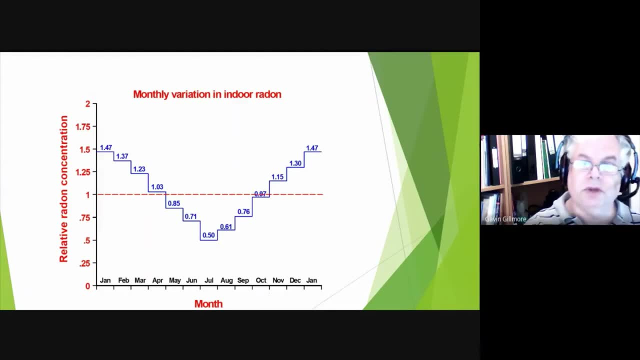 January value will be approximately one and a half times the average. Okay, so, in other words, you'd see this kind of thing. So the idea is that you see monthly variation in indoor radon. so usually in the summer indoor radon is lower than in the winter. Okay, so you want to, if you want to have a sort of 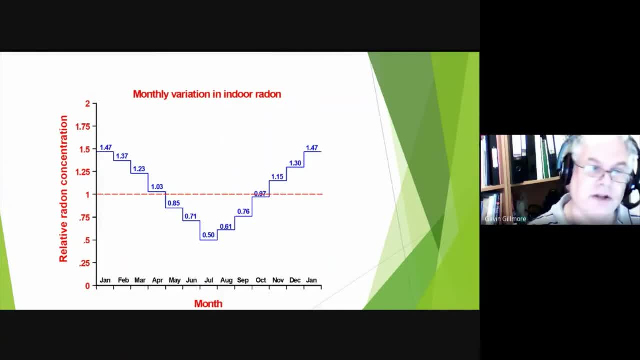 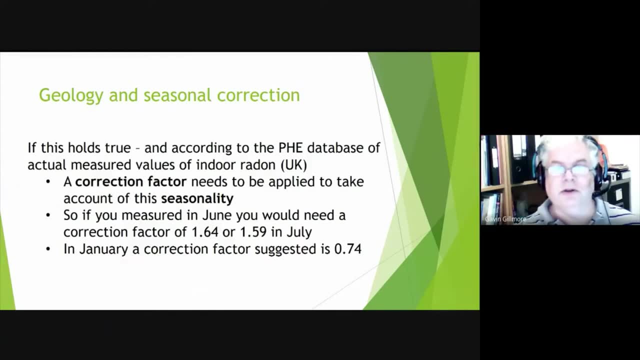 an averaged yearly reading. you want to apply correction factor to get to that. So if this holds true, according to Public Health England databases of actual measured values of indoor radon, a correction factor needs to be applied to take account of seasonality in the data. 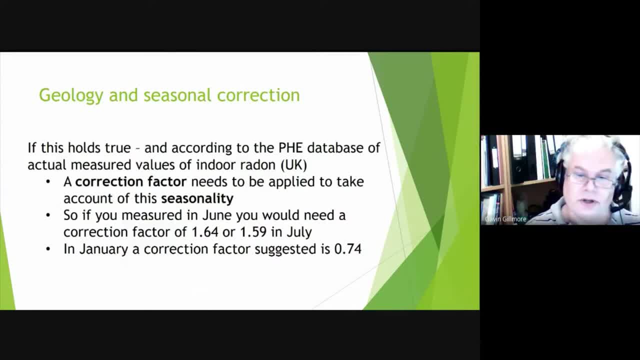 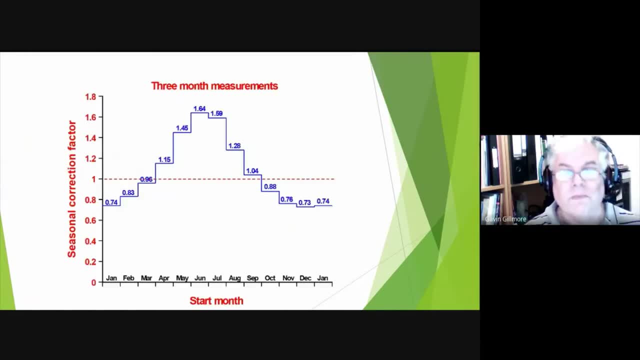 So if you measured in June, you need a correction factor of 1.64 or 1.59. in July and January you'd need a correction factor of 0.74.. Okay, so these are sort of seasonal correction factors that you might need to use. 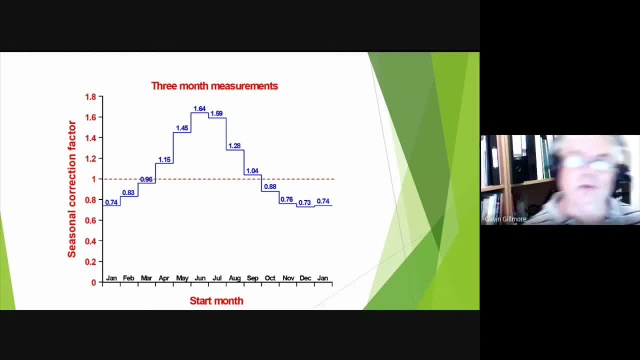 Of course, with the data that we showed in DEFRA, if you applied the correction factors, you could actually then say, well, you should remediate when you didn't need to, or you're in a problem when you do have a problem, Okay. so hence coming back to this. so the potential problem is, as I've just 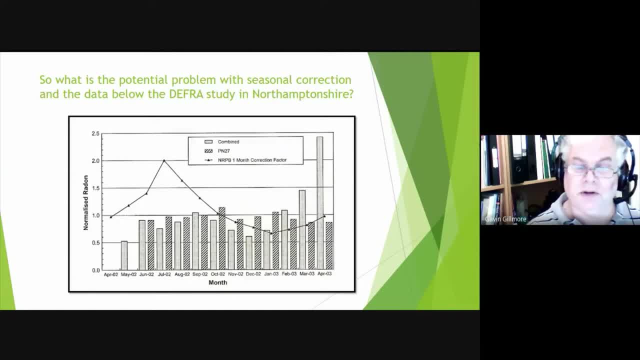 outlined, Okay, so you may be remediating when you don't need to or not taking action when you need to. So this is the problem with a sort of country-wide database. it doesn't necessarily fit in with an individual area. So if you're looking at different regions of the UK, the DEFRA Public Health England looked at having 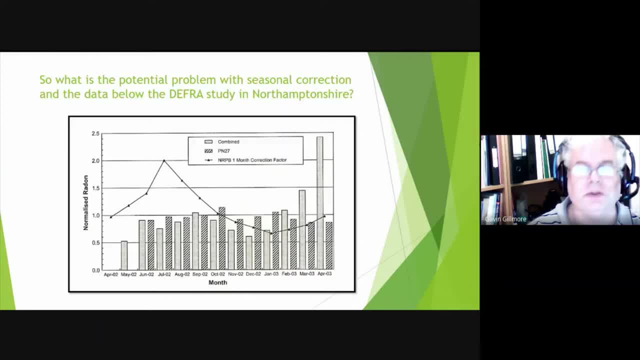 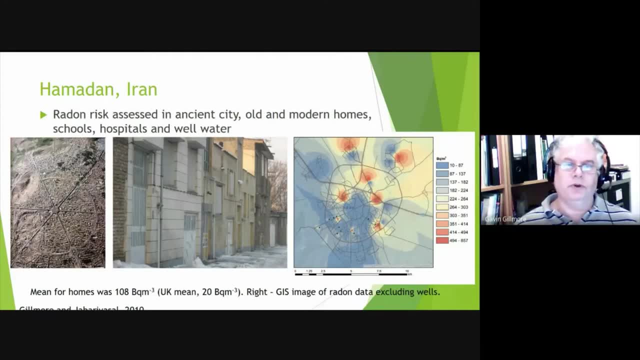 possibly different correction factors for different parts of the UK, then that just confuses the picture. So I said I'd just talk briefly about some work we were doing in Iran. So this is the city of Hamadan, ancient city. So the city was assessed for radon, looking at old buildings and modern buildings. 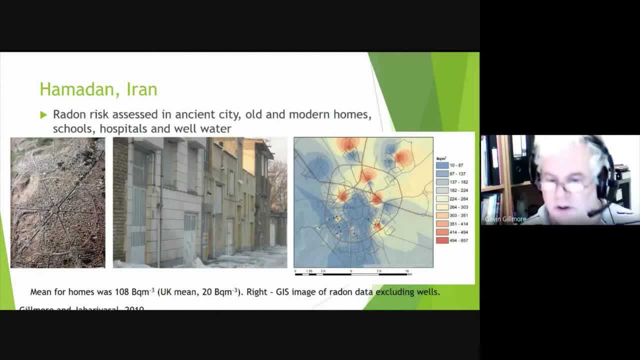 and well waters and also the atmospheric radon in wells. so the mean for homes in hamadan worked out about 108 becquerels per cubic meter. remember the uk mean is 20 becquerels and as we produced this gis image on the right here of radon data, you can see hot spots, basically, and cool spots. 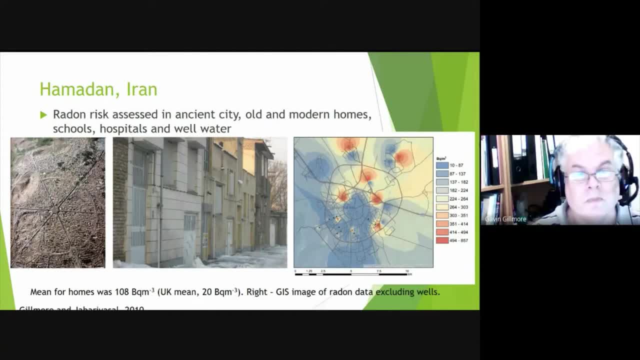 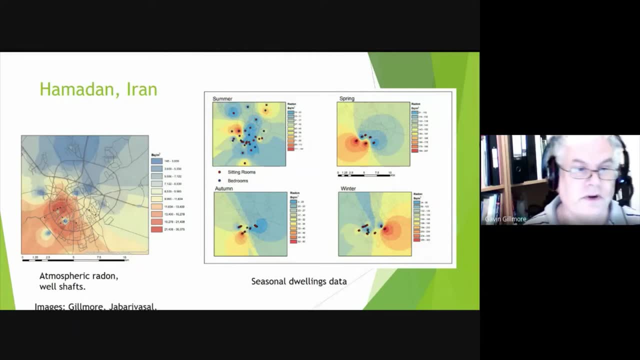 in effect excluding well data, and then we looked at atmospheric well data so you could see actually some of the radon in well shafts could be very high. and then looking at differences between summer, spring, autumn and winter radon distributions and you can see quite distinct seasonal variations. 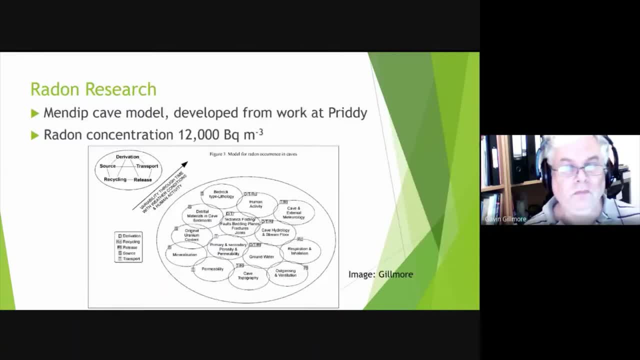 okay. so one of the interests in that particular project was, of course, radon can be transported by water. also, the wells were used for drinking water. you know people, you know, were people drinking radon laden water? or actually the fact that you've got wells, were those wells actually? 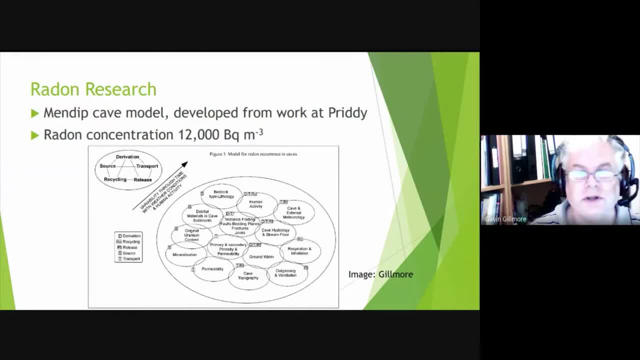 leading to higher radon concentrations in some parts of the city. okay, so trying to understand the way that radon moves around is complex, so we developed the we called the mendip cave model from work we did at pretty caves near bath and we actually looked at the- the radon in these particular caves. there were about 12 000 becquerels per cubic meter. 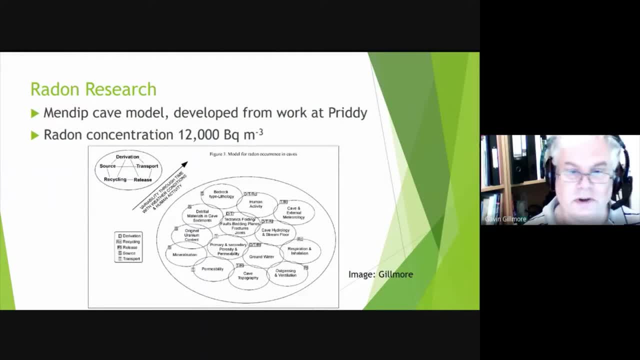 so quite high and you could see the huge variability on controls on the radon in the cave. so you know how much radon was in the groundwater permeability of the material. what was the uranium content of the material? what was the bedrock type in terms of lithology? 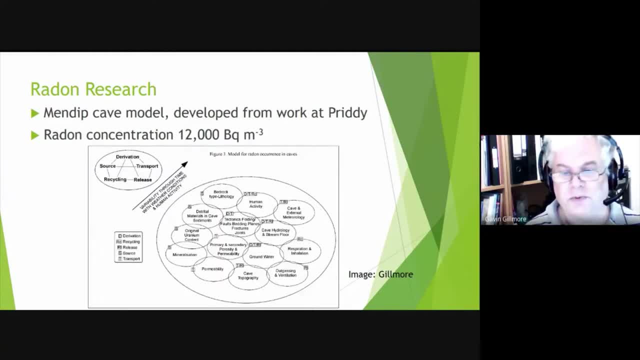 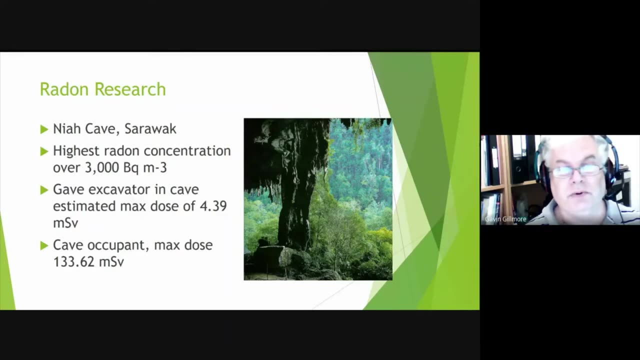 what was the cave hydrology like, how much was being out gassed and what was the ventilation like, etc. so all these factors you need to bear in mind when you're trying to consider particularly radon in caves. so we looked at work in sarawak, for example. uh, here we were actually. 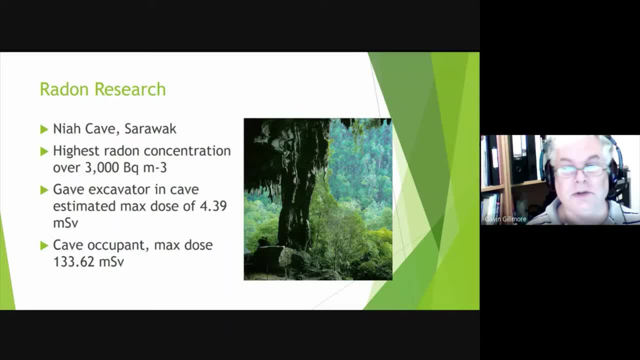 looking at the risk for somebody living in the caves, because people do live in caves out here. highest radon concentration here was about 3 000 becquerels per cubic meter, so a cave excavator. so this was actually an important archaeological site. so a cave excavator was a cave excavator. 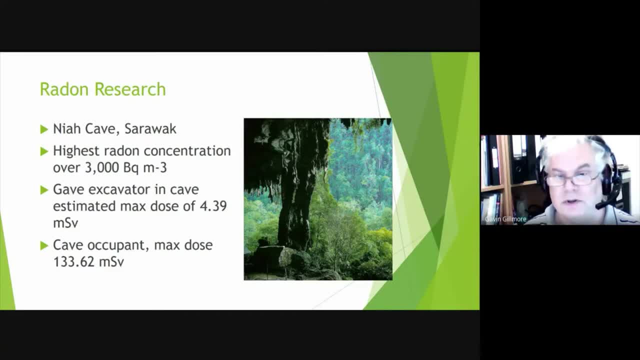 excavator could get a maximum dose of 4.39 millisieverts, which, if you bear in mind, the average dose for a person in the uk is around 2.6 millisieverts. that's a bit on the high side and also the recommendation is that you shouldn't get more than one millisieverts above that 2.6. 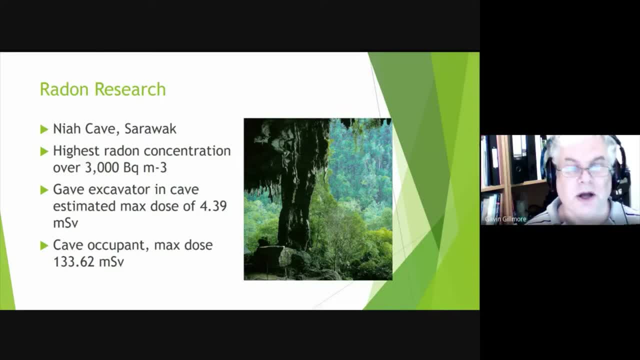 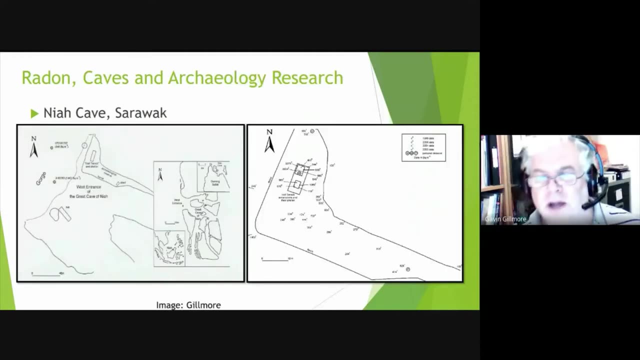 millisievert dose as a member of the public. a cave occupant could get a maximum dose of 133 millisieverts, so perhaps living in caves isn't such a good idea. so this just shows you some of the distribution of some of the data, and the highest data was in. 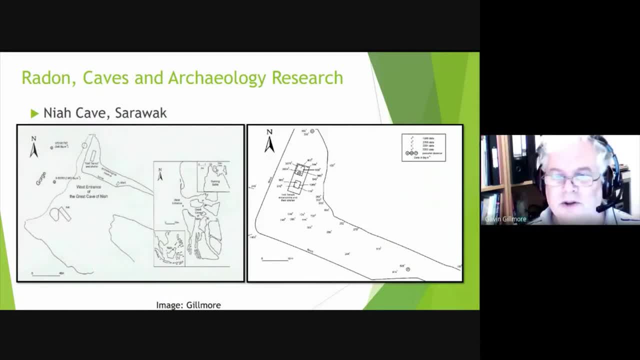 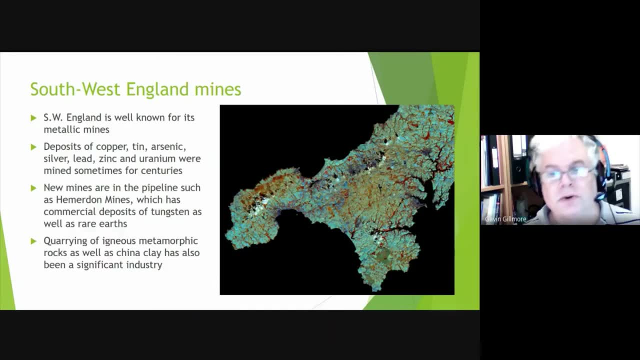 what they called hell pit, which was around a thousand becquerels per cubic meter, or hell trench actually. um, uh, yeah. so we also looked at radon in mines in the uk, so x metallic mines, so deposits of copper, tin, arsenic etc. and uranium have been mined for in southwest england. 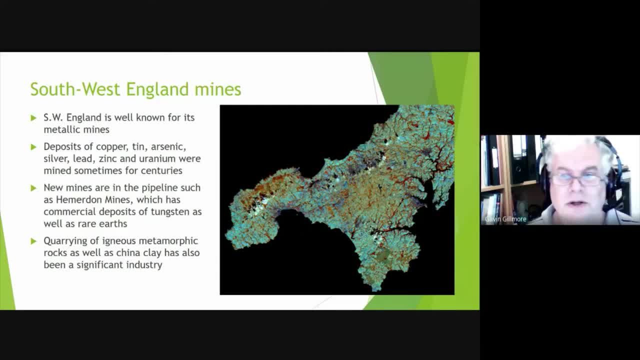 it's like there are new mines in the pipeline, such as hammered and mine which is looking at um exploiting tungsten as well as rare earths, and also, of course, they've quarried metamorphic igneous rocks etc. in the region for many, many years. so we measured in. 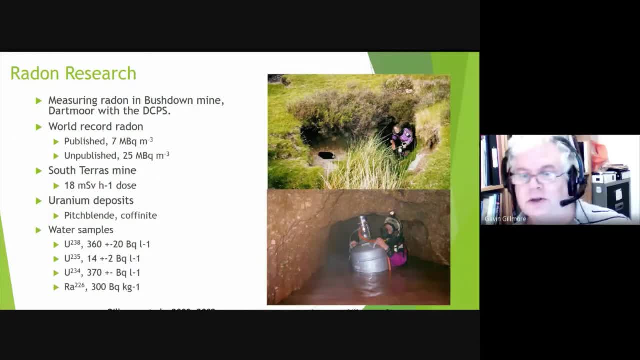 different mines. so, bushdown, mine was on dartmoor, on granites, and you can actually see in the lower picture the the large uh feldspar crystals of the granites um, and we recorded world record radon levels and we published seven mega becquerels, seven million becquerels per cubic meter. 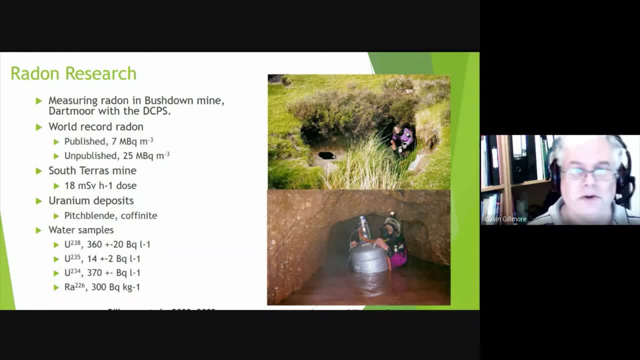 um. we've also discovered 25 million becquerels. we haven't published that number, though one of the mines- south terrace mine was actually mined for uranium at one point- contains pitchblende and coffinite, and we measured 18 millisieverts per hour dose. so bear in mind. 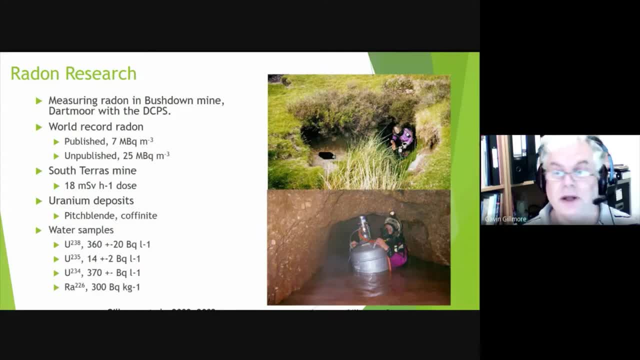 what i was saying. one millisievert per hour is a maximum for a member of the public and also, incidentally, you could get 200 millisieverts per hour, which is about 200 millisieverts per hour to 200,000 becquerels per cubic metre, just standing outside the mine entrance. 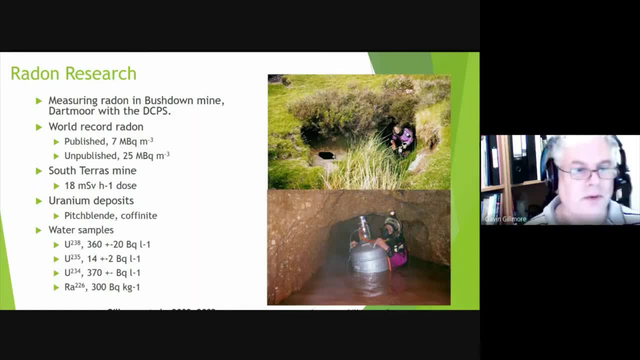 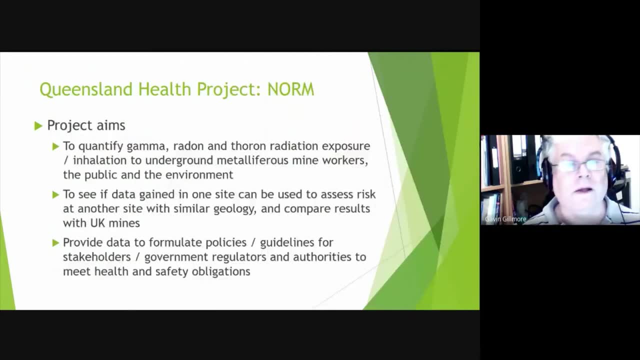 So we looked also at water content and said, well, what's in the water here? Well, uranium-238, 235, 234 and radium-226.. So this led us on later to a project with Clewinsland Health, looking at what's called. 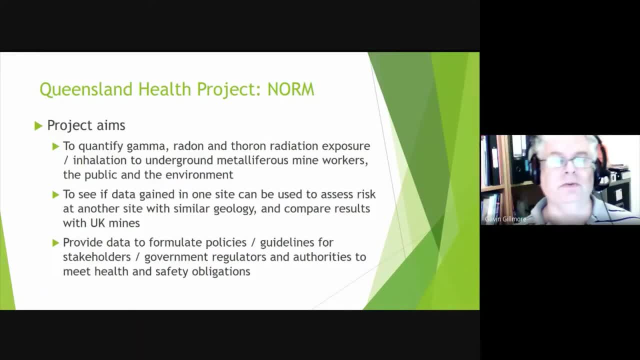 NORM Naturally Occurring Radioactive Materials and the idea was to quantify gamma, radon and thoron radiation to metalliferous mine workers to see also if data gained in one site could be used at another site with similar geology and compare the Australian results. 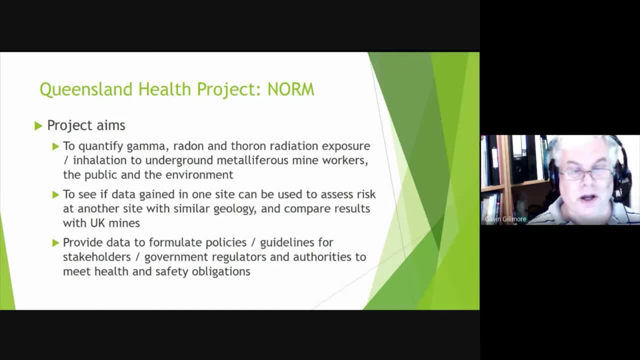 Clewinsland Health with UK mines that we've just been talking about, And the idea was to provide you know policies and for regulators, et cetera, and make sure we met health and safety. So it was with a company called Wolfram Kemp Mining and Queensland Health and they were 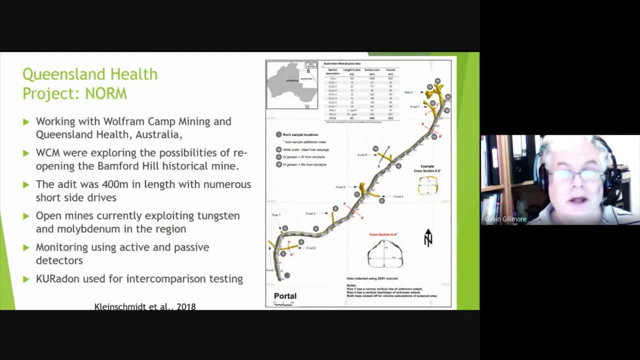 exploring possibilities of reopening Bamford Hill mine And they had. it was something like 400 metres in length, lots of little short drives off from it, And they are currently exploiting the area for tungsten and molybdenum as to be put in. 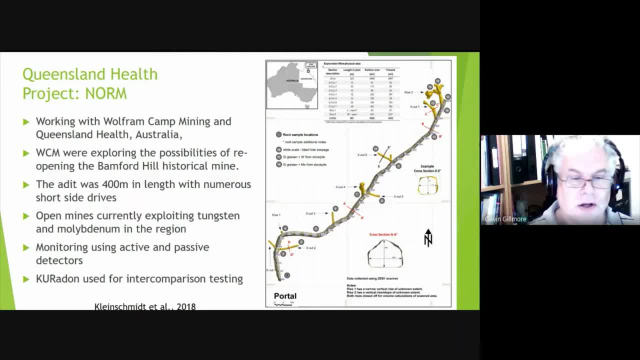 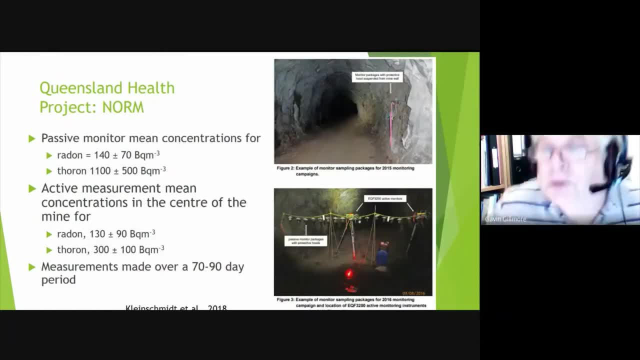 active and passive detectors And we used KU Radon for interpretation And we used KU Radon for comparison testing with different detector types. So you can see the mine itself on the right here showing you the monitoring campaigns And in the centre of the mine you can see we strung up some string, basically, and attached. 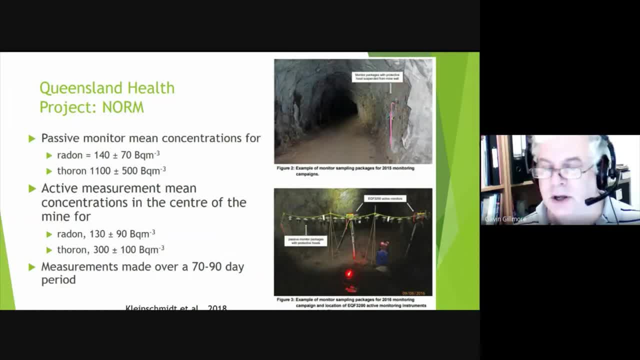 detectors across that- passive detectors in this case- And the idea was to actually see what the variation was across the airspace. So we measured radon around 140 becquerels. But we also measured radiation across the airspace, So we measured radon around 140 becquerels. 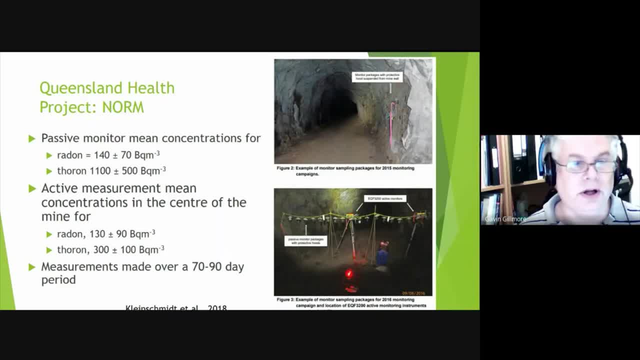 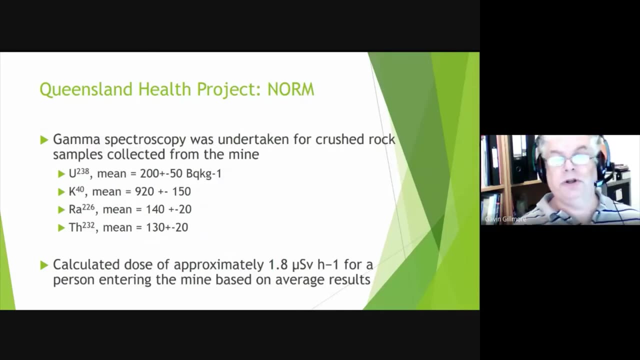 But quite a lot of error margin in that Thoron was relatively high And the centre of the mine radon was around 130, thoron around 300. And we measured this over a 70 to 90 day period. We also did gamma spectroscopy of crushed rock samples. 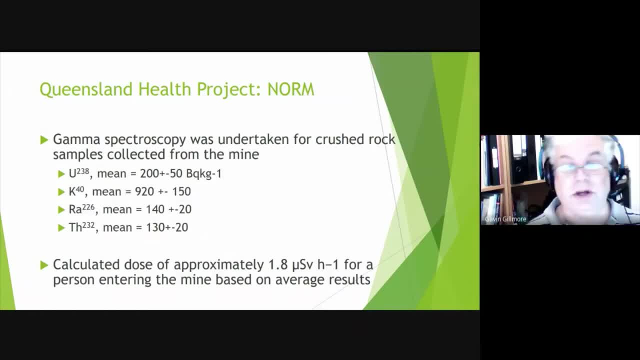 And we were able to show that there was uranium in the rocks, potassium 40,, uranium 226, and a thorium 232.. And the calculated dose of approximately 1.8 microsieverts per hour for a person entering the mine. 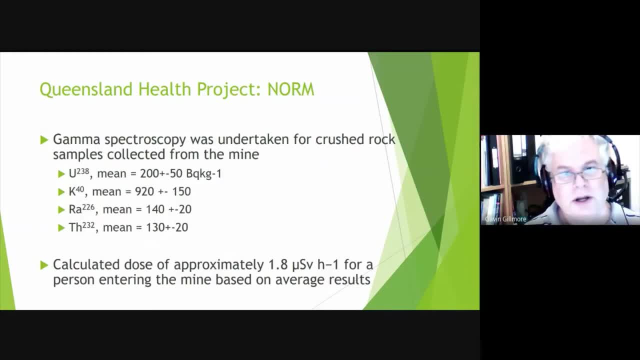 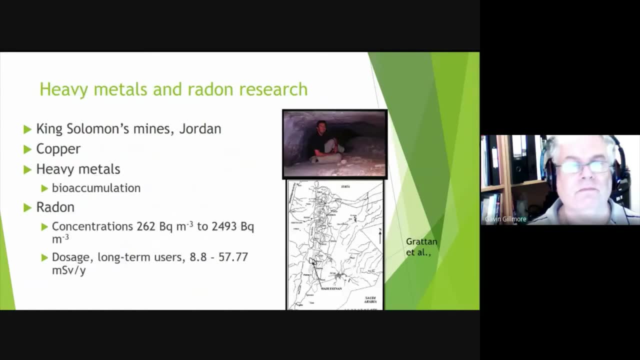 Bear in mind that the mine in South Terrace mine we were looking at 18 millisieverts per hour, An order of magnitude different. So we then looked also at mines in Jordan that had been heavily exploited for copper. So one of my colleagues, John Gratton, at the top here, 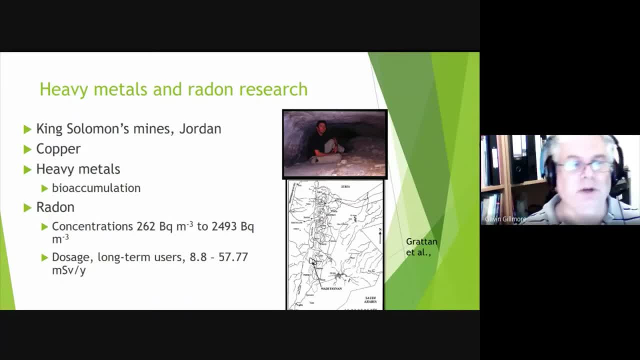 He was looking at mines that were still there. heavy metals- Bioreaccumulation- that we were looking at as well- And radon concentrations varied a lot, from 262 up to about 2500 becquerels per cubic metre And you could see long term uses- those people who exploited the mines for copper workers. 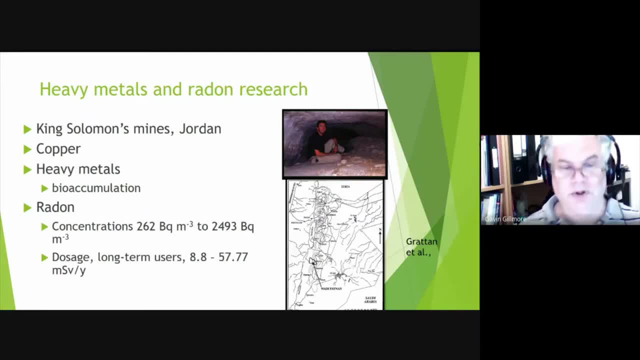 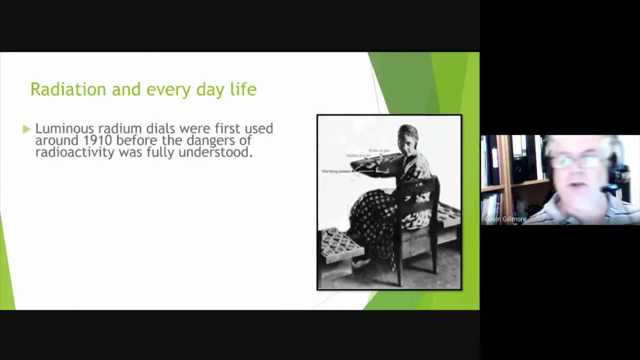 in the mines, basically in Wadi Fanin, would get between 8.8 and 57 millisieverts per year life. Sorry, I'm trying to sort of wrap this up a bit more. So we're exposed to radiation in everyday life. I don't know. 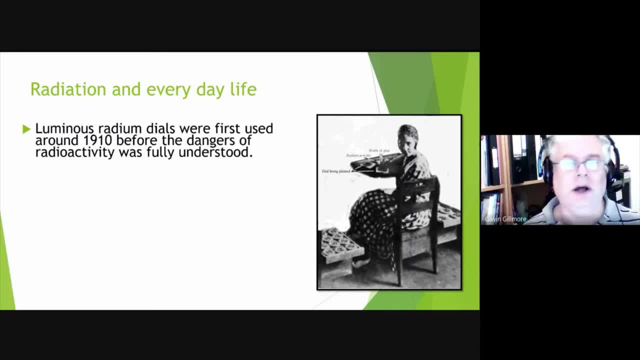 whether you've got an old pocket watch or an old clock. But up until the 1960s, radium powder tended to be mixed with paint to paint the dials with in order to make them luminous. So the idea here is that there's a zinc sulfide material in in the 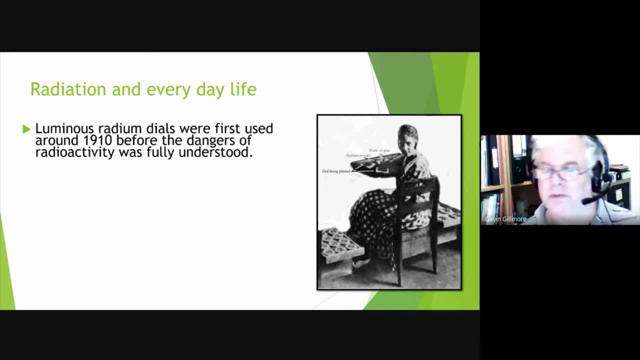 paints And, as the radium sends off alpha particles, hits the zinc sulfide and causes it to fluoresce. Okay, very useful if you're in the dark and you want to see the time. But you can see the lady here. she's got a bottle of glue. she's got 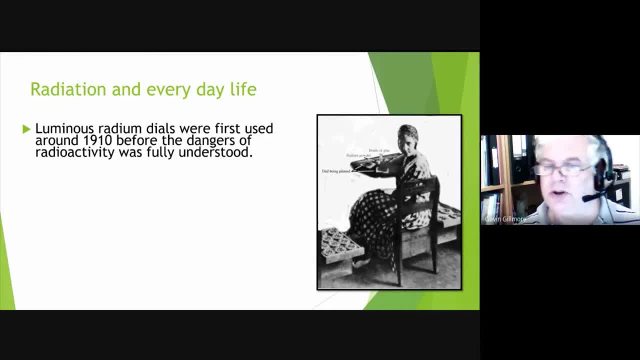 radium powder, and then she's dipping a brush into the radium powder and then dipping it into the glue, or the other way around, and then brushing onto the dial, which doesn't sound too bad until you know the way she got a point was to basically lick the. 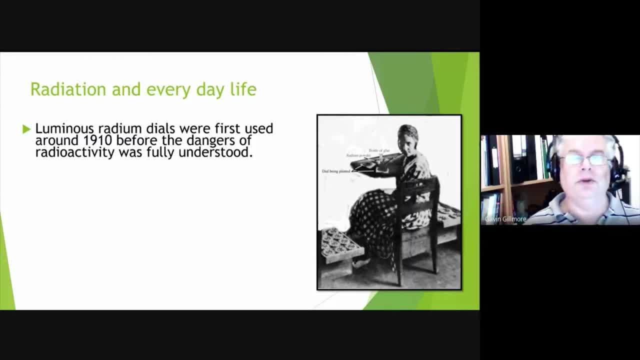 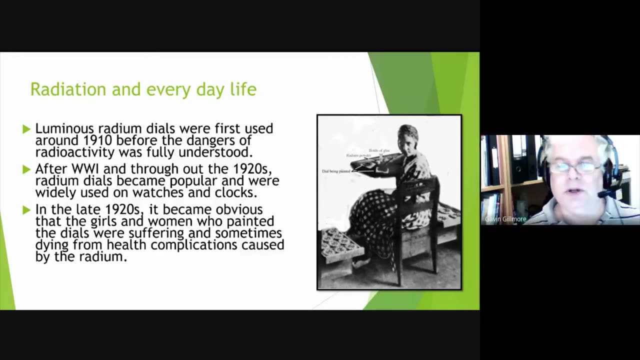 the end of the brush. So luminous radium dials, first used around 1910.. After World War One and throughout the 1920s they were very popular, widely used, widely used on watches and clocks. 1920s became obvious that girls and women who were 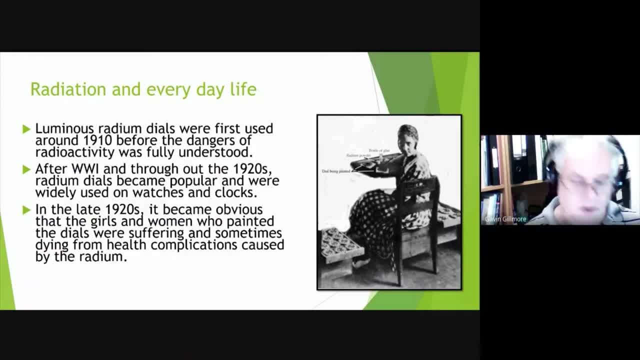 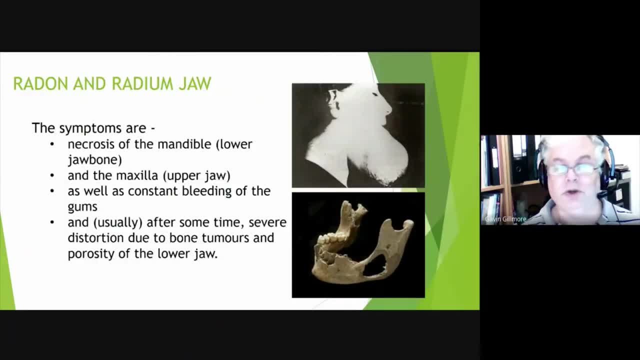 employed in this kind of work were suffering, sometimes dying, from health complications caused by radium. So these slightly unpleasant images, this is called radium jaw. Okay, so this is as a result of ingestion of radium. Remember, radium is the precursor for radon. Okay. 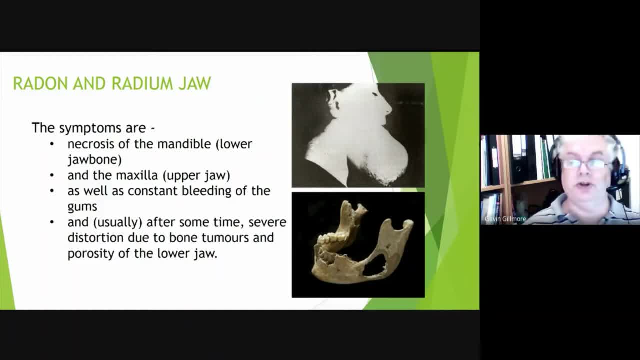 so actually these people were not only exposed to or ingested radium to two six, they also exposed to radium 222.. So this led to the necrosis of the mandible, the lower jaw bone. you can see the lower jaw bone here with a great big hole in. 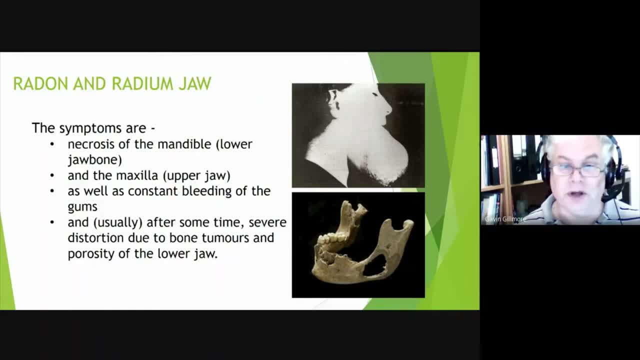 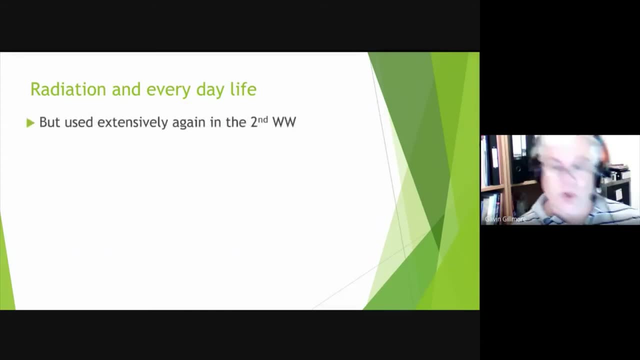 it fell out: constant bleeding of the gums, severe distortion due to bone tumours, porosity of the lower jaw, and there were also very high incidences of things like breast cancer. So come Second World War, we used the material again. Well, okay, so why did we do that? Well, 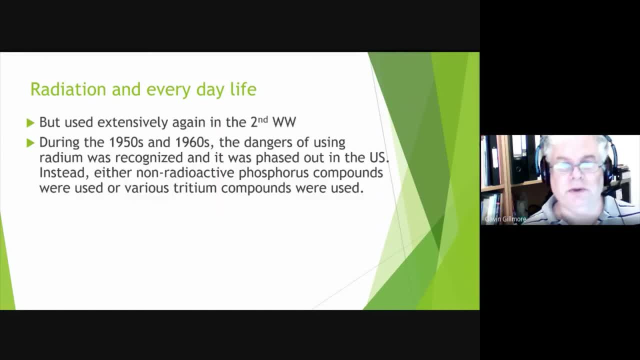 I think they deemed it was safer to see the time than to pop your head above the trench at the wrong time and be shot. So during the 50s and 60s danger of using radium was recognised and it was phased out and they now use either non-radioactive materials or some tritium compounds which are 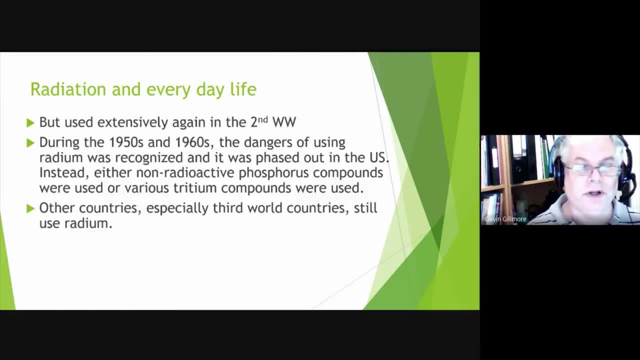 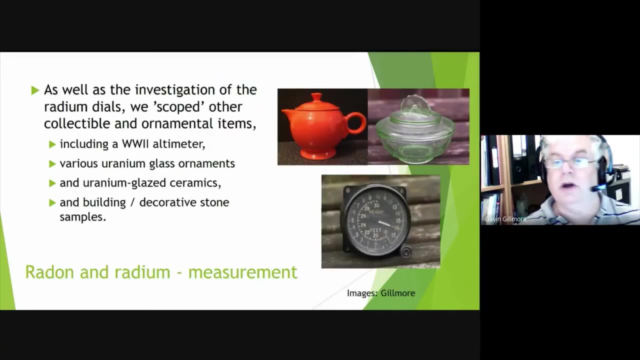 also radioactive, but not for so long. It tends to be a beta emitter rather than an alpha emitter. So other countries, especially Third World countries, still use radium, and during the Gulf War the Iraqi tanks, for example, had radium dials. So there are other items that you might find out there still. So we did some work looking at radon. 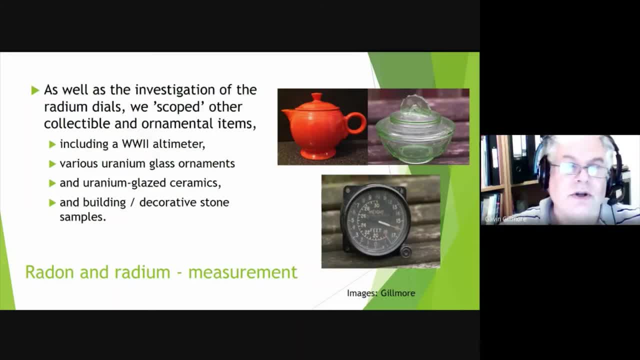 and radium measurements in some of these items. So we collected materials. So here you can see a teapot which is uranium glazed. You can see uranium glass and then you can see an altimeter from a Spitfire of the Second World War and the sort of orangey coloured paint that you can see. 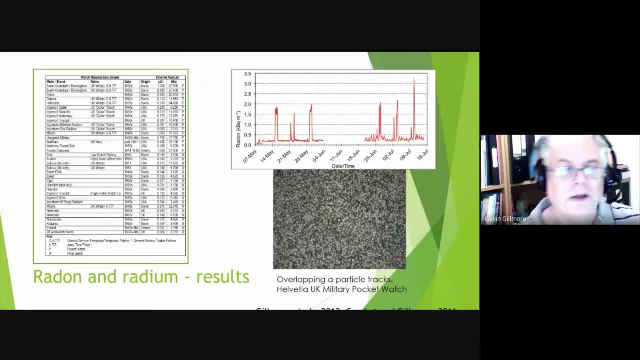 here is radium paint. So we collected watches and some of these items. put them together into a collection. measured the uranium content, put them all together in a room and this is what we got. So you can see radon being generated in quite significant amounts around 2000. 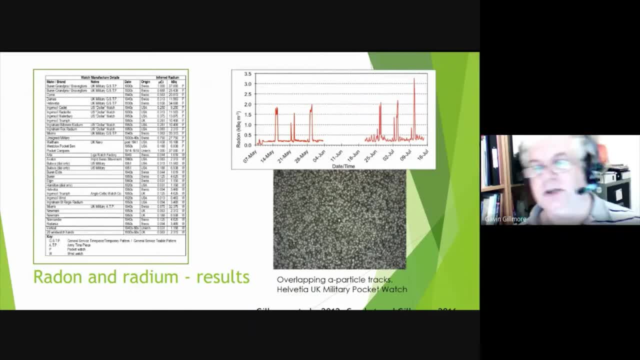 peaking up to around 3000 becquerels. Notice the peaks and troughs and this. basically, this was in a lab. so this is when the air conditioning was switched on and switched off. Okay, so when the air condition was switched off at night, then the radon levels peaked. 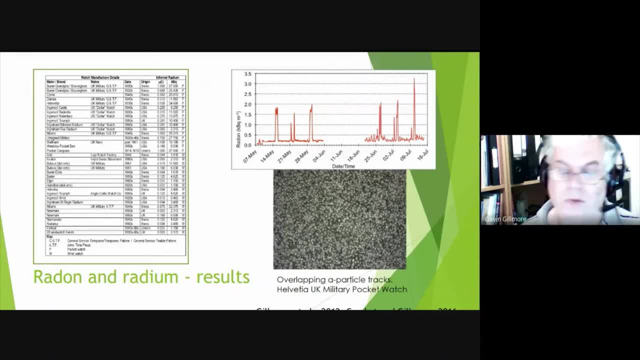 And then this is an alpha track. well, this is a SSNTD which has been exposed to one watch and you can see basically the track. the SSNTD has been obliterated with tracks. so there's: the watch is so radioactive So this was reported in the national press at the time. so this is the mail online, but it appeared. 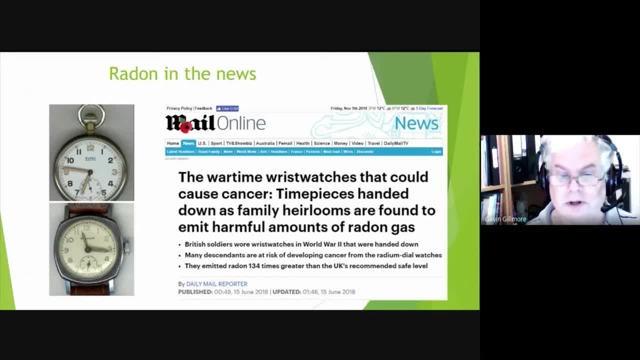 in quite a few, I think Times Telegraph and various other ones as well. So these are a picture of some of the watches saying wartime- wristwatches that could cause cancer. timepieces handed down as family heirlooms are found to emit harmful amounts of radon gas. So they emitted radon 134 times. 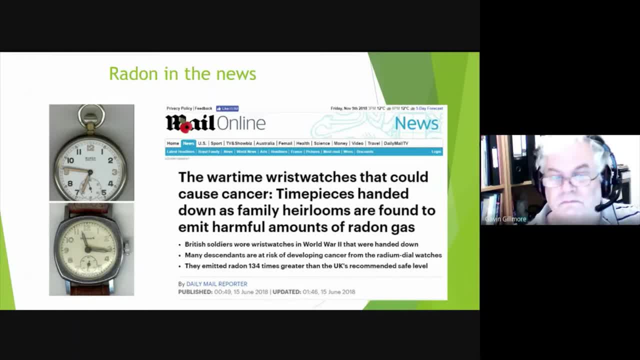 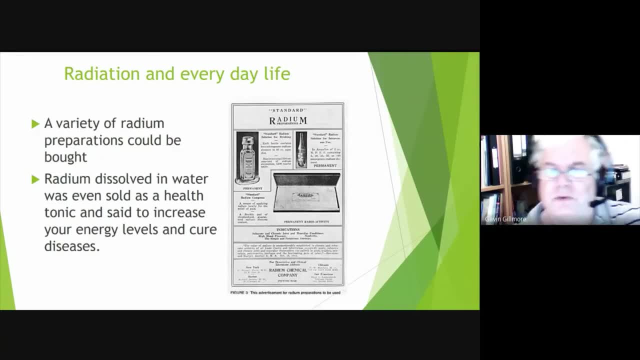 greater than the UK's recommended safe level. So, believe it or not, radium was actually used in all sorts of different things before we fully understood the risks. So here we've got an advert for radium solution for drinking, standard radium solution for intravenous use, a radium compress, and, believe it or not, they. 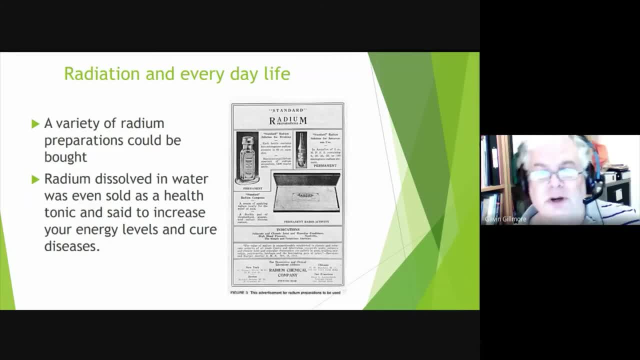 also had things like radium suppositories, Because radium was being used by Marie Curie to treat cancers. therefore the idea was then: this must be good for you. So the idea was sold as a health tonic to increase your energy levels. So I said: 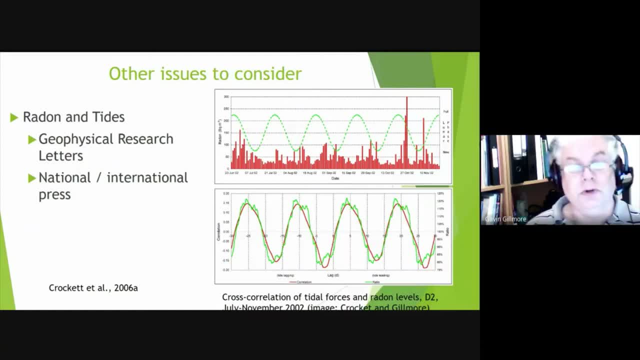 actually radium can be used as a useful tool. So together with a colleague of mine at Northampton University, we worked on radon and tides and published some work in geophysical research letters- And this also hit the national and international press at the time- And two images. 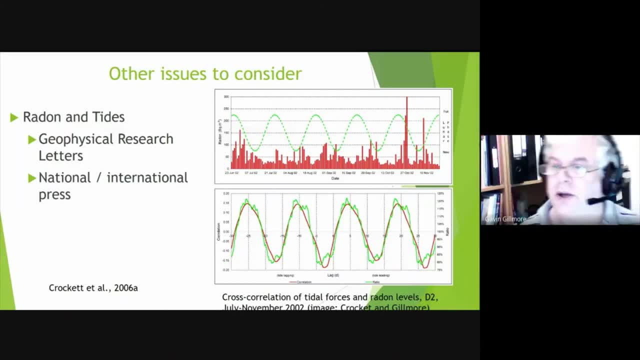 here show a correlation between radon and lunar phase. So this is part of the data was gained, partly as a result of DEFRA work that we were doing, And we were able to demonstrate that there did seem to be a cyclicity in the radon data. 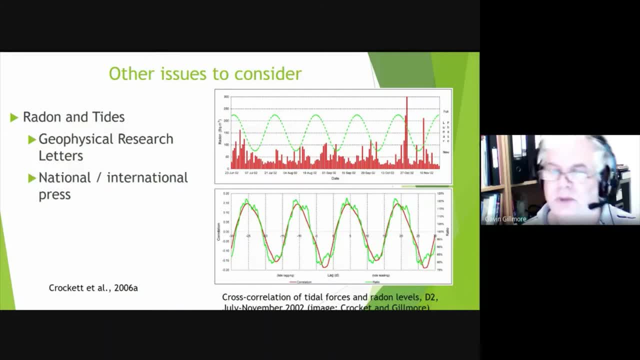 And if you took out things like weather changes and weather patterns, you could actually link tides or the lunar phases to radon peaks and troughs. And when you think about it, it's not that surprising in a way, because if you think of earth tides and ocean tides, as the ocean tide comes in, 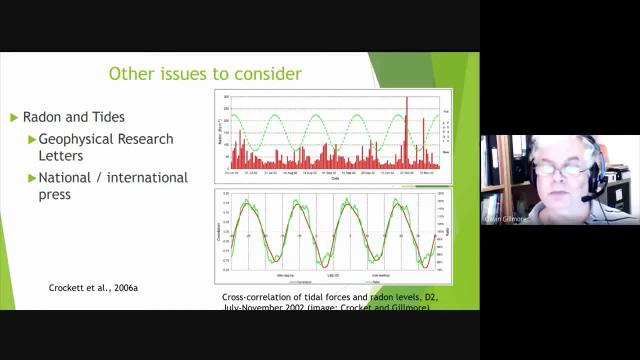 it presses on the crust might open pores up and as it goes out the crust can relax So you have a pumping action for any gasses within pores within the rock. So this led us to also look at other sort of anomalies in the data that we had. 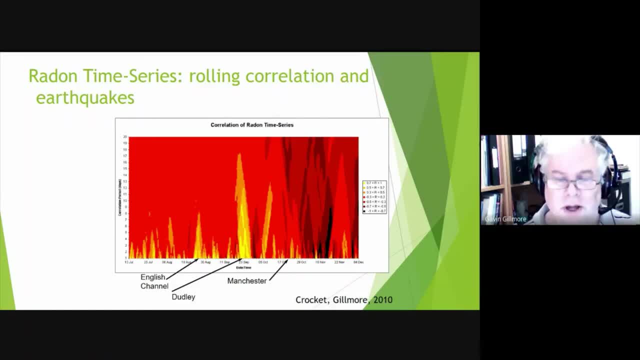 And this was actually a What's called time series analysis, looking at earthquakes, And we're able to show that there appeared to be a correlation: earthquake peaks or earthquake activity and radon peaks. now this is a highly controversial thing. in some ways, people have recognized this pattern before, but 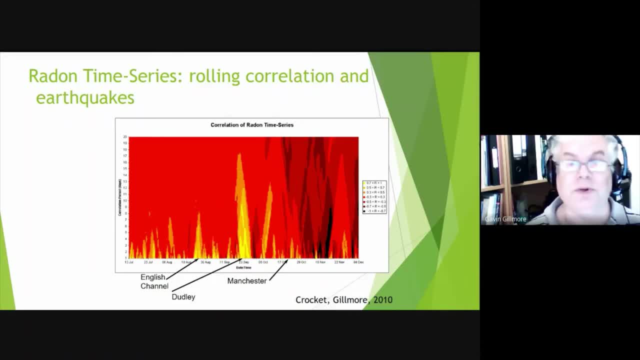 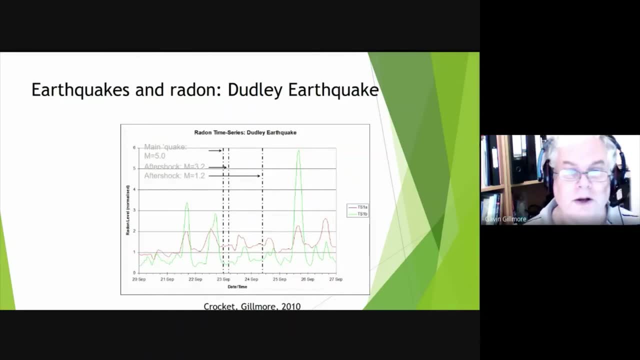 only retrospectively. some people have said: well, perhaps we can use this predict earthquakes, maybe maybe not. so this is the Dudley earthquake and you can see the green and the red lines are two real-time radon detectors that we had out measuring at the time and you can quite clearly see peaks in both set. 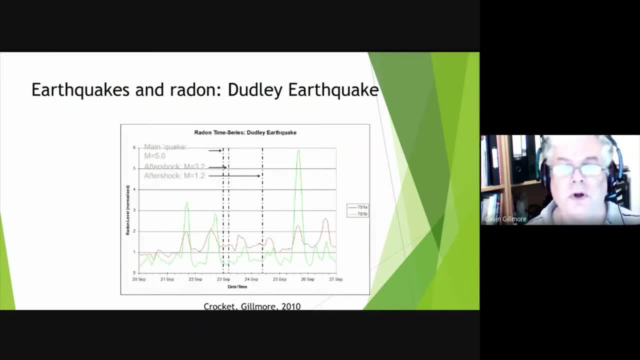 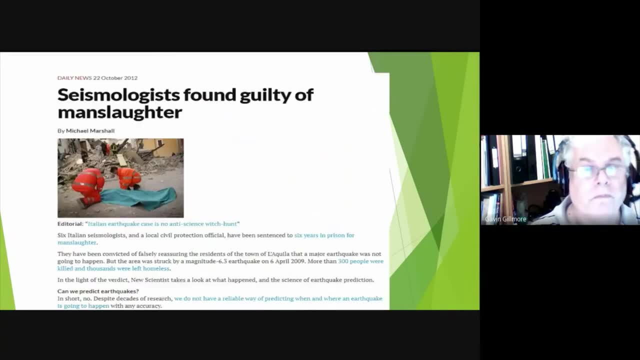 data sets and how these are correlating to just before the main quake and also associated with the aftershock. of course, this does bring up an interesting story: seismologists found guilty of manslaughter. so this was a- um uh- italian situation, where six italian seismologists were sentenced to six. 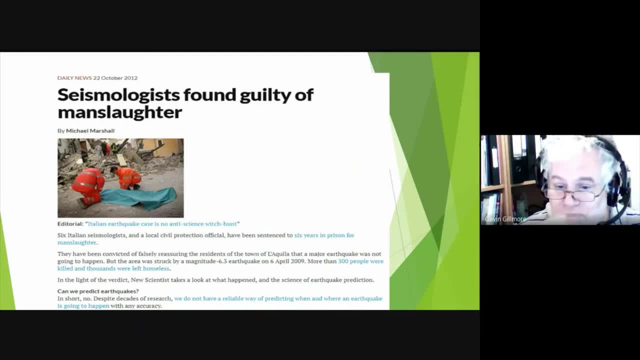 years in prison for manslaughter. um, if you want to know a bit more about this case, it's um, associated with somebody who had a lab. um was measuring radon and then said: well, we're going to have a big earthquake. the earthquake happened and, of course, people at time were saying: 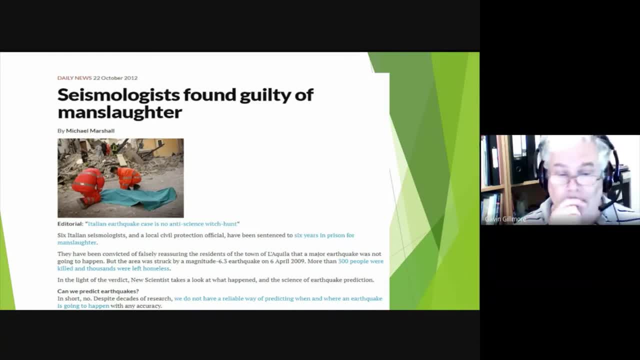 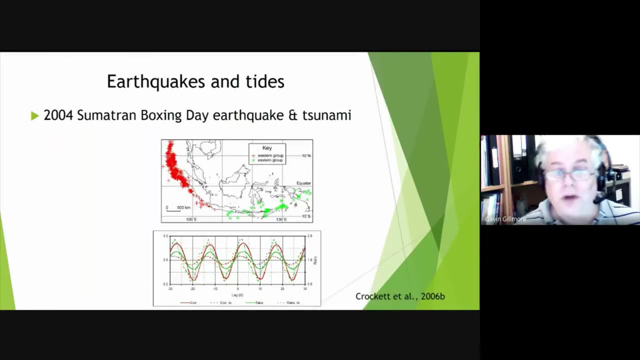 we're not going to have an earthquake. it's a lot more complicated than that the story, but i recommend um reading up about it. it's fascinating um. they have since been acquitted, by the way, so we said, well, okay, um can we look at um things like the boxing day earthquake? 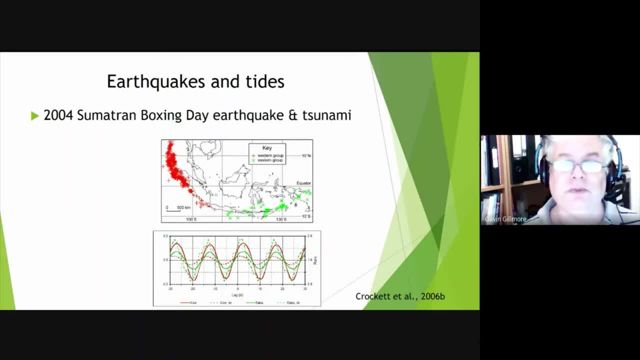 does that? you know, is there a tide and effect with um earthquakes? so there seems to be a tide effect with radon and we were able to show actually fact um, there did appear to be a link between the 2004 samaritan boxing day earthquake and the boxing day earthquake and the boxing day. 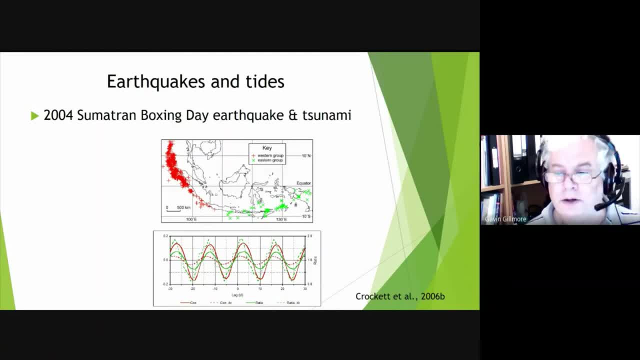 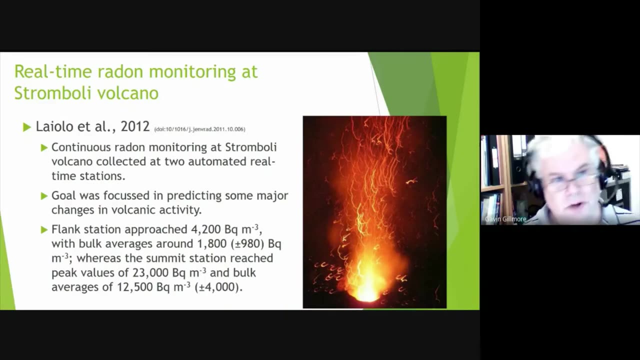 earthquakes and tsunamis again. if you look at the croquet hotel paper 2006, you can read a bit more detail about that and how that worked. so radon um has been used and is being used as part of a suite of measures to look at earthquake activity. 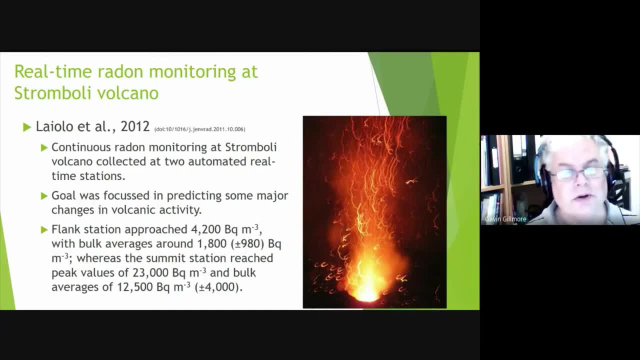 another thing that people are doing and have done is to look at volcanic activity. so here we've got, um um. Iolo 2012 has actually looked at real-time radar monitoring of Stromboli volcano in order to try and predict to some extent what's actually happening with the volcanic activity. So the 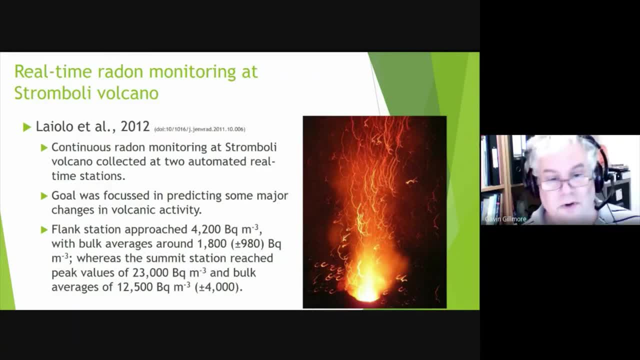 goal was focused on predicting major changes of volcanic activity. So the flank station approached 4,200 becquerels- bulk averages around 1,800 becquerels- whereas the summit station reached peak values of 23,000 becquerels. Okay, so there's clearly a lot of radon being. 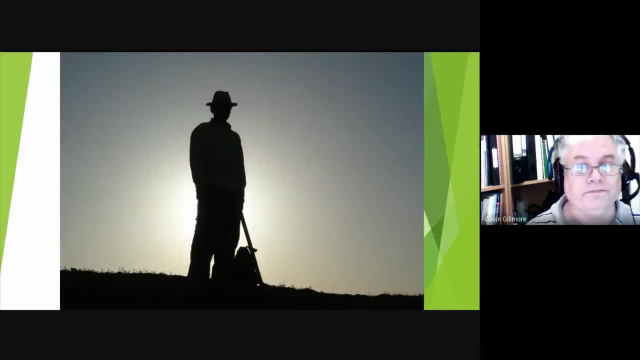 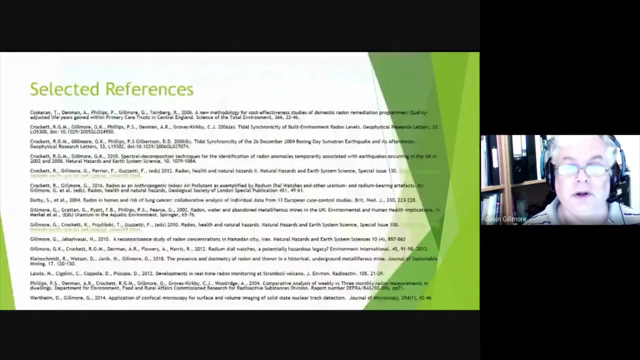 pushed out of the volcanoes. Okay, so that's the end of my talk. Sorry, it's been a little bit longer than anticipated. This is a picture of me, believe it or not, a few years back on fieldwork in Iran, taken by one of my colleagues, And then this is just a selection of references. 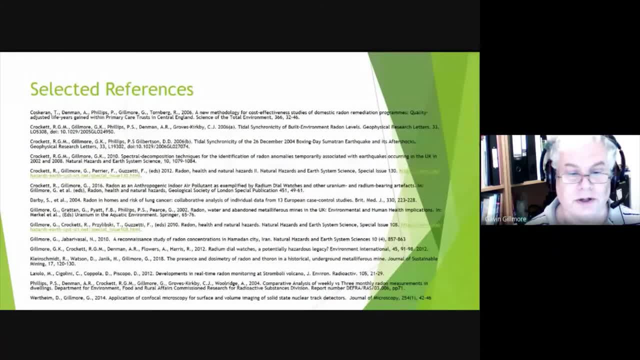 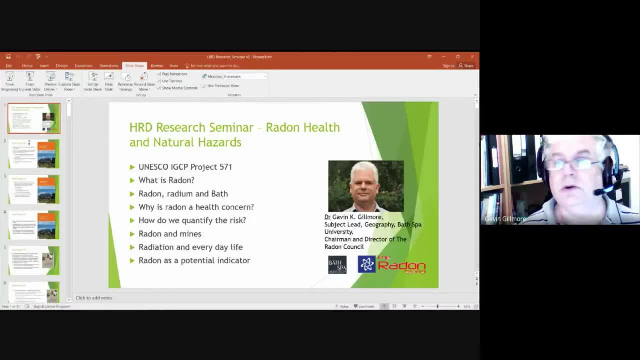 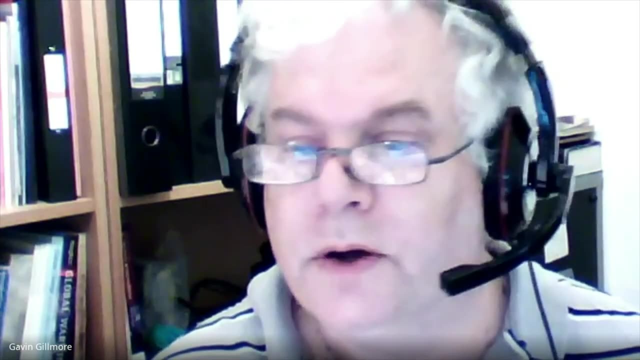 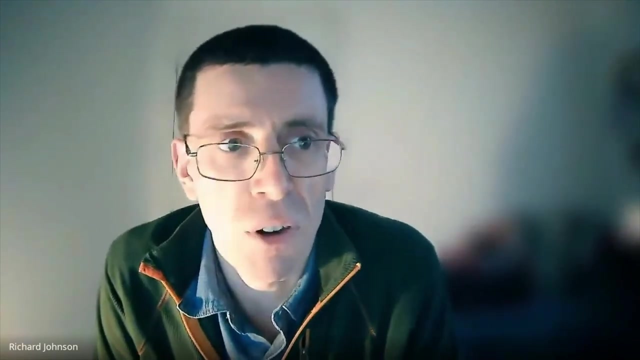 references referring to the papers that I've been talking about and some of the research work we've been doing. Okay, so that is the end of my talk. I will close my PowerPoint and stop sharing. Okay, Sincere thanks, Gavin. This is Rich here again. That's, you know, a really insightful. 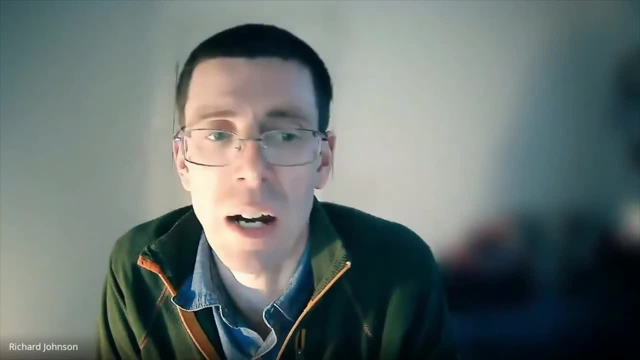 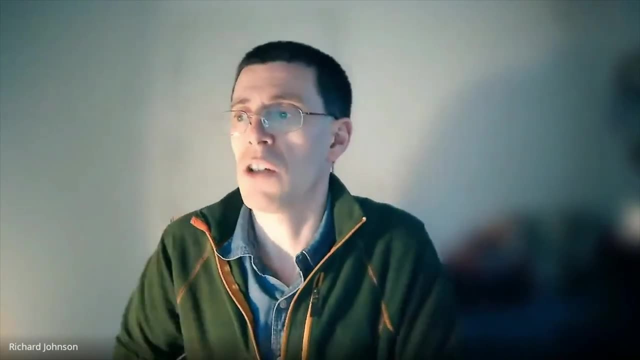 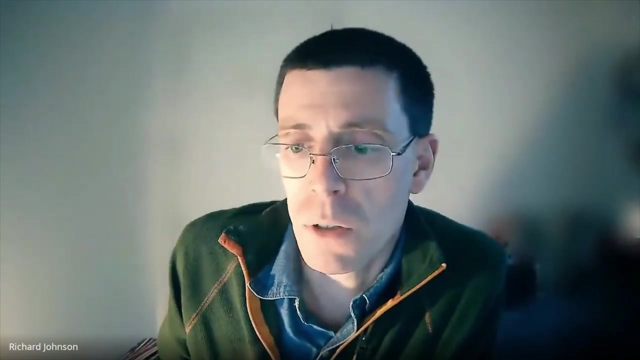 and broad and deep discussion of this issue. I think we can clearly see that we need to take note as a society, not just in the UK but globally, And there's a real challenge here. So there's a real impact behind this work. But I obviously now want to open up this afternoon to sort of 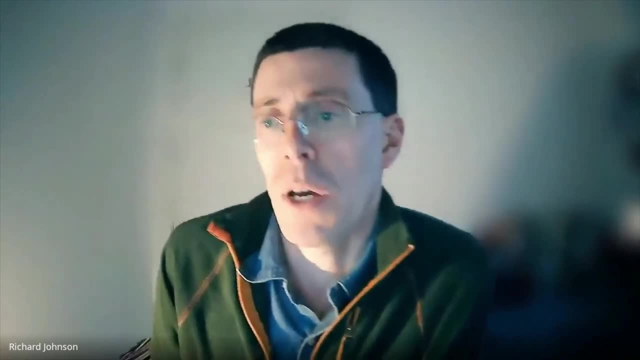 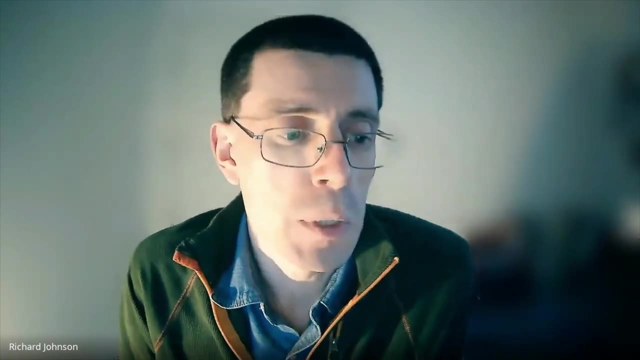 a question and answer session. So if people do have questions, could I invite them to type them in the Q&A section And we'll certainly have a look at those. Be aware, if you were to turn on your microphone and your video, you'll be part of the recording. So if you wish to remain anonymous. 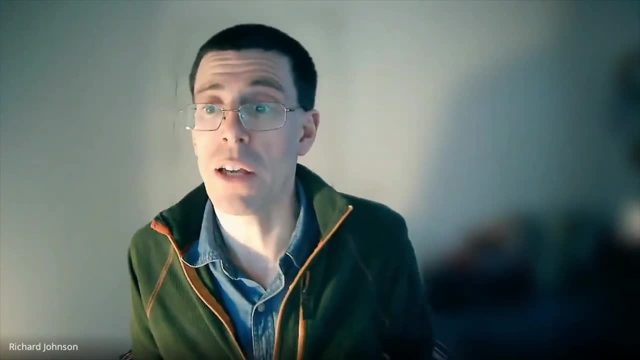 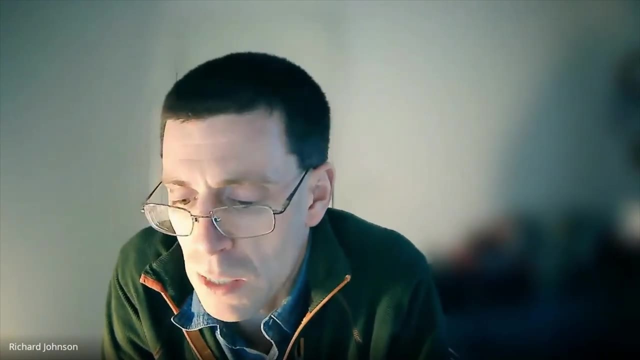 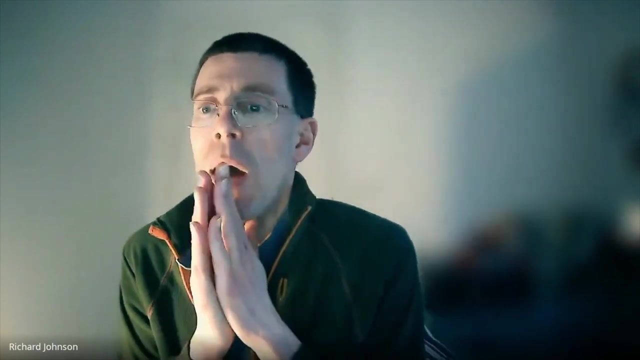 please use the Q&A, And so I'll start things off. And it actually relates to some of your final slides, Gavin, and that's how we assess radon hazards in association with other environmental processes, And I sort of jotted in my questions and I think I can perhaps merge them together. 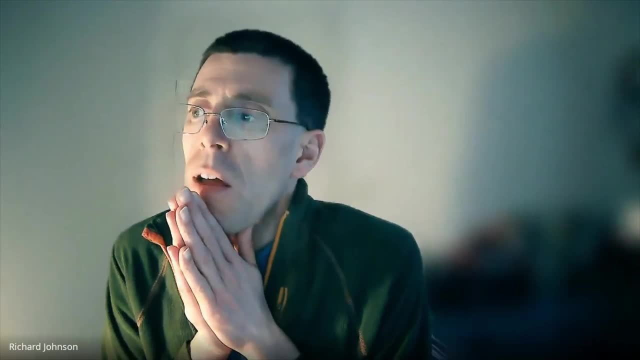 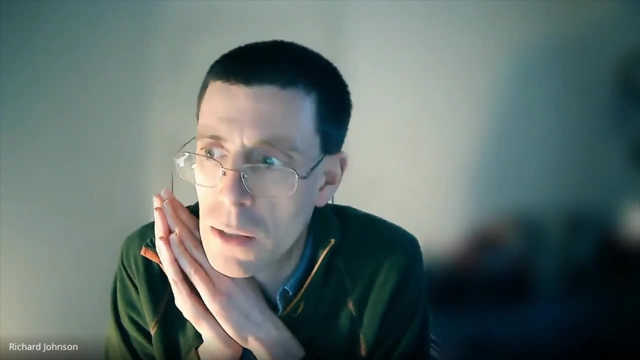 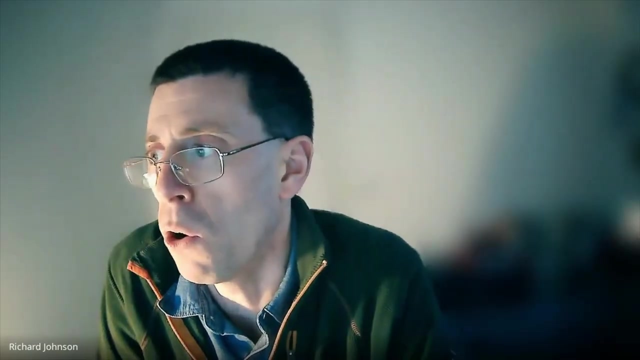 And it's just one chain of thought I have, And that is: how do radon emissions, or how could they change in time in the context of environmental variability, so forth? Example: cryospheric melting with climate change in variability or flood episodes. 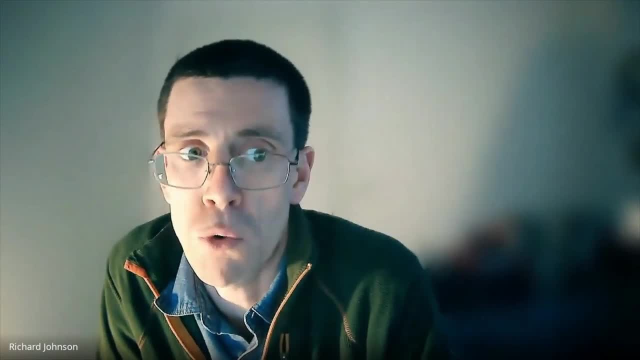 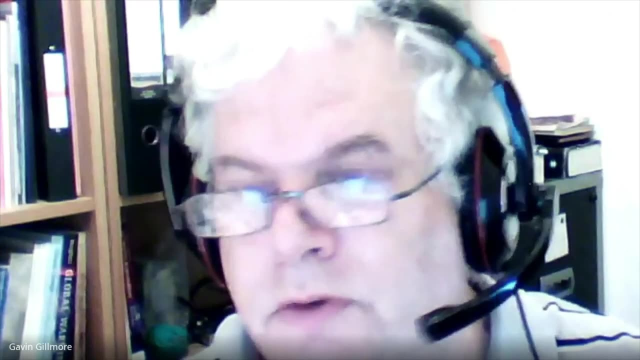 Is there a need to look at these cascading hazards and put radon in that chain? Simple answer is yes Because, if you think about it, radon relies on permeability of the soil, So anything that's changing the permeability of the soil. 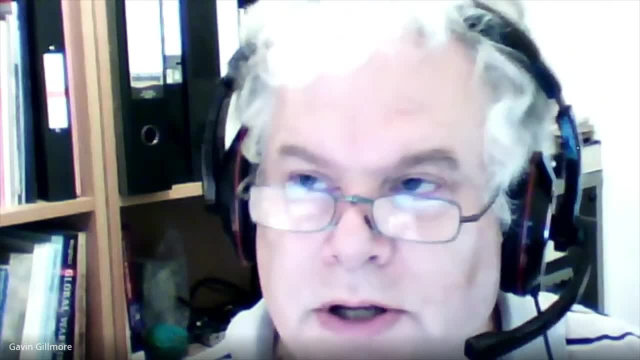 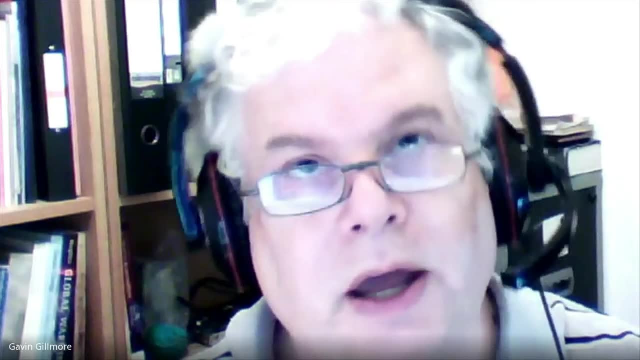 So, for example, you have clay soils. Normally clay soil will act as a good barrier for radon, But if then you have a very dry episode and clay soil cracks, then there are pathways then for gas to escape through that barrier. 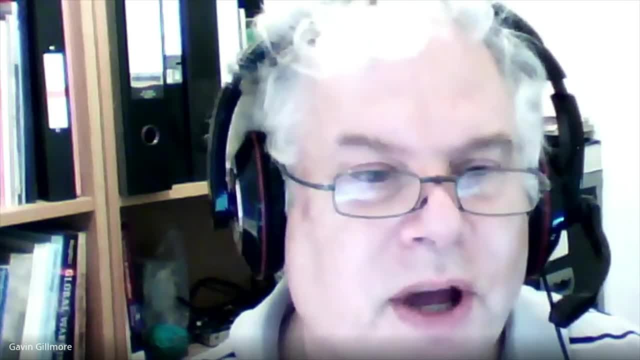 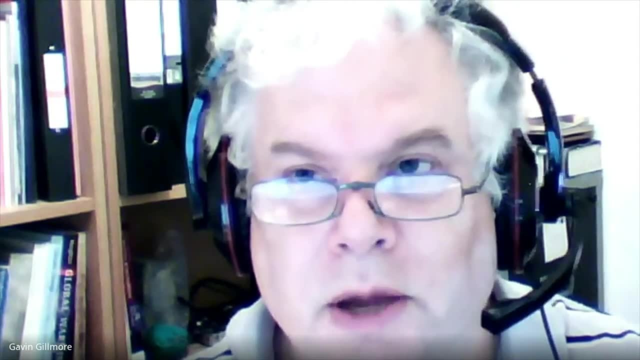 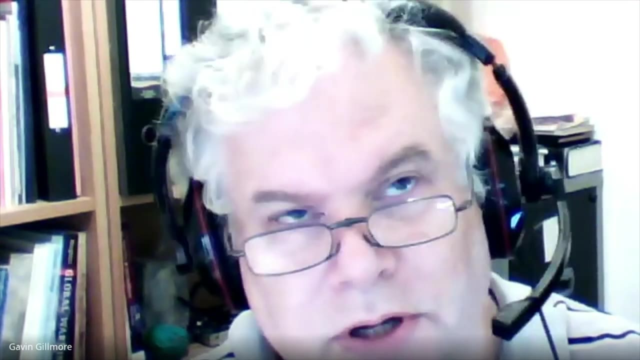 Similarly, if it's water laden, then of course, then that might act as a good barrier and stop radon from passing through it. It's certainly true to say we're seeing changes in radon level that we previously haven't seen, So let's rephrase that: 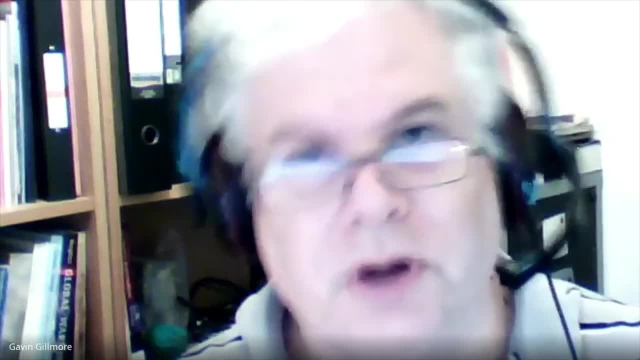 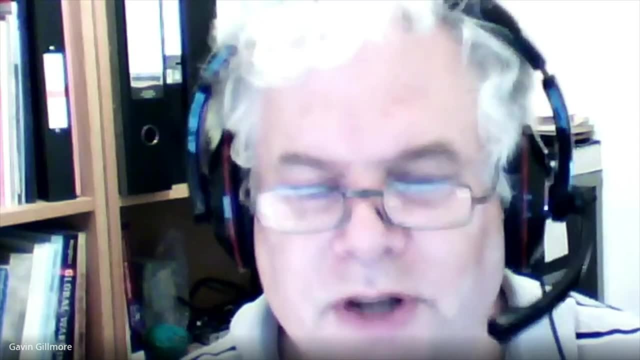 So normally we'd sort of measure a building and say, well, it does or it doesn't have a radon problem. Problem is with climate change. you can't take that black and white view anymore, because next year and the year after and the year after. 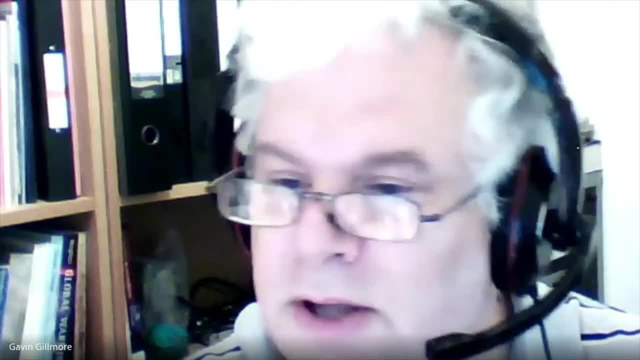 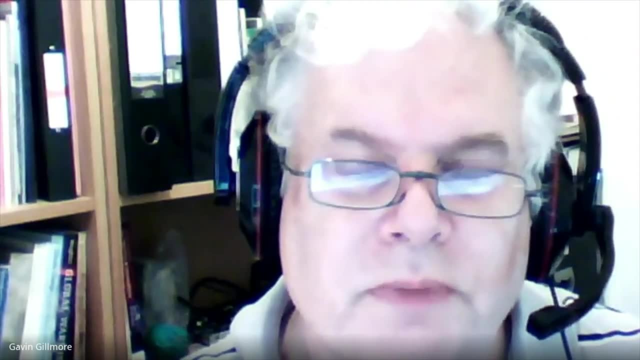 radon levels may be very, very different because of changing ground conditions. So climate change, I think, is having potentially a big impact, Also what we're doing to buildings. we're saying, well, we should make buildings more environmentally friendly. 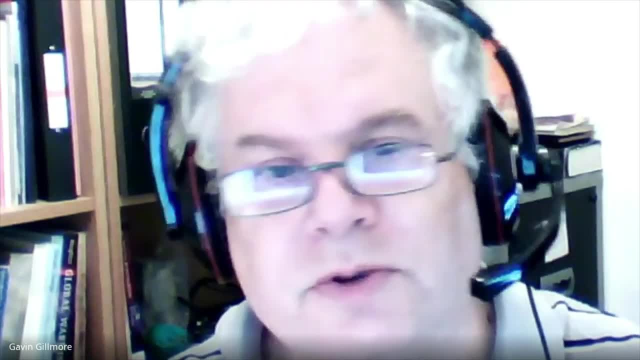 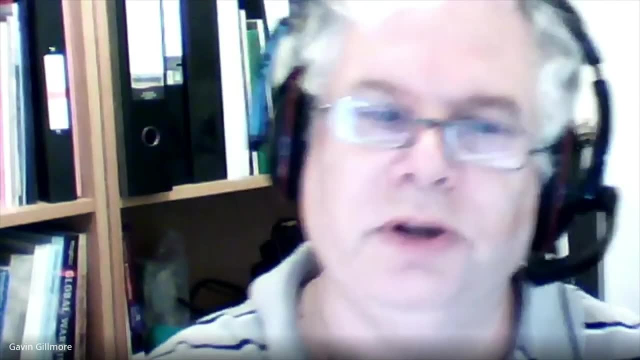 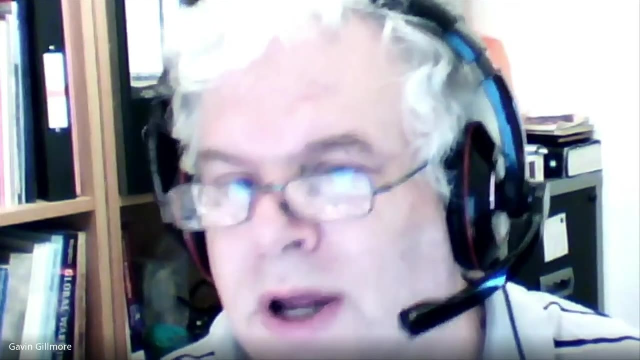 and therefore less air exchanges per hour. But of course then that traps air within the building and therefore means you could be concentrating radon gas. So I know that's sort of built environment as opposed to natural world. But yeah, I do think that if we're getting more cascading hazards. so another good example is one: 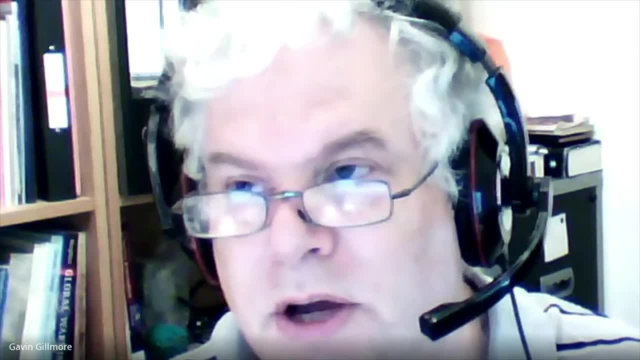 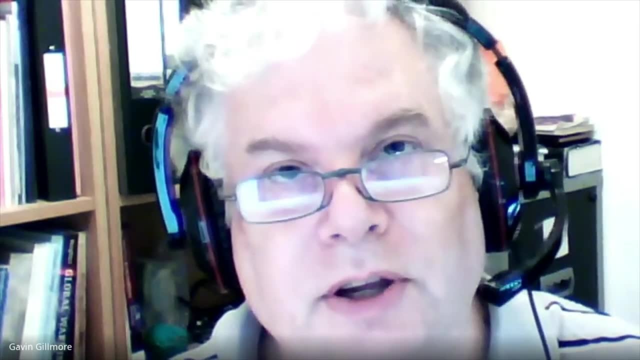 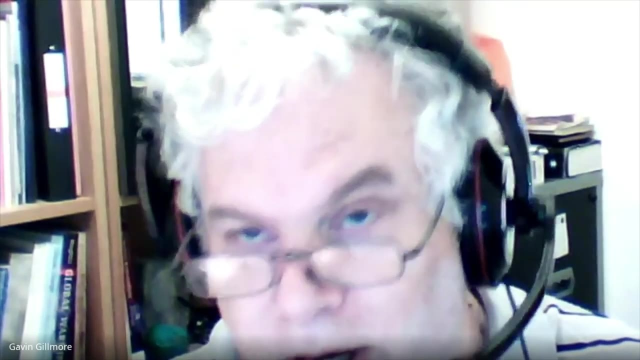 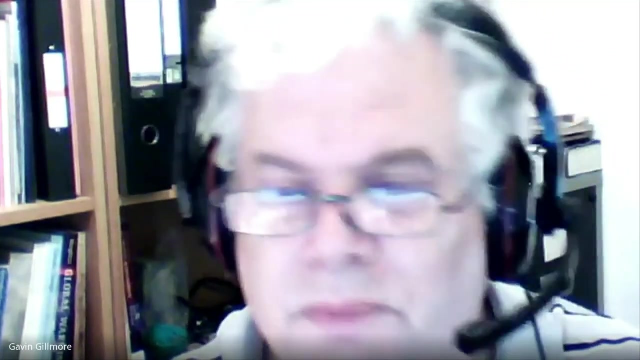 suggestion that with melting ice caps we may see a release of pressure on volcanoes and therefore more eruptions, And if what people have said is true about radon and volcanic eruptions, then it may well be that we see more radon being exhaled as a result of increased volcanic activity. 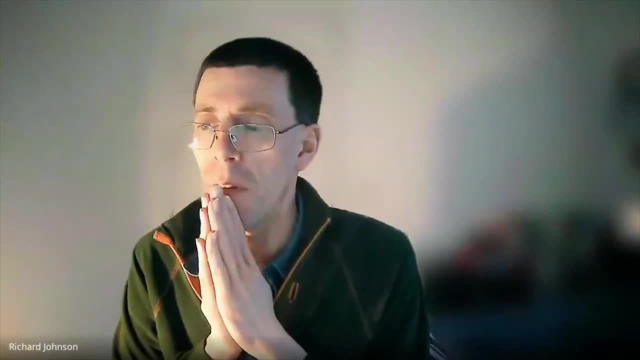 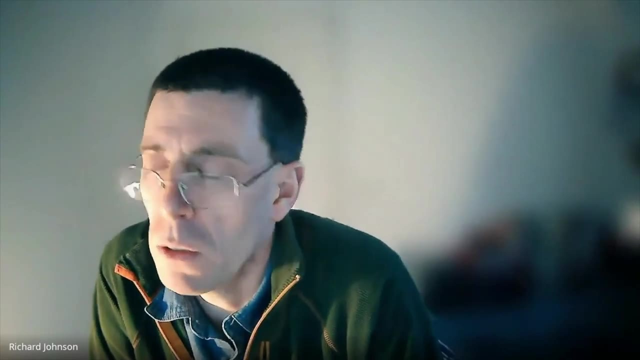 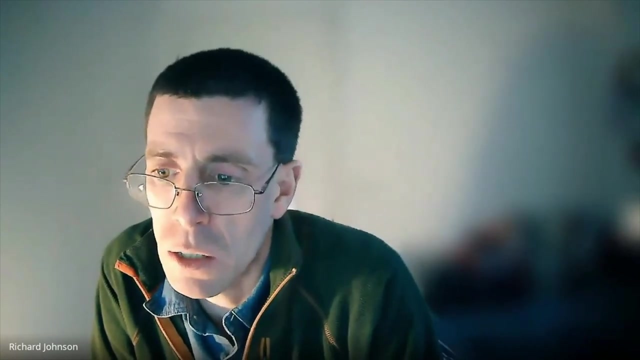 Thank you, Gavin. Fascinating And again I'll pick up on another point, And that is relating to the built environment and society. I suppose my follow on looking at your, your maps of potential radon levels in the UK, if we have sufficient legislation to manage this, and I'm thinking of two things: one, 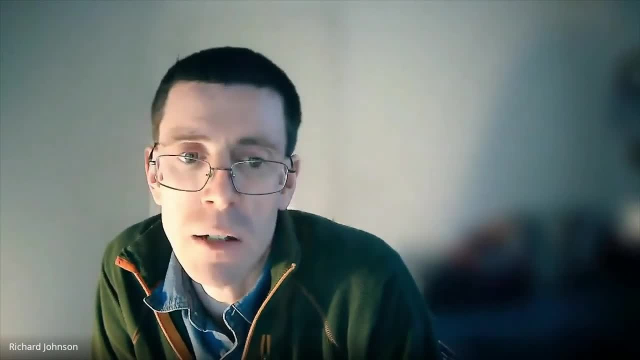 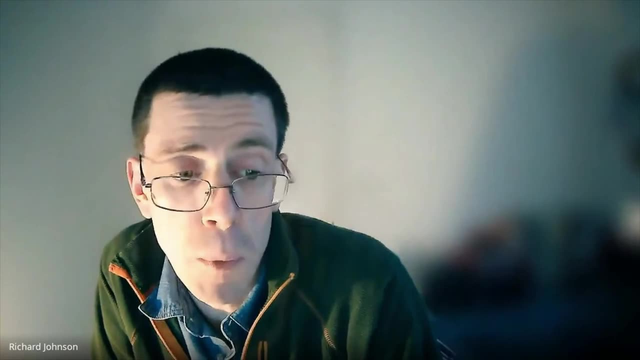 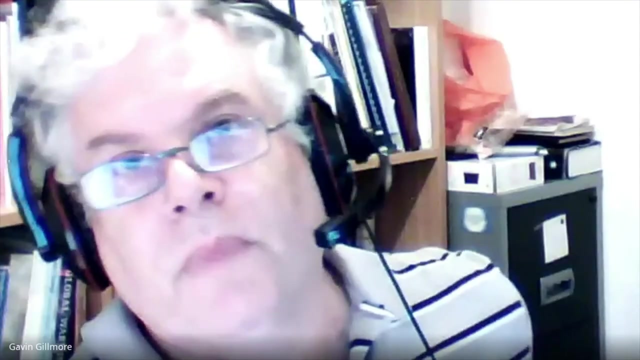 should it be mandatory for radon to be measured in advance of a house sale? And secondly, should there be mechanisms for new build, where all new builds should by law have mitigation, irrespective of where they are? It's interesting because different countries have taken different approaches. 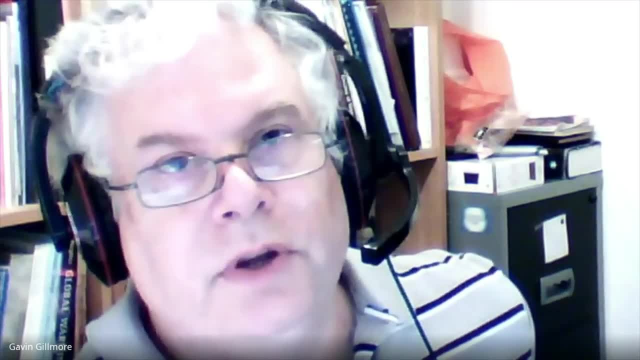 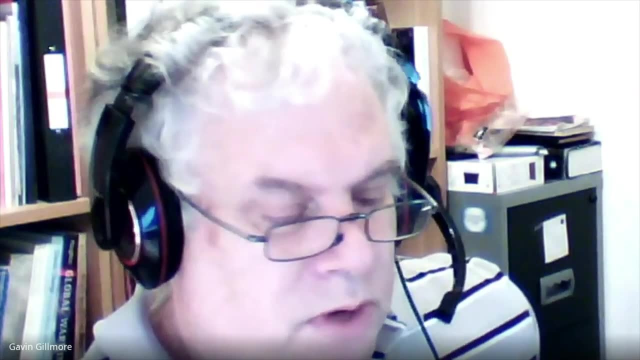 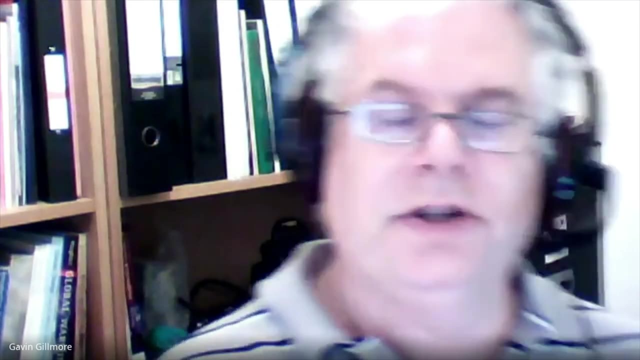 So Ireland, for example, say that if you're going to build a new property you must put in basic radon protection measures. So that might be a radon proof membrane instead of a normal damp proof course and a sump, but they may not activate the sump, but the sump is built. 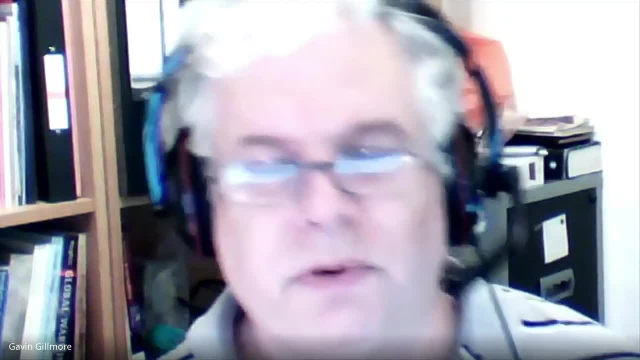 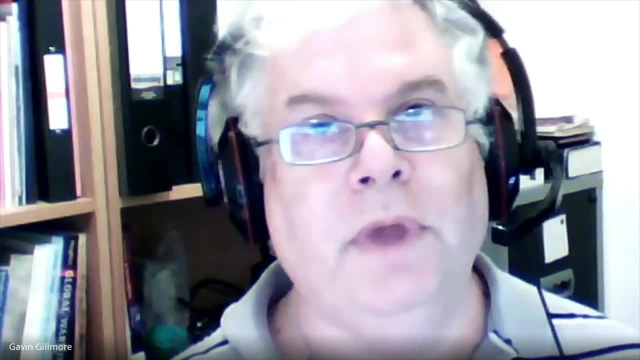 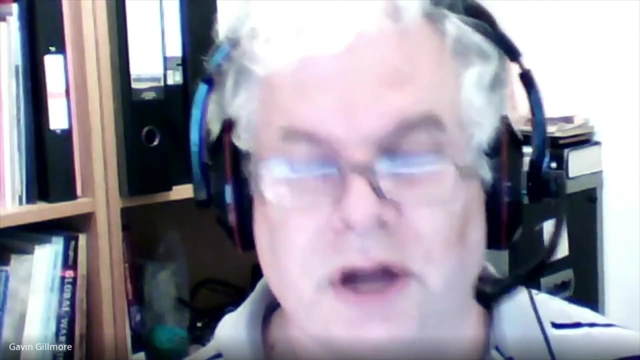 in. So basically they say: you know radon is a problem virtually everywhere. just build it. it's part of your costs. That's a very sensible way forward In the USA. most states in the USA say you must do a radon test. prior to your sale. In the States they do sort of one week radon tests. The UK tends to say, well, one week is not enough. Therefore we need to do monthly tests. people don't want to wait a month. 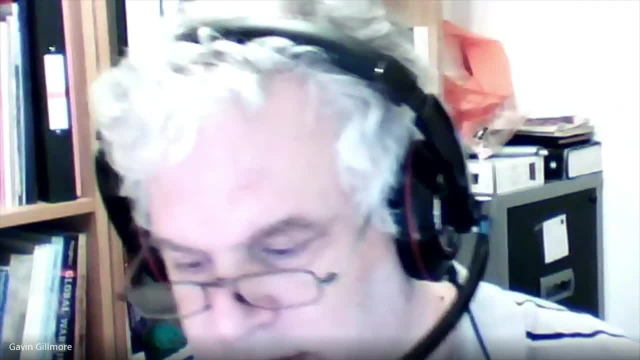 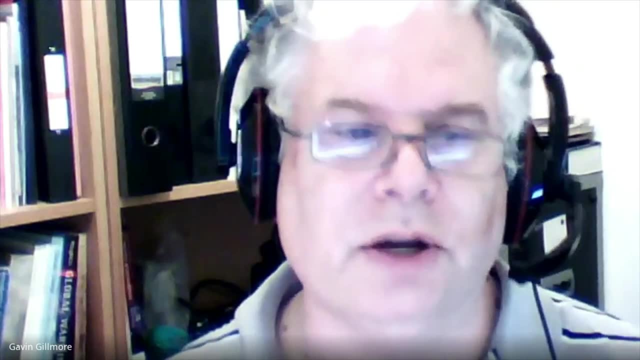 So they don't have this pressing need, as it were- if that's the right way of putting it- to do short-term radon tests. They don't think they give you accurate results, So different countries have different ways of doing it. I think the simplest thing is just to say: 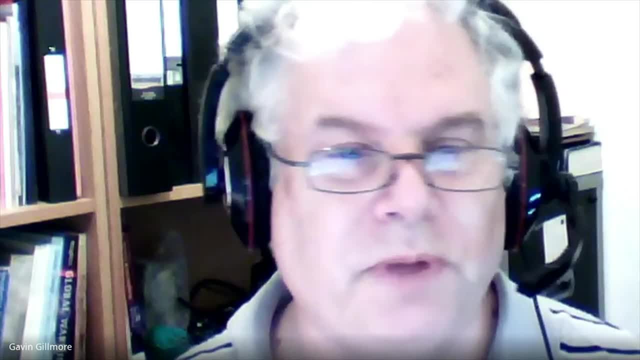 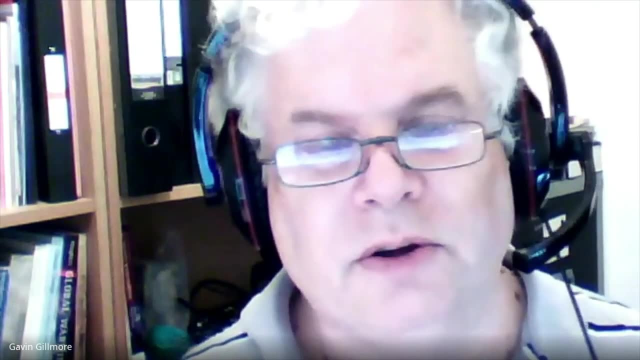 put in a radon barrier, put in a sump. it's part of the build costs, But the UK is so far behind building the number of houses it needs. the UK government doesn't want to impose that on the building sector because it's an additional cost. They did try and make the whole of the UK. this is Public Health. England propose making the whole of the UK a radon affected area, in which case everybody would have to apply the same rules and put down radon proof membranes, for example, But that didn't go. 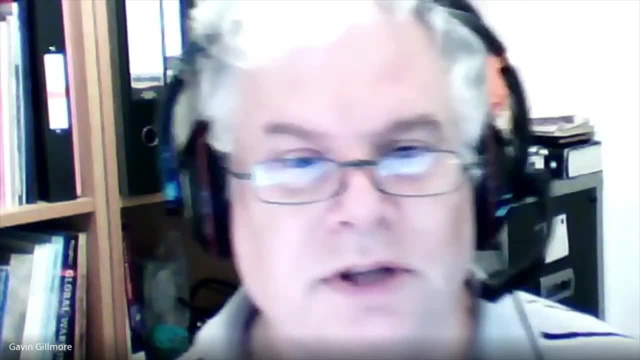 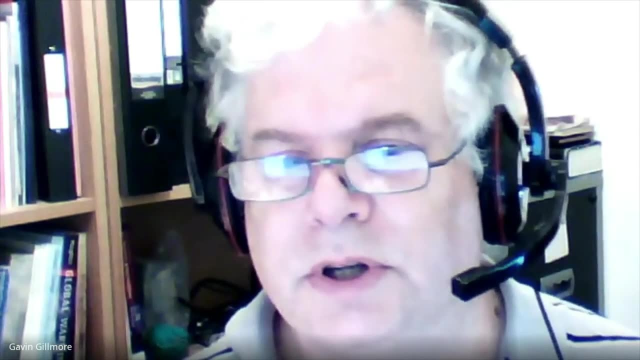 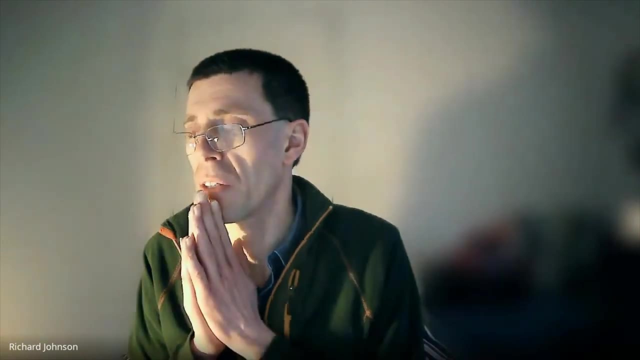 down very well politically because it was seen to be an expense for the building trade And, as I said before, that wasn't a rather sensitive thing to do really. Thank you, Gavin. Fascinating, Definitely, a debate there between health and politics. 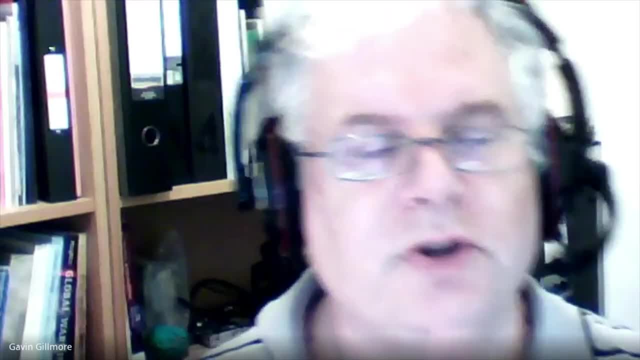 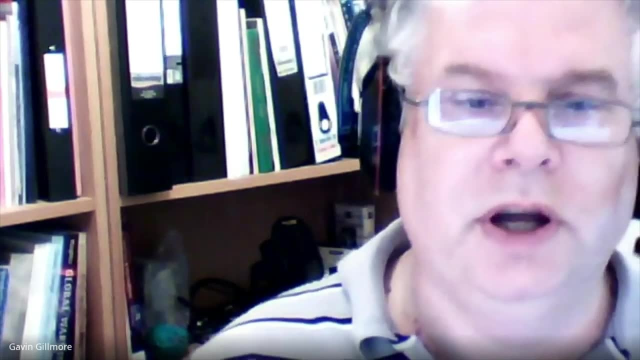 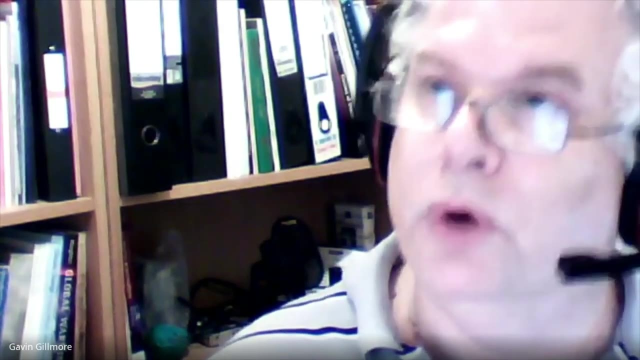 but we shall avoid that for now. I'm sorry There's a part of your question I didn't answer was the action level. in the UK is 200 becquerels in the home. There is no framework to force people to do that. There's no framework to force people to do that. There's no. 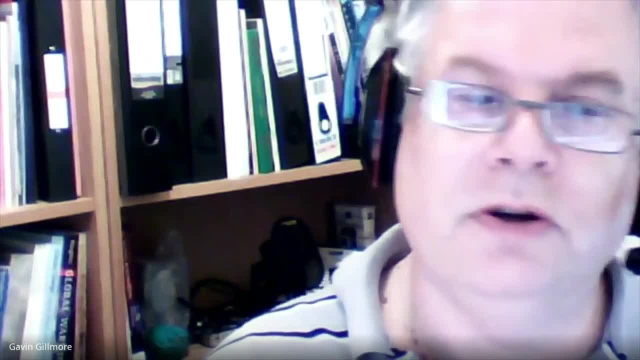 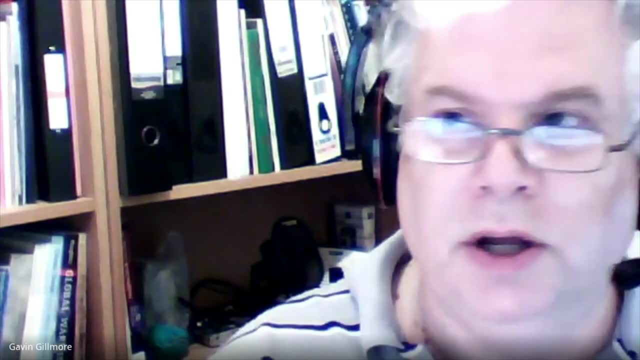 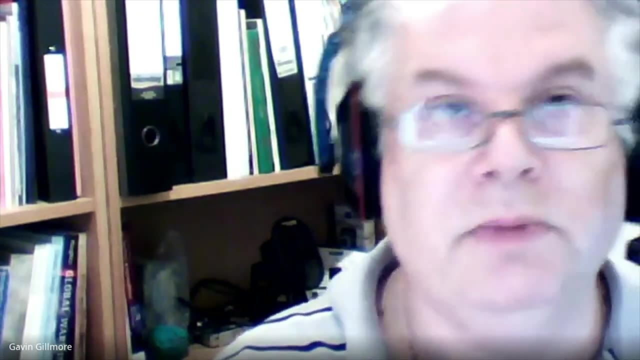 framework to force people to actually undertake either testing or remediation. There's recommendations by Public Health England and by the government, but there's no law which will force you to do that. But if you're in the workplace, the limit then is 400 becquerels. 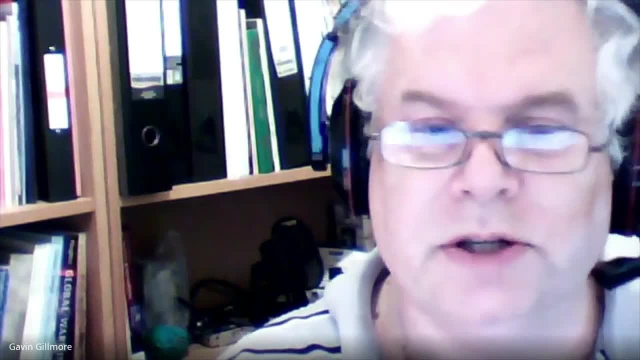 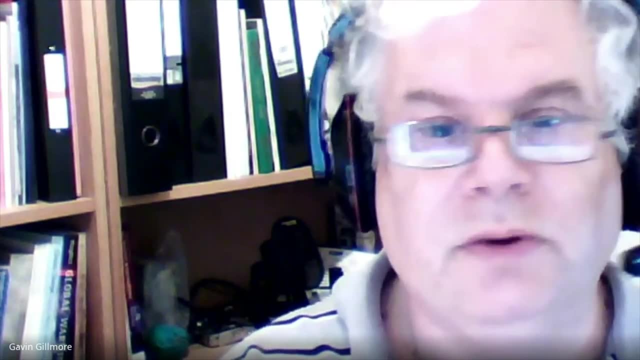 the logic being that you spend less time in a workplace, although they just dropped that actually to 300 becquerels. Then the health and safety executives say: you've got to do this, You've got to do this. You must take a test in your affected area And if it's positive, in terms of 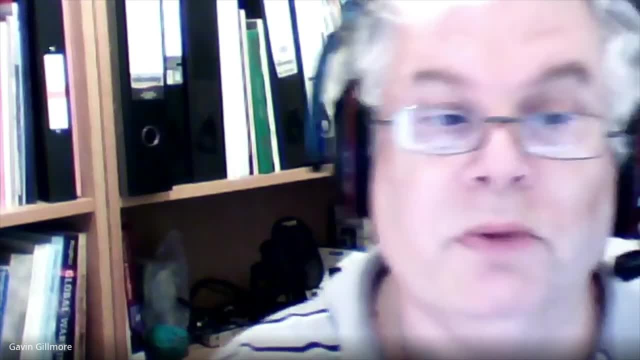 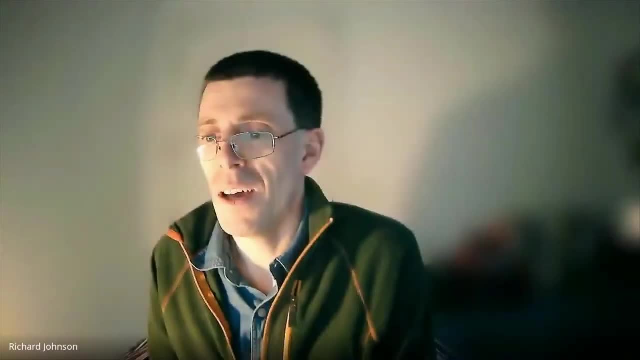 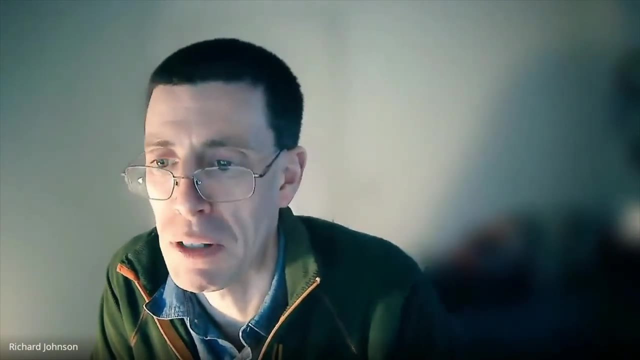 it's an issue, you must do something about it. That might not be remediation, That might be just working less in certain buildings. Thank you, Perhaps I can open questions to the floor. So if anybody else has a question, now's your opportunity to address that to Gavin. 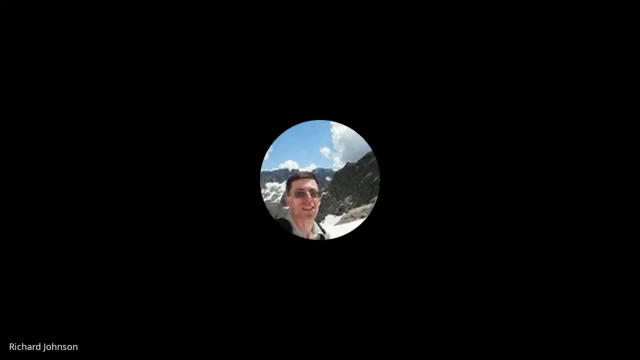 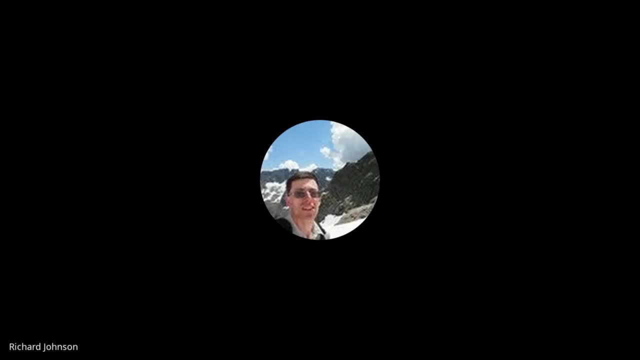 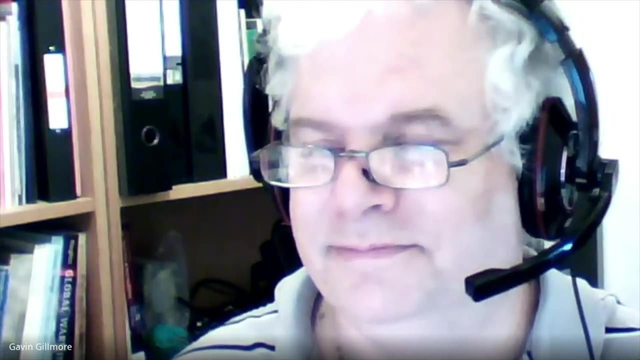 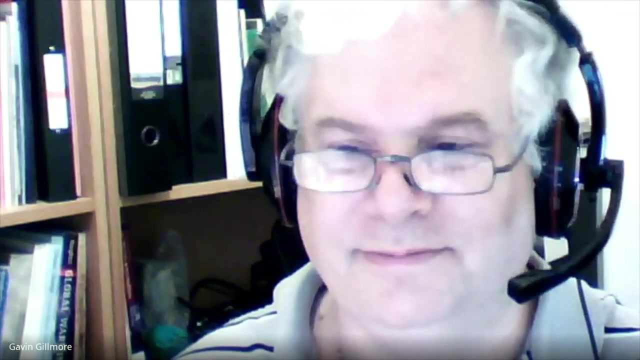 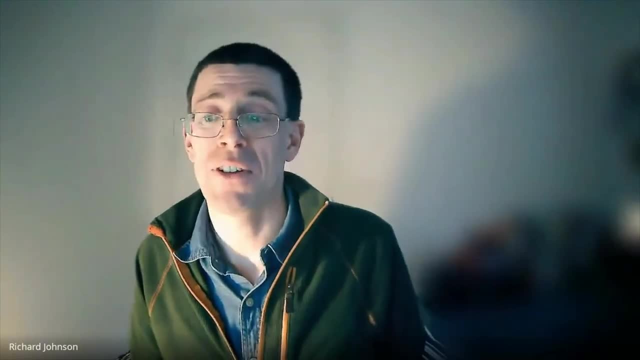 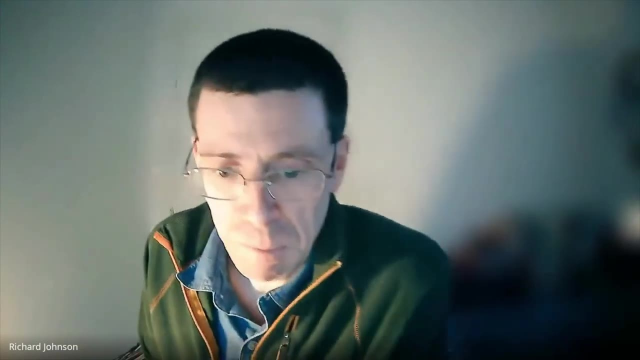 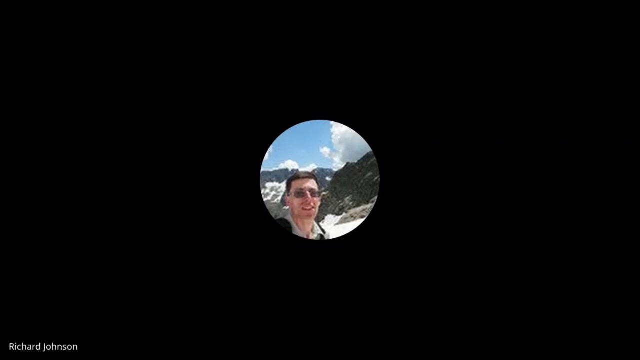 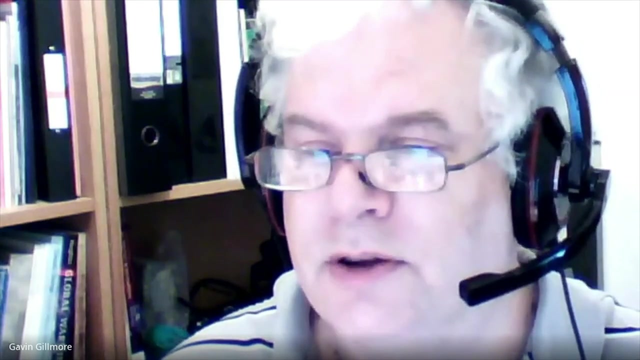 Thank you. It doesn't appear we have any further questions, but we may have the question from a question from peter. peter, do you want to try typing it in? ah well, i'll just say peter um works with the radon council, so um, uh, it's very nice to have. 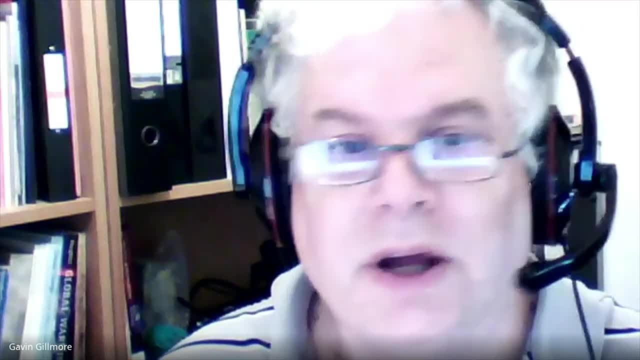 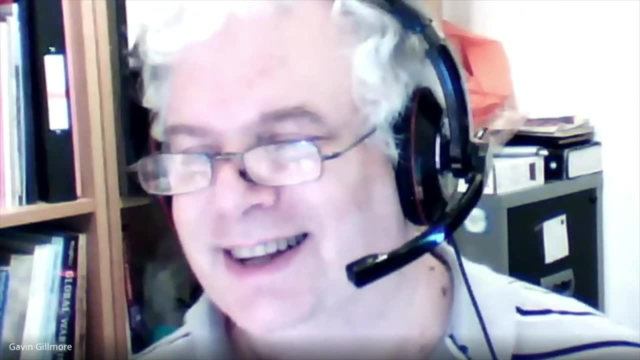 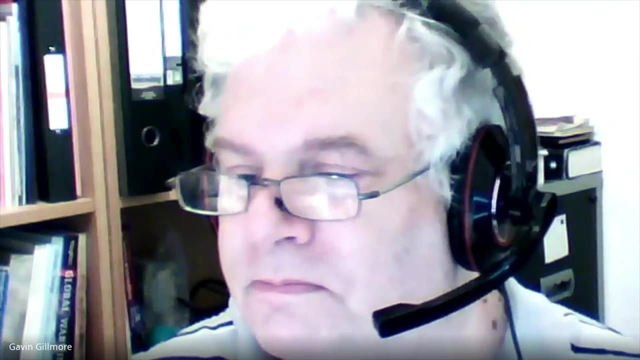 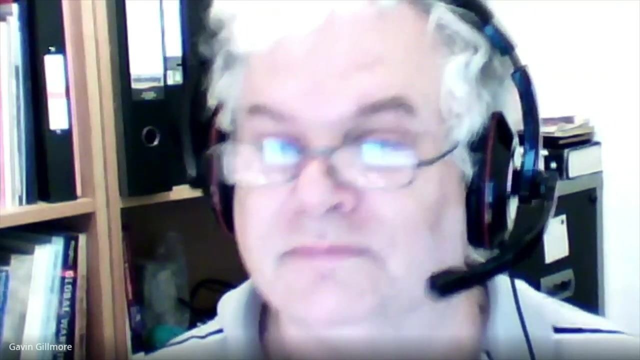 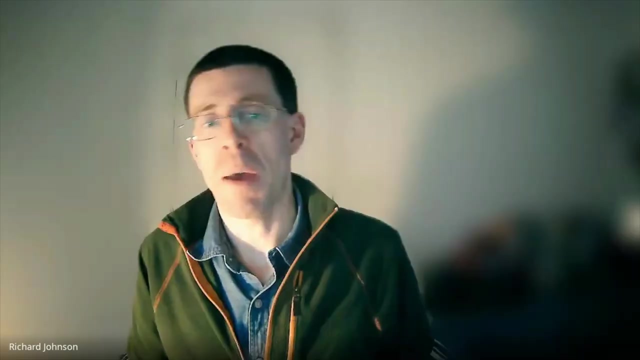 somebody from the random council here. um and uh, he knows an awful lot about radon. um, i'm intrigued to know what your question is, peter. i think we've got a problem getting the question through here. rich, it appears so. um well, i'm sure, if anybody else has any further thoughts or questions, that gavin will be more than happy. 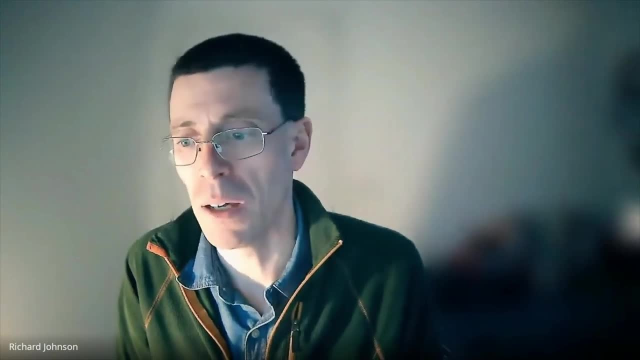 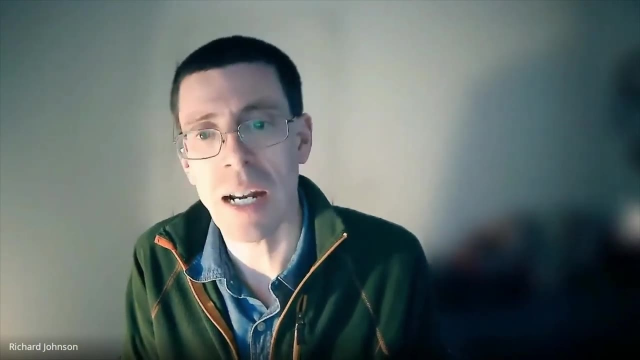 to address those and, of course, he's contactable by email, but i obviously want to thank you for your efforts and your insight this afternoon. gavin, i found that quite fascinating and i can clearly see, as my questions suggested, that those environmental links and cascades and 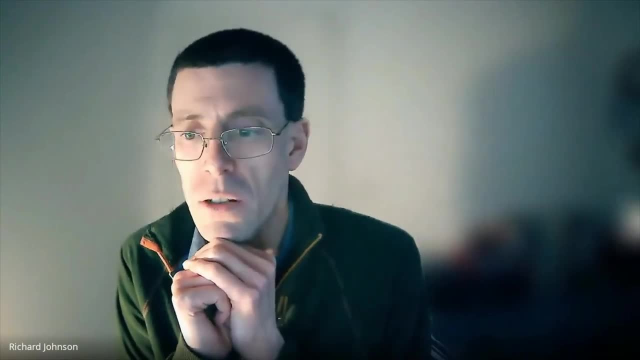 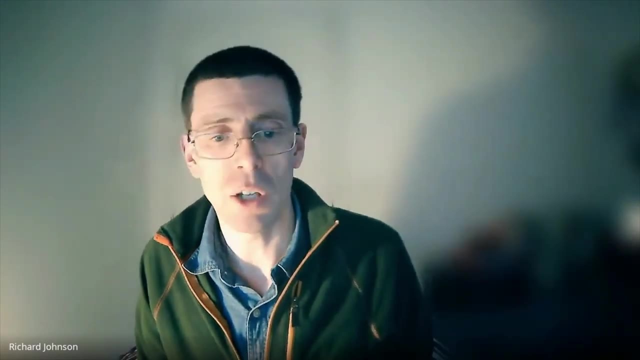 that's where i start to get quite interested in those process connections and, of course, that's how this is is generated and how we manage it. so thank you. i'm now going to hand over to jim, who's going to say a little bit more about what comes next. so over to you, jim. 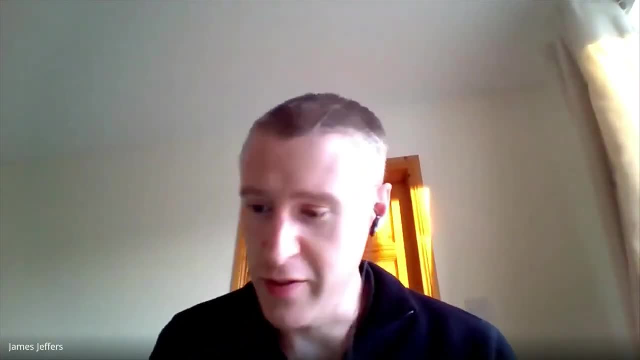 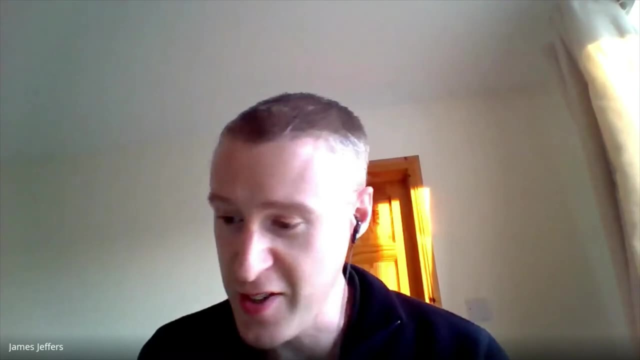 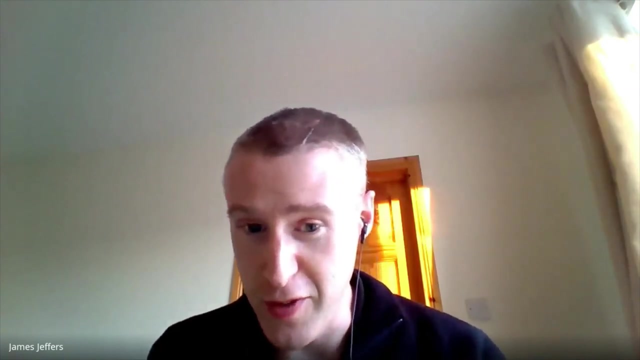 thanks, rich, and i would just add my words of thanks to gavin for a very interesting talk. and today's session wraps up our semester, one portion of our our lecture series. but in just a few weeks time we'll be um kicking off our semester two series and i just want to tell everybody that we have another. 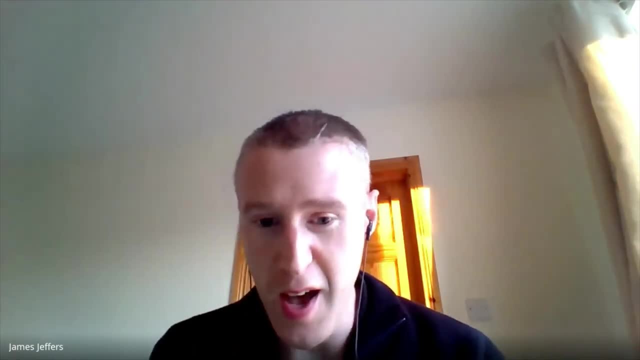 um seven events coming up in semester two and we'll hopefully have all of the details on those up on the the website, hopefully next week. but we'll be kicking off on wednesday, the 17th of february, with um professor james k mitchell and professor emeritus in the department of